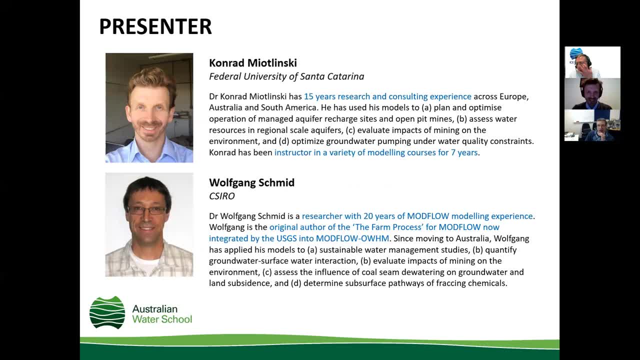 Where are you from, Konrad, this morning, this evening, this afternoon? Hi Trevor, I'm originally from Poland, but I'm currently based in Brazil. I used to live in Australia, too, for well, basically six years in CSIRO. 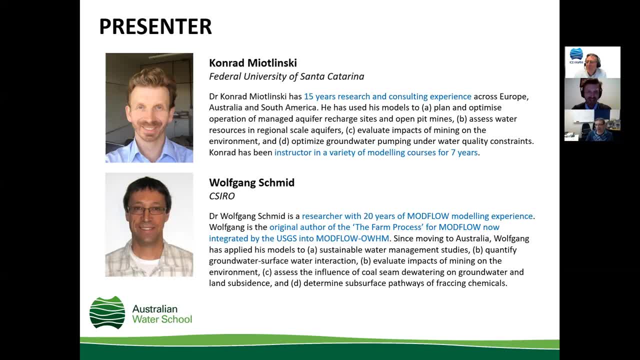 And apparently I live in Brazil, Yep, And burning the midnight oil, I understand. Well, it's actually not that bad. It's now, it's about nine and a half pm, so it's not very late. I could see that some participants from the middle part of that map you showed they must. 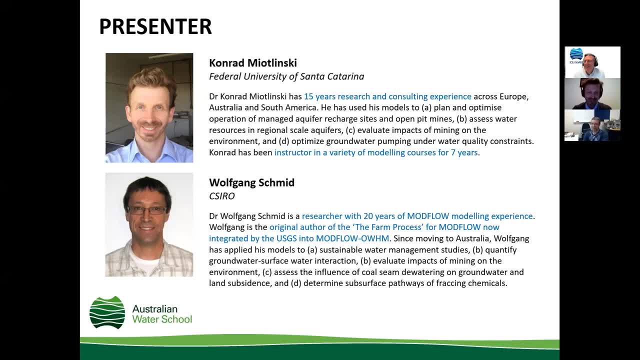 probably be in Madrid, Yeah, So it's probably a much more inconvenient situation than I am here, That's for sure, And probably that's the case for Wolfgang over there. You're in Western Australia, Wolfgang. your mic, your microphone, is not on, Meredith, yeah. 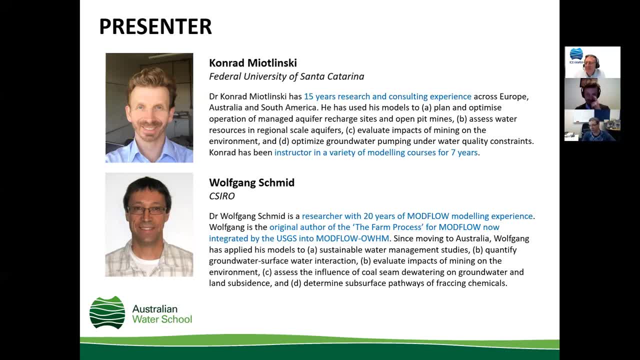 Yeah, I'm in Western Australia and obviously with a name like this, it can only be a German name. so I'm originally from. but I have come across the world, in many parts of where we have participants from, so I've been in the Middle East. so to you and then: 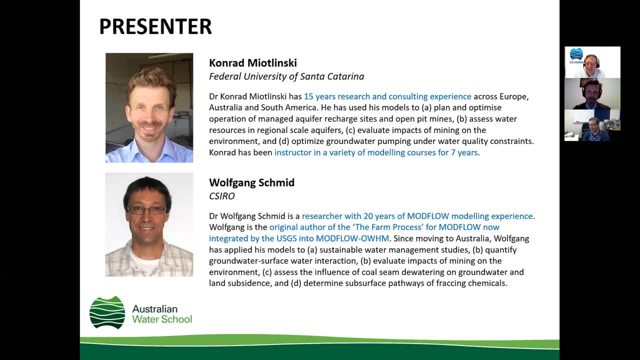 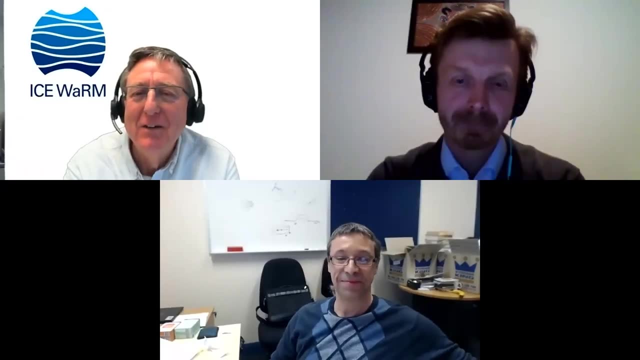 you know, In the United States, although there, and obviously in Europe for sure, and my wife is Filipino, so whoever is from over there, Well done. Yes, no, that's fantastic. It's great to have presenters who understand the breadth of our attendees at the webinar. 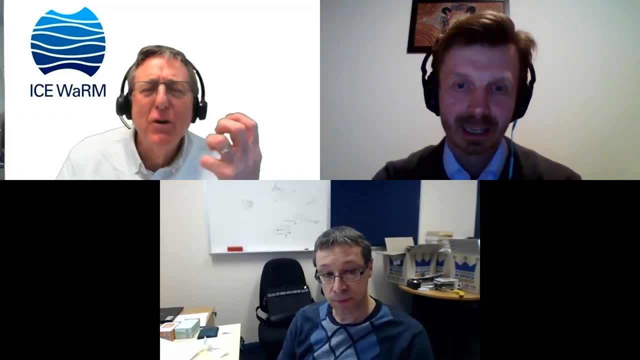 today? Where are you presenting? So what is your motivation, you know, and driver Conrad, for doing this work? Well, probably the most important thing, I think, is that you know we have a lot of participants. 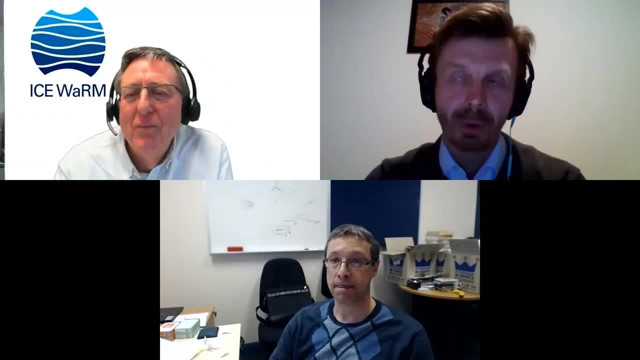 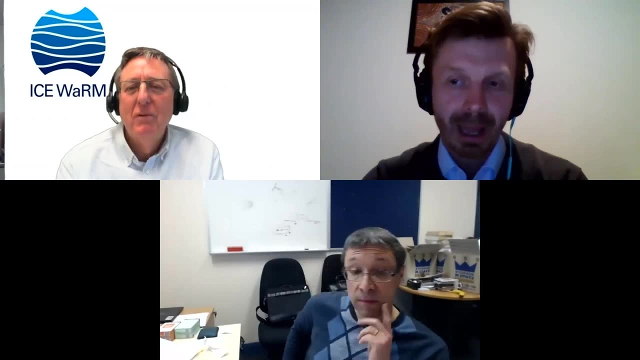 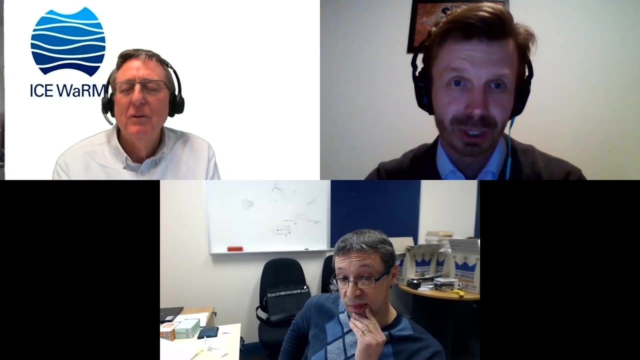 I think there are a few elements here, but I think that the most important Trevor is that we want to see our models to be more impactful and in order to achieve this, we need to firstly, support professionals to make sure that the models are good enough. 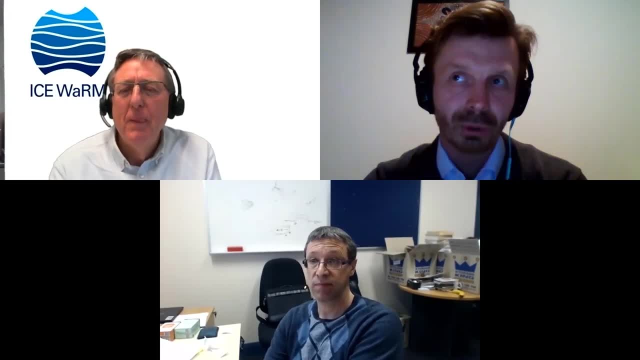 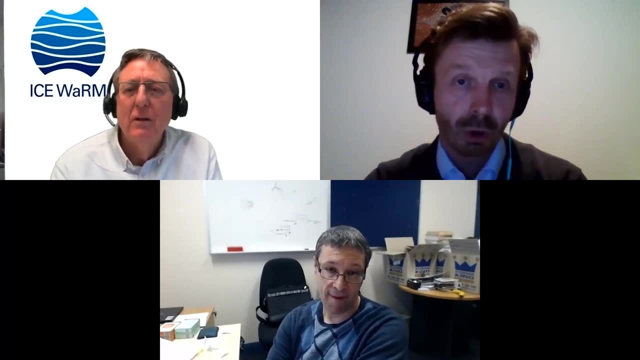 and secondly, we also need to convey our messages to our message to decision makers, to make sure that they feel comfortable to adapt the decisions that are coming from modeling. Yeah, So this would be basically the most important thing. 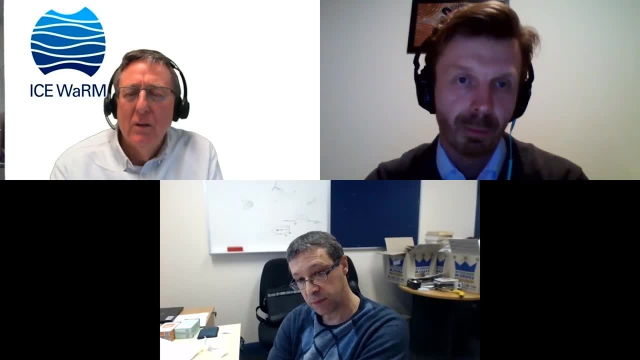 Probably there are a few others, but this is the most important motivation to give this kind of webinar. but it's excellent to be with you guys here. also, This is my first webinar. This is the first webinar I'm giving, so it's an excellent experience and I'm really 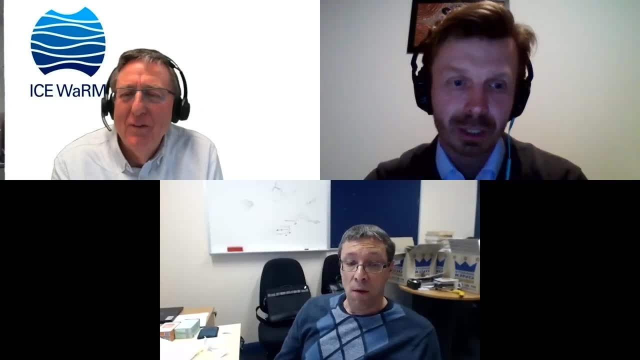 happy with the crowd that is spread around the world. There is probably more than 100 participants, and that's great. It's my great pleasure to be here. Yep, yep, You've certainly gone beyond that now, but thank you for that. 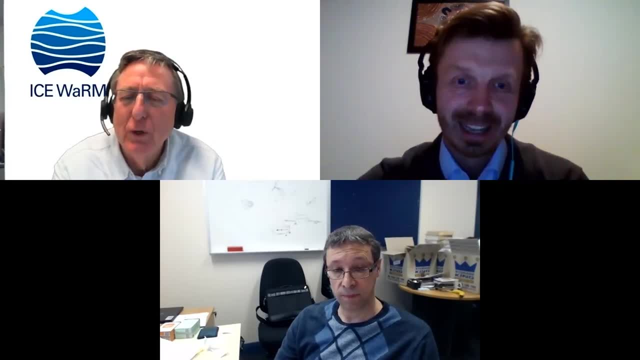 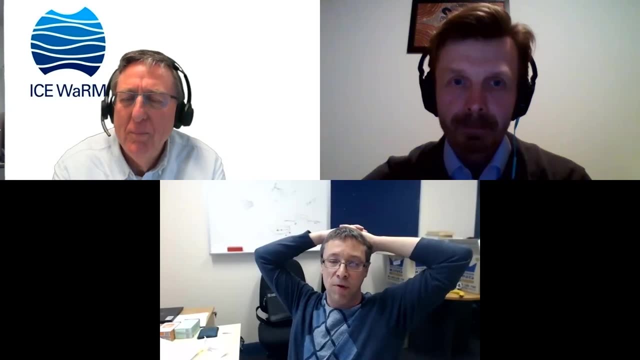 Yes, and yourself, Wolfgang. what motivates you into this sort of work? Well, I've been in this kind of business for a long time, probably 20-plus years- and for a long time, A long time, Matflow was just Matflow. 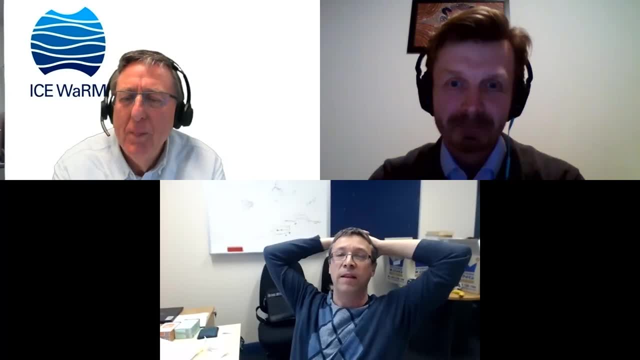 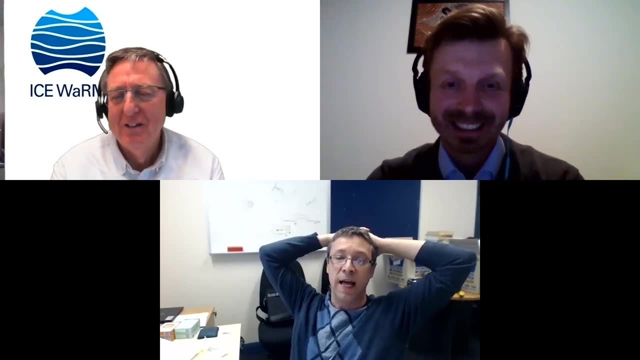 So my motivation is really to educate the public a little bit about the fact that Matflow is really not Matflow anymore. No, Matflow is at a crossroads and we are basically branching out in this class into different types of Matflows: one in the direction of more integrated hyperlogic models and 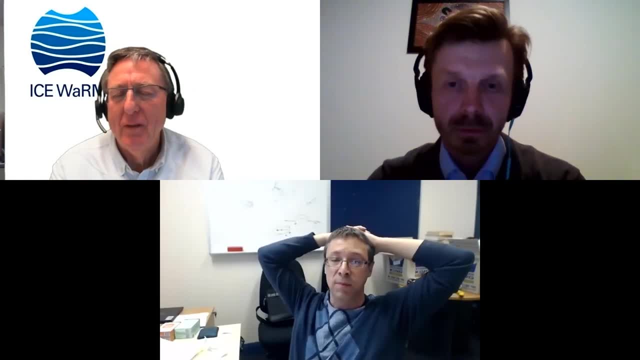 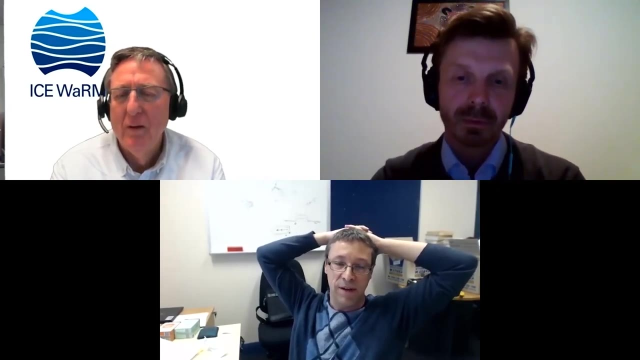 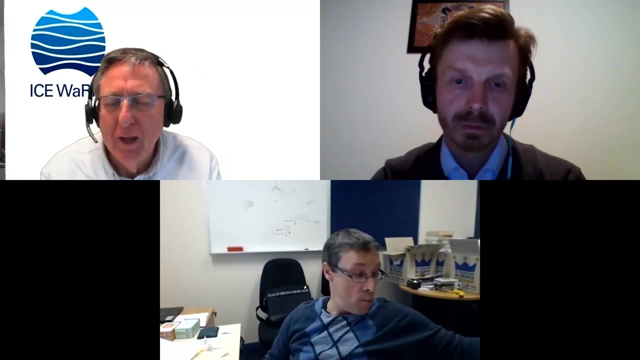 the other one in the area of having multiple models presented in one simulation or more heterogeneous aquifer conditions. All of those things have huge impact for management and management in the times of global climate change. Fantastic, That brings a huge amount of experience to it and you've put your finger on an emerging issue. 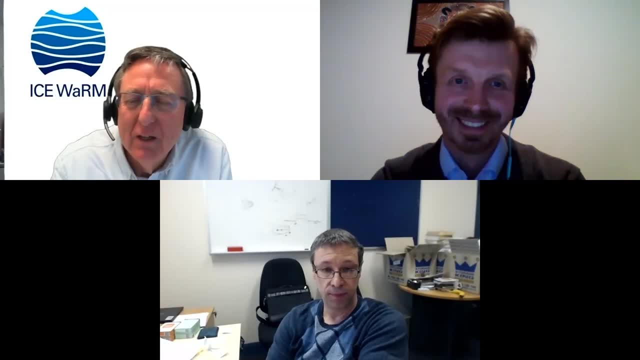 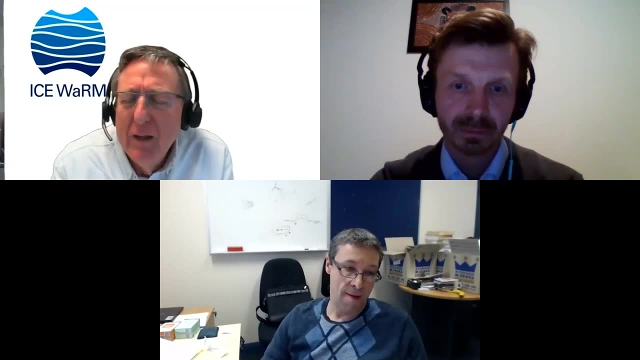 Matflow is no longer Matflow. Fantastic, beginning this, I haven't done a formal introduction. Can I just do that for a minute, Christy, if you want to put that screen back up again? I just wanted to see the background for both yourselves from different parts of the modeling experience. 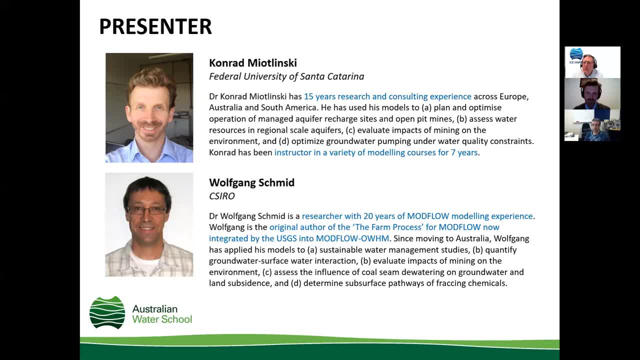 So Conroy has 15 years research and consulting experience across Europe, Australia and South America and has been an instructor in a variety of modeling courses for seven years. And Wolfgang, with CSIRO, is a researcher with 20 years Matflow experience and original author of. 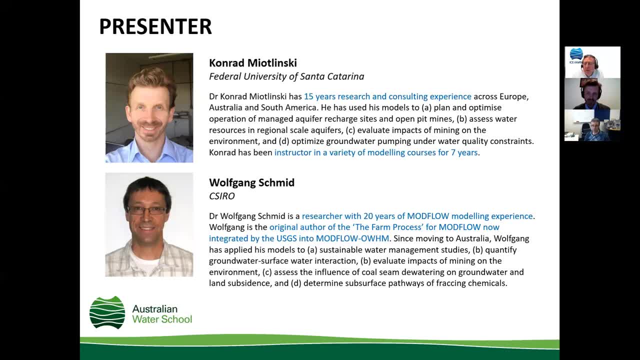 The Farm Process for Matflow, Now integrated into the US Geological Society's Matflow OWHM. So there's a large amount of experience being brought to bear in this webinar today, And I just wanted to highlight that you'll be hearing from the best of the best. 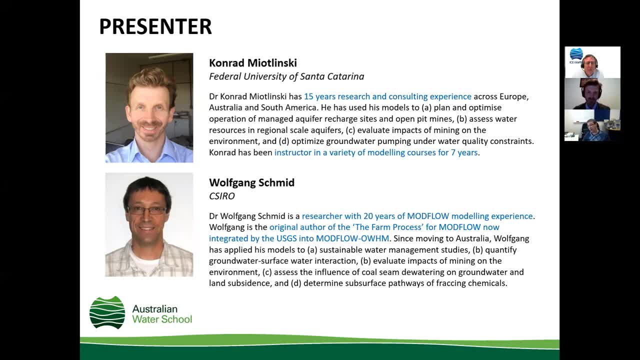 and we just encourage you to get your questions and discussion issues up on the Q&A board or come on screen. Both would be great, But by all means get them in early, get them in often and let's have a good discussion over this next webinar. 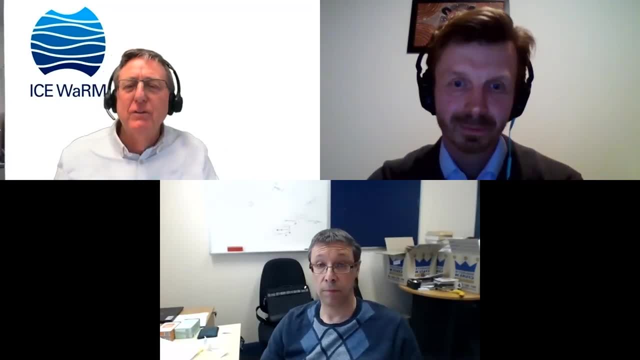 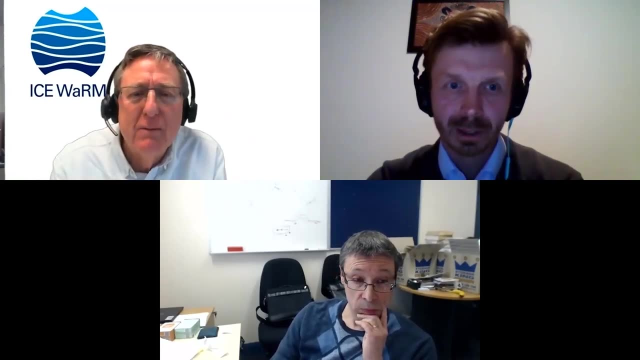 And I'll see you in the next 60 minutes, But for now I'm going to hand over to Conroy and you're just going to pass it between you and Wolfgang Conroy. I'll leave that to you, and any relevant questions that come up as we go through, I'll break in at the right moment. 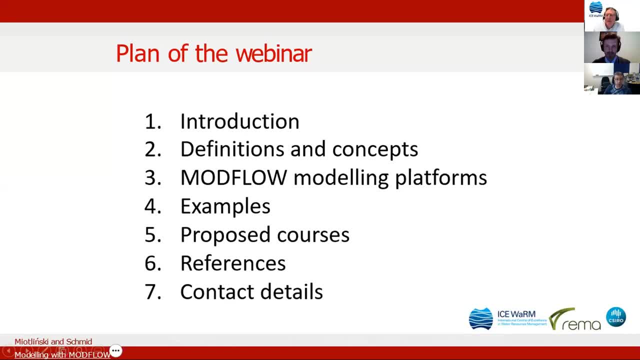 So over to you, Conroy. Thank you, Trevor. So we would like to start this webinar giving a little bit of introduction about what the model is, what we can expect, What we can expect from modeling, what we- why do we really bother about modeling? 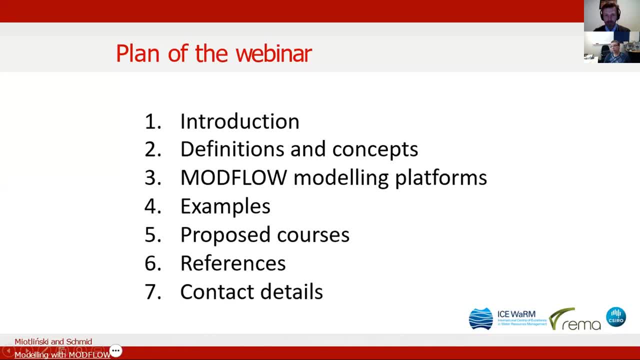 Then we would like to present you guys a little bit of, to show a little bit more about Modflow, how it does the computation, but without going too much into details. Then we would like to present to you two examples. We have some suggestions for the courses that we would like to share with you. 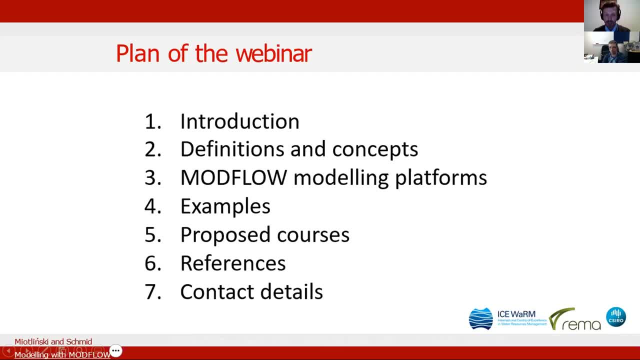 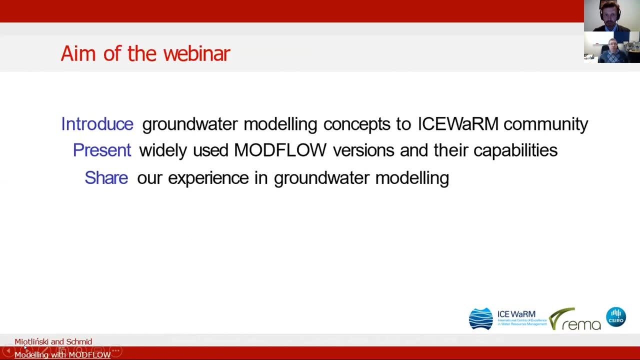 There are some interesting references and, finally, we will provide with our contact details. So, firstly, the aim of this webinar is basically to introduce groundwater modeling concepts to the ice worm community and to present widely used most flow versions and basically their capabilities. 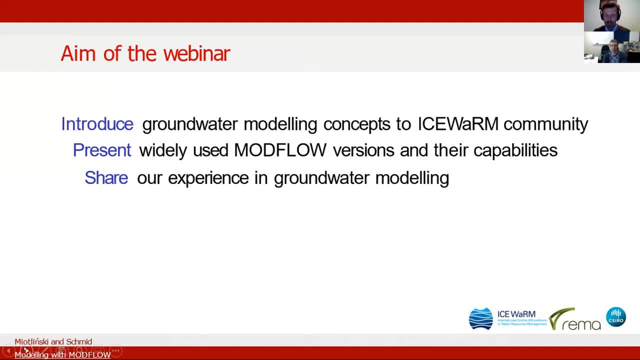 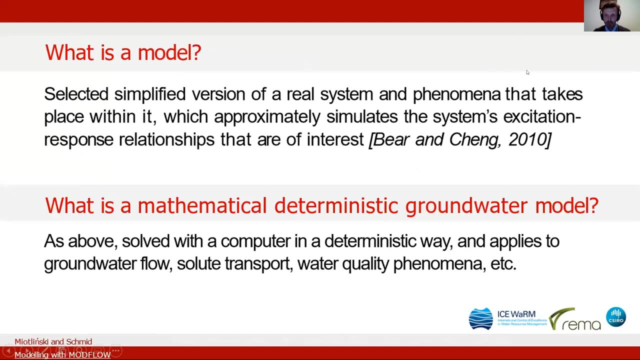 You will find that the capabilities differ quite significantly. And finally, we'll share our experience with modeling. So what is a model? It's basically a simplified version of a real system and phenomena that takes place within this, which approximately simulates the system's excitation response relationship, that are of interest. 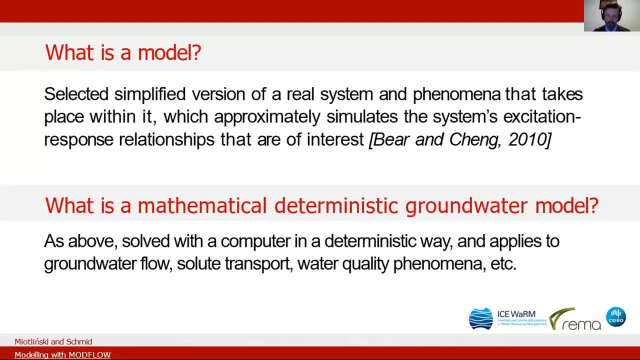 And this is very broad definition. When we talk about groundwater modeling, we normally think about mathematical model, But obviously there may be also analytical models, And this particular situation will be talking about deterministic groundwater models. So it means that we think about a model that is solved with a computer in a deterministic way. 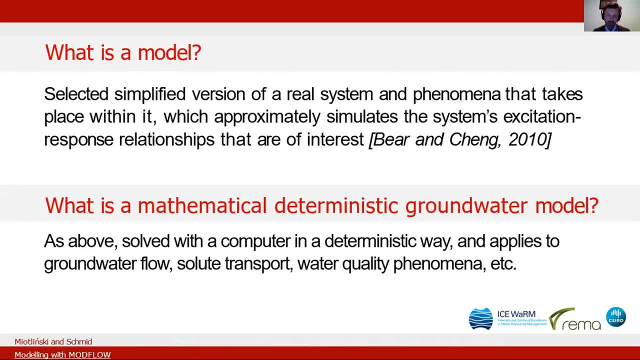 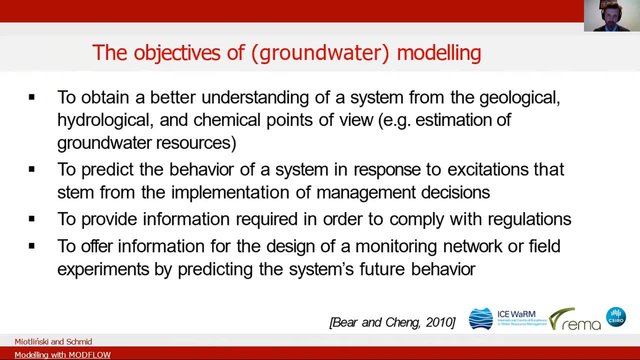 and it applies to groundwater flow, solar transport, water quality phenomena, etc. So it applies to the groundwater, to a specific groundwater problem, And the objectives may be as follows: Firstly, to obtain a better understanding of a system from a geological, hydrological and chemical point of view. 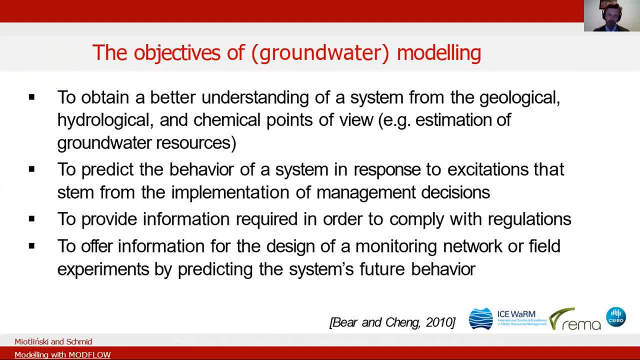 For example, we may want to estimate groundwater resources, or we may to understand spreading of contaminant, or we may study infiltration and processes of clogging during managed aquifer recharge. Secondly, we use models to predict the behavior of a system of groundwater system. 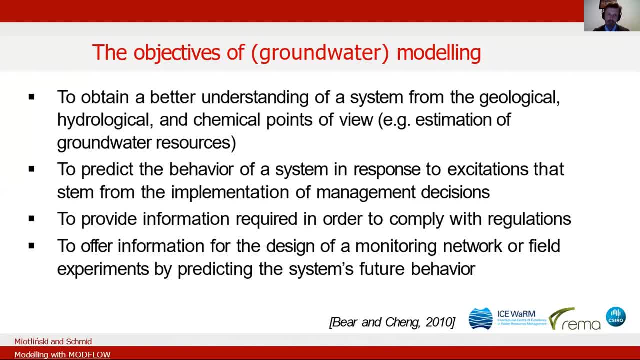 in response to excitations that stem from the implementation of management decisions. We use them to provide information required in order to comply with regulations And, finally, to get information for the design of a monitoring network or field experiments, by predicting systems' future behavior. 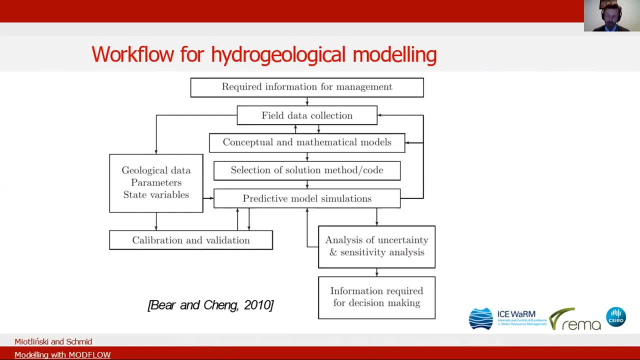 And there is a workflow for hydrogeological modeling. There is a number of steps involved. Everything basically comes from the top. that is what is really needed, What's the motivation of the modeling or what's the objective. And then there is obviously we need for modeling, any kind of modeling. 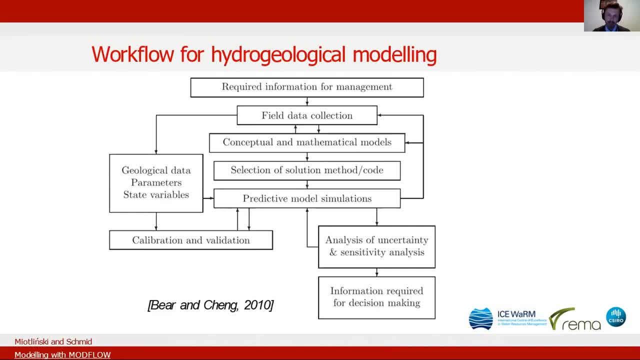 we need data, quality data, And then we develop a model. we start developing a model, Firstly starting with a conceptual model, which I explain a little bit what it is about, And then developing mathematical models. In this case it's very broad, actually workflow. 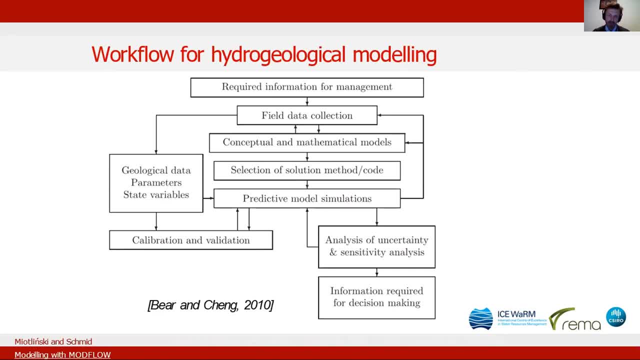 In this case it's saying that we develop mathematical models but obviously, if some codes are available for us, we don't. well, we have to develop them, but some of the elements that are shown in this particular workflow we basically don't do. 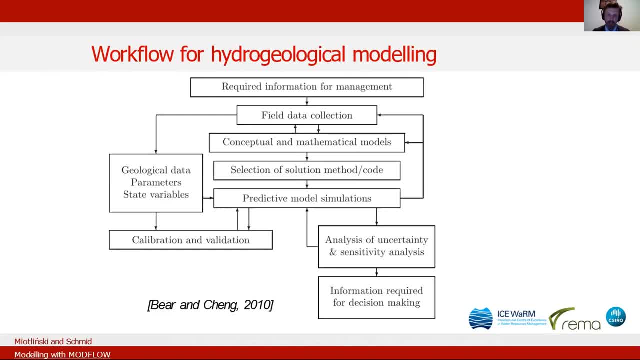 We use the ready solutions. This could be, for example, the next element, which is selection of a solution, method and code, And then we, as modelers, we run simulations To predict a certain scenario And there is a number of other elements involved, and you can see that there is some looping here. 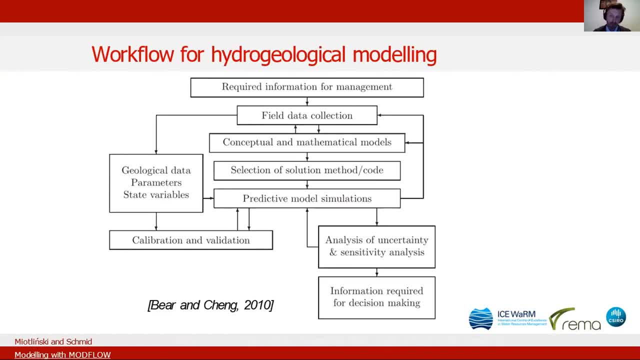 After predictive model simulations, we may need to probably calibrate and validate the model, but it's very likely that we may need some more data or we need to verify our conceptual model. Almost any time we need to do some kind of sensitivity analysis and analysis of uncertainty. 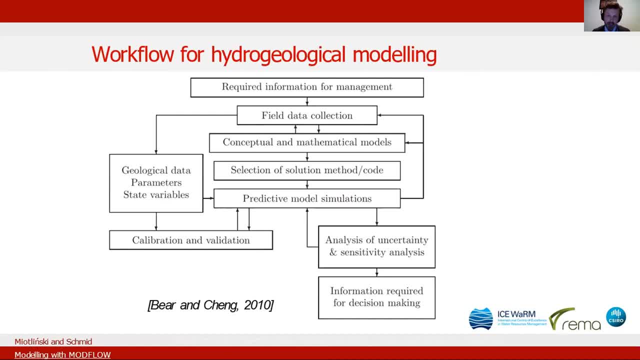 particularly when we talk about the predictions And then we finally give the answer. This webinar is basically focused on three steps, So we'll not be talking about quality of field data or how to perform uncertainty analysis, but what's conceptual model, why we select certain code. 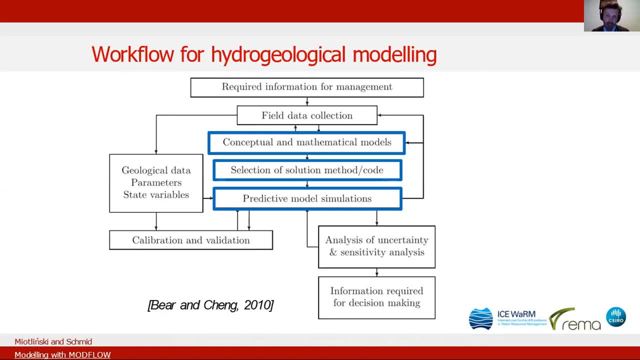 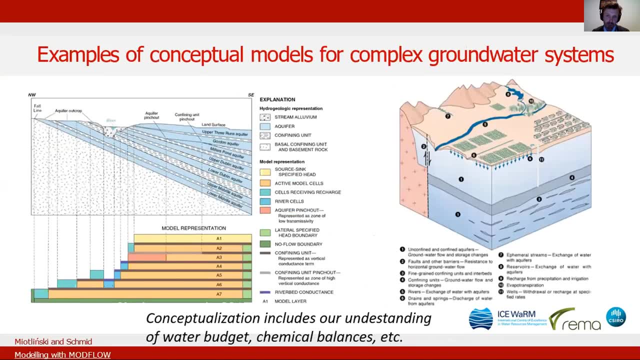 and what those codes offer. And when talking about examples, we may talk a little bit about predictive model simulations. So here in this quite complex slide, we have two examples of conceptual models. On the left-hand side we can see a model of multi-layered simulations. 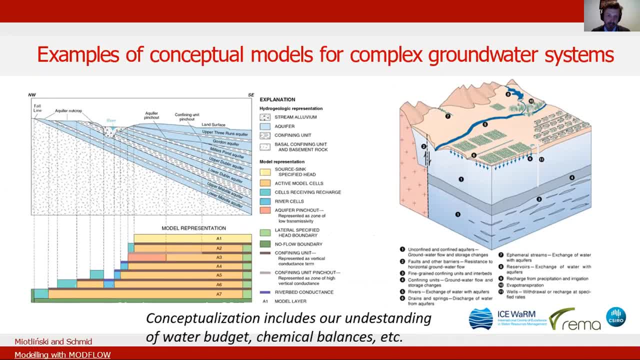 It's basically on the upper part. we have hydrogeological cross-section. So this is the cross-section we normally have to have in mind if we this kind of image we need to have in mind when we do modeling. So we have seven aquifers. 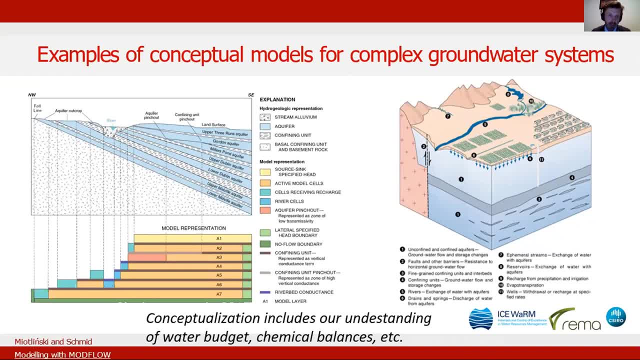 And they are. they have certain connections or they may not have any connections, But in the lower part of this plot we can see how these layers or how this hydrogeological information is represented in a conceptual way And how certain layers may be connected. 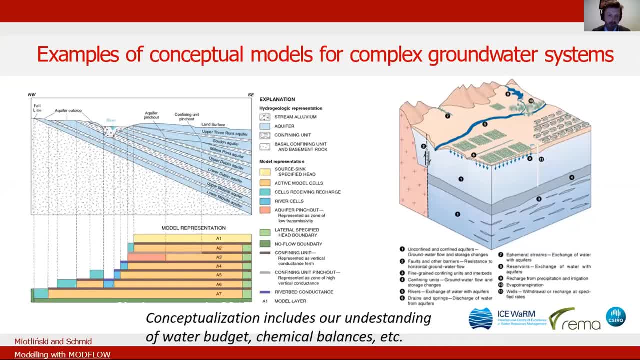 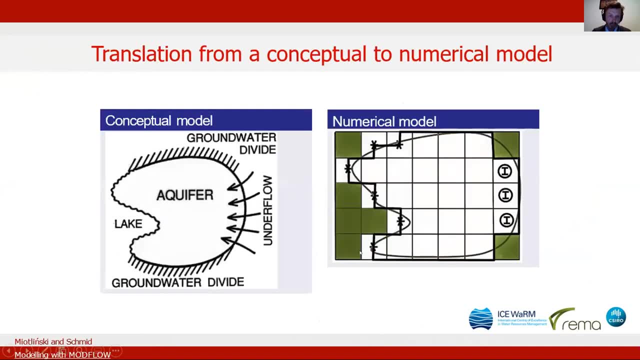 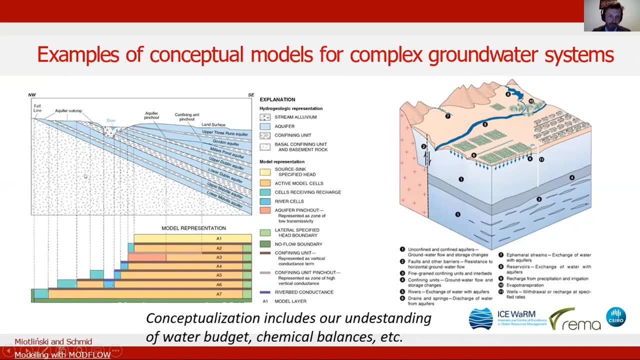 with respect to each other, but also with respect to the surrounding, Which, in this case, on the left-hand side, we can see, oops, we can see that there are some connections with a river system, or it can be connection with atmosphere. 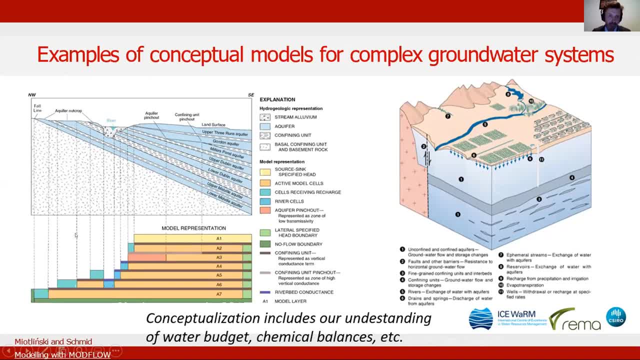 And so the aquifer is in this particular location. This aquifer is unconfined aquifer And may receive recharge from precipitation. And on the right-hand side, there is another way of representing conceptual model: It's a 3D diagram. 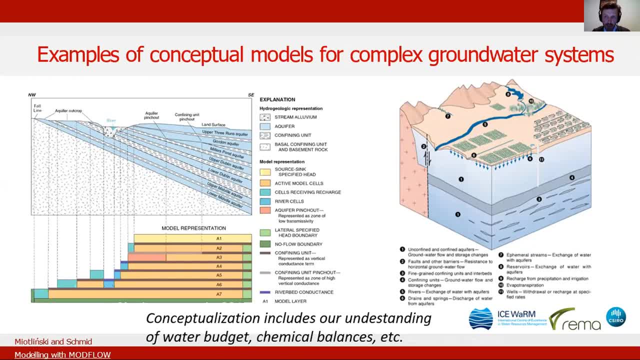 And a number of processes is shown here We have- we have basically two aquifer systems. The upper aquifer, unconfined aquifer, has strong interactions with surface water. It receives recharge, but it's also not only from precipitation. 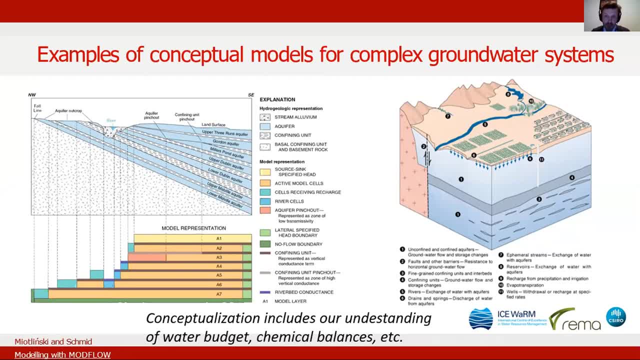 but also from irrigation It also it's drained. There is a river, There is a pumping well And you could also see that there are. there is some connection, probably not well. from this we can't really see much. 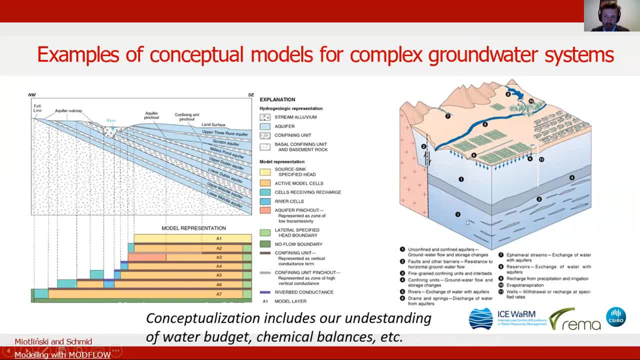 but there is some connection with the lower aquifer, which is confined aquifer, And then we may, we may, looking at this picture, we may always think where possible connections may be, or where percolation, where the percolation takes place. 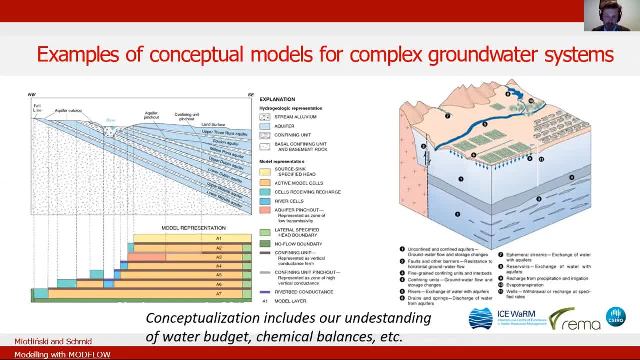 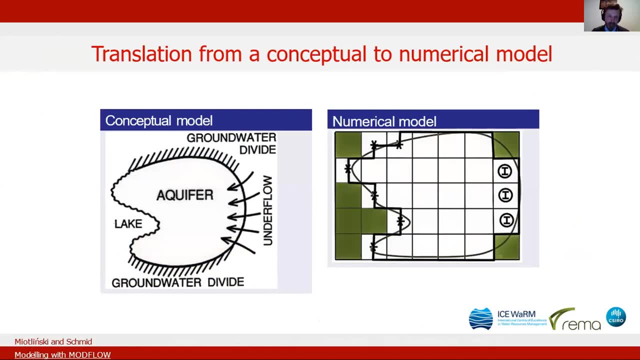 exchange between aquifers and so on and so on. So this is the conceptual model And this, basically this slide shows you how we translate the conceptual model into numerical model. So we have an image- We need to have an image- of the system we model. 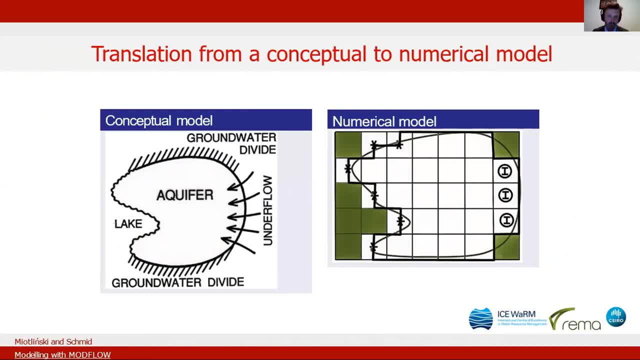 Obviously, this is very simple scenario: Two-dimensional aquifer, looking from a top plan view And on the right-hand side. this, this conceptual model, is already divided, or subdivided into smaller elements. We call them, we call it green, And then we have, we call it white. 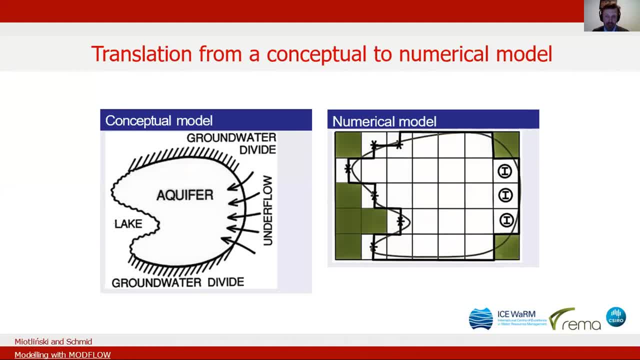 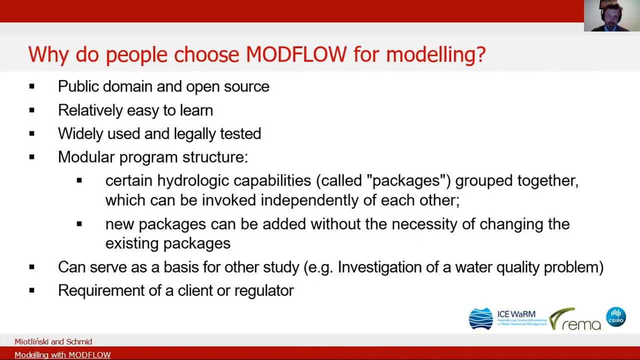 And for each element. each element has specific calculation that's taking place for each single element And they are connected with respect to each other. They may have a bit different function And I will also talk about this a little bit more- And so at this stage, when we talk about selection of the 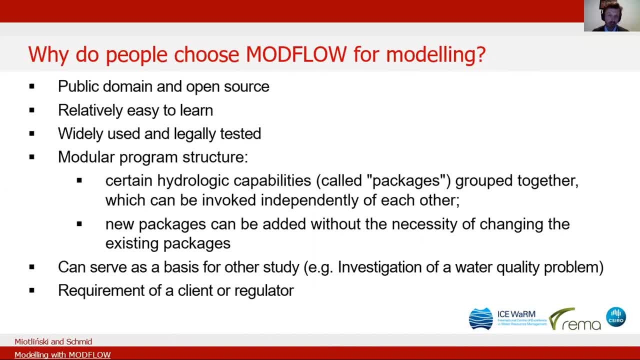 code or program. we would like to show you why people normally or would like to discuss with you how, why people normally choose Modflow for modeling, And I particularly started also with Modflow many years ago in Poland And I found it at this time- at that time, quite easy software to learn. 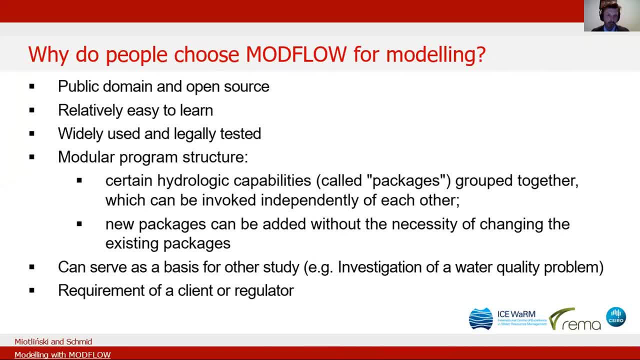 But there are also different motivations And they are as follows: This is a public domain and open source, So you can, using certain tools, you can basically run, use models, develop models for free. Obviously, there are some commercial, there is some commercial software. 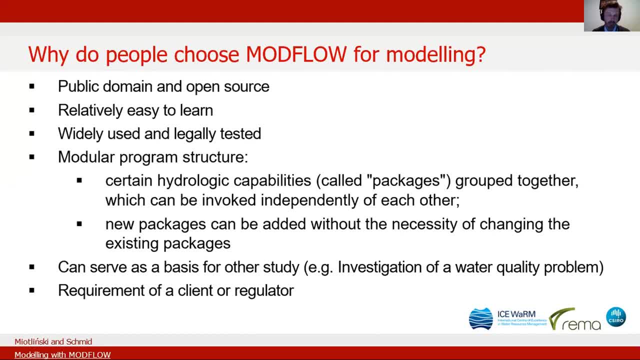 on the market available, which may help you to develop models, But it doesn't have to be, And Modflow is very widely used and it's legally tested. It has very convenient modular program structure, which means that certain hydrologic capabilities are grouped together and which may be invoked. 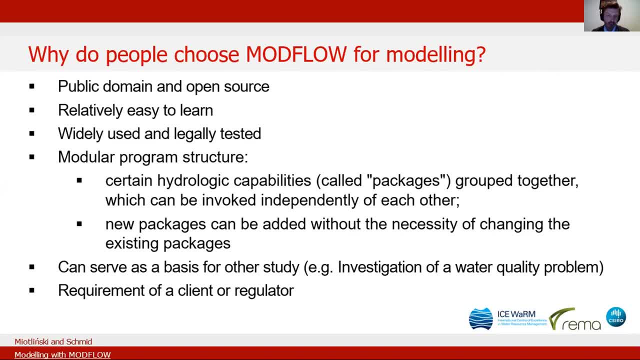 and they can be invoked independently or of each other. New packages can be also added without the necessity of change The existing packages. So this is something once you get, once you get familiar with this concept, then the workflow is quite easy. 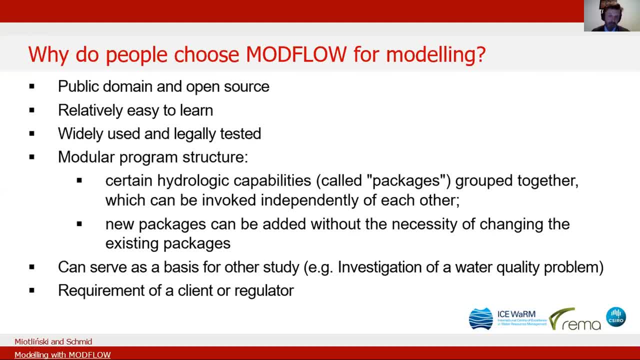 Modflow is also used because it also serves as a basis for other studies. For example, very well, together with Modflow, together with different software, it can be used to study contamination problems or water quality problems or density dependent flow and so forth. 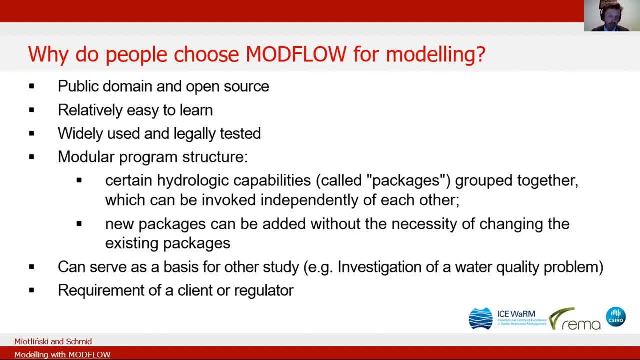 And sometimes it's also used because there is a requirement of a client or a regulator. Obviously well, personally, I'm not very much in favor of this kind of requirement, because I believe that a modeler should be capable of influencing what kind of choices are made. 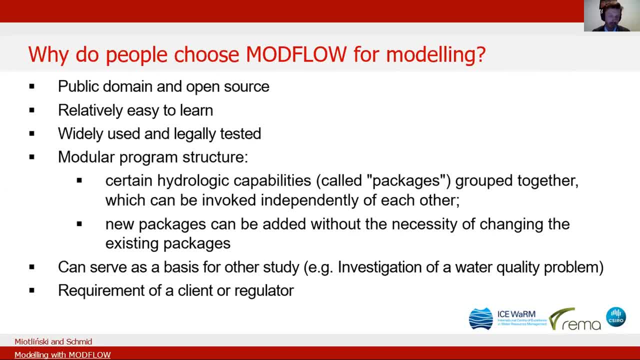 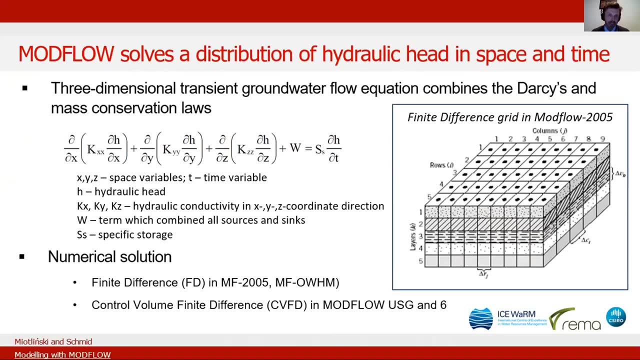 Modeling choices, including choices of the code, are made depending on the objective of the modeling, But in practice this is often also the case. So what Modflow does is basically it solves a distribution of hydraulic heads in space and time using a groundwater flow equation. 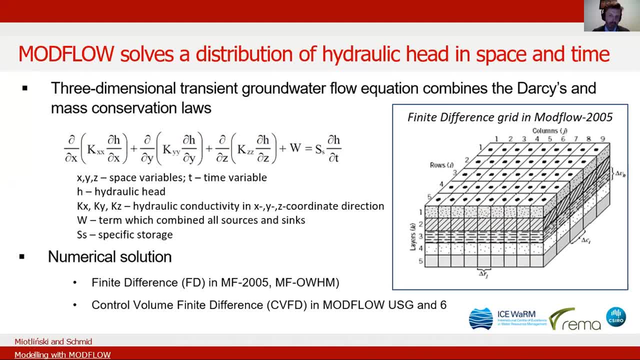 This groundwater flow equation that you see on the screen is basically combines Darcy's law and mass conservation law, And it's it's a three-dimensional equation. So we have three space variables: X, Y, Z. There is a time variable if we run models in transient mode. 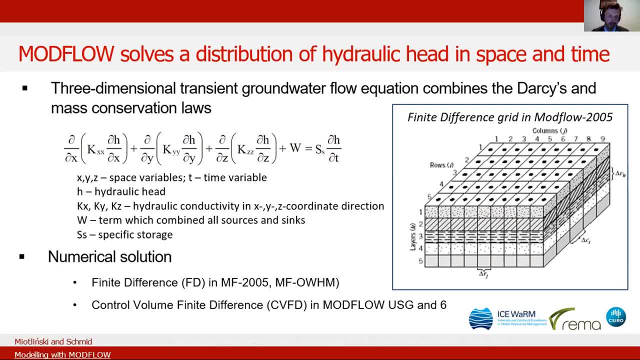 And there are certain parameters, basically hydraulic conductivity of the aquifer material, but also a specific storage, And we also have a very important term that is shown here as W, And this term combines all sources and sinks. So this is a very important term in the model, because this model is not isolated. 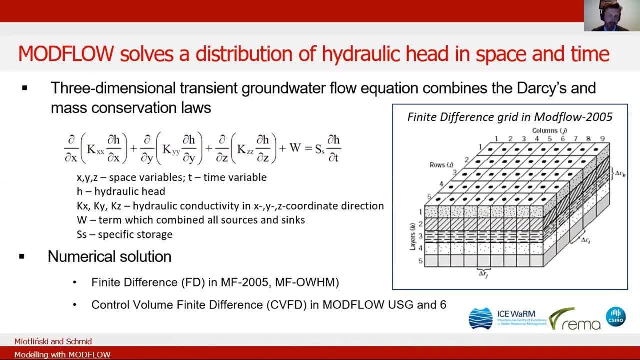 It's. there is always some kind of- almost always some kind of isolation. There are very few, very few groundwater systems in the world we know that are that would be completely isolated from the surrounding, So this term is is responsible for this. 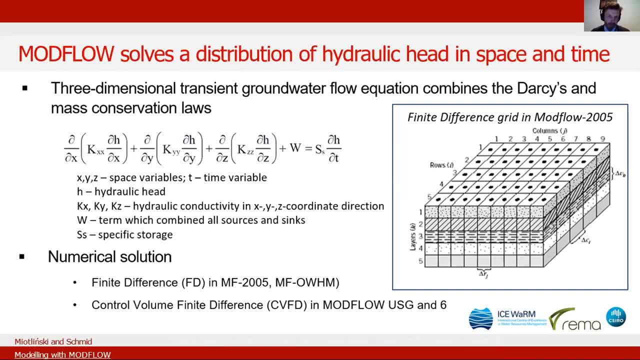 And then there are many ways of solving numerical this equation. basically- And in ModFlow it's basically it's either finite difference solution or control volume finite difference solution. that started back in 2013 with ModFlow USG And it continues now with ModFlow 6.. 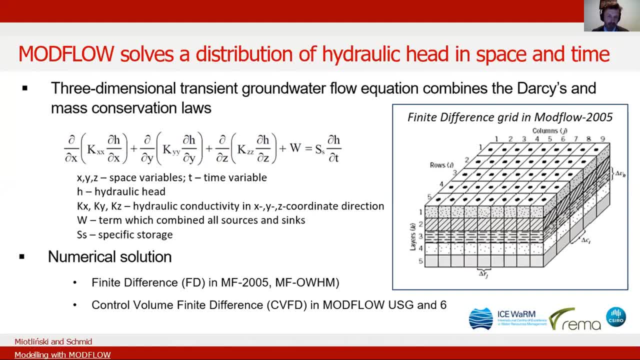 On the right-hand side you have a picture that is showing finite difference scheme used in ModFlow 2005.. It's, as you can see, it's very regular, very regular grid, And so for every single element of this or cell, we call it cell. 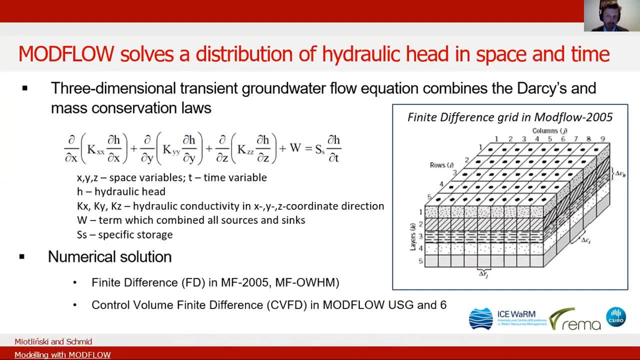 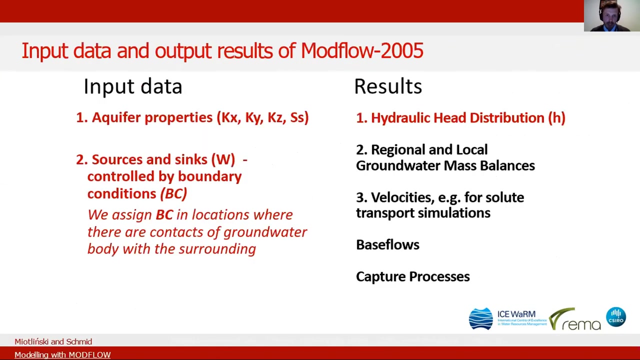 And we calculate, We may get, we can calculate hydraulic, hydraulic head. And you can also see that every single element is surrounded by minimum three other elements, or maximum six, six elements If they are, particularly if they are somewhere inside this, this, this big cube. 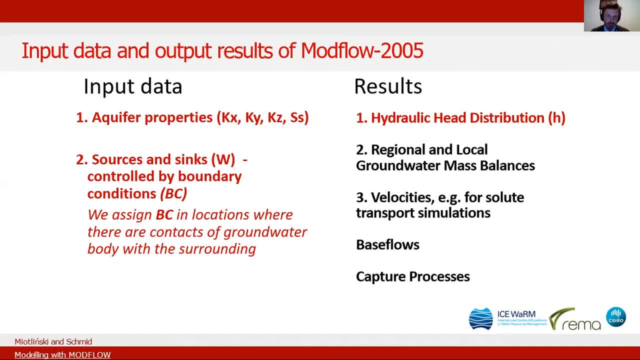 Just trying to wrap it up. It's: we have input data And those. this is the data we gathered from from from the field study, Sometimes literature surveys and so on. This includes hydraulic conductivities in in, so aquifer properties, hydraulic conductivity and specific storage. 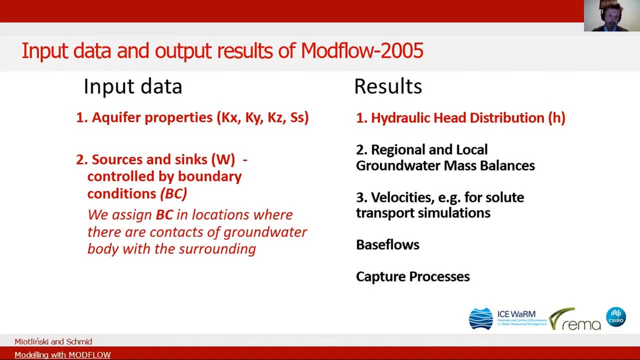 And then we have this sources and sinks The W term in the equation, And they are controlled by boundary conditions. We assign boundary conditions in specific locations of the model, Basically where there are contacts of a model or or this or of a system with the surroundings. 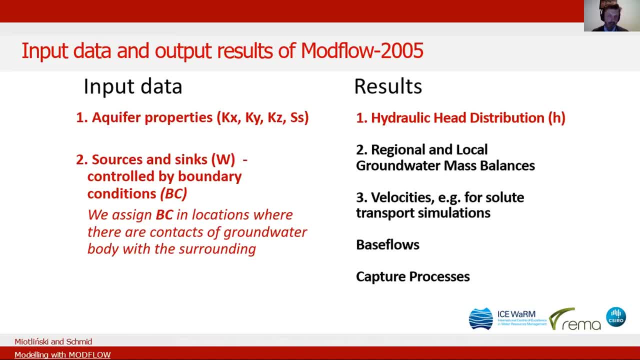 And, as a result, the ModFlow solves the equation and it gives us the hydraulic head distribution which we which can actually. from hydraulic head distribution, then the balances or the water budget is calculated. Also, velocities, Velocities may be important, particularly if we want to know, we want to use them for solar transport simulations. 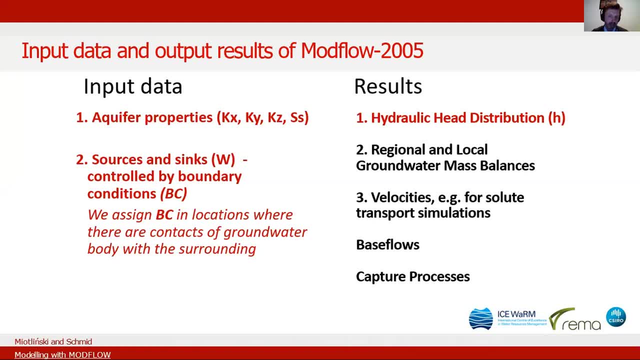 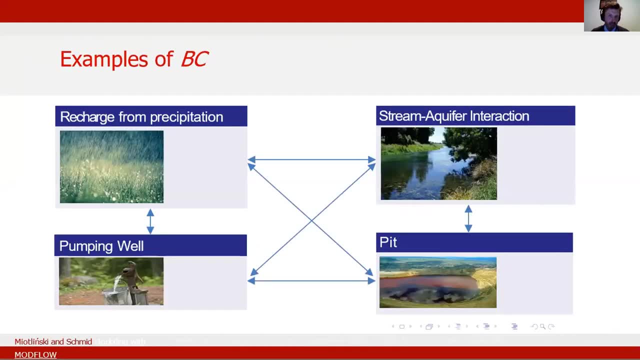 And and a couple of other things like base flows or capture processes. So the boundary conditions, the examples you can see. So this is where this is. this is how the water is exchanged between the groundwater system and the and the surrounding. 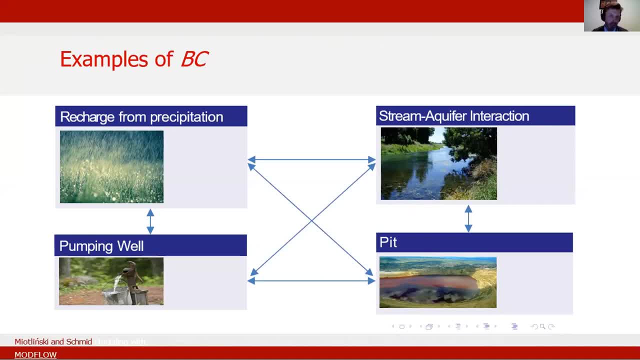 And water groundwater system may receive water, And the example would be recharge from precipitation when, when water. So this is the input of water to the system. If we have pumping wells, Then it works very, in a very similar way. The water goes back to well, it's removed from the system. 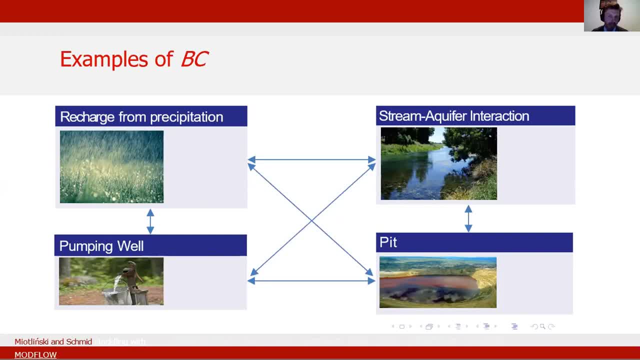 Aquifer and stream or aquifer surface water interaction are quite complicated and they can be treated in different ways, And we may also have an another example. is is an open pit or or closed mine also. It's also an example of boundary condition. 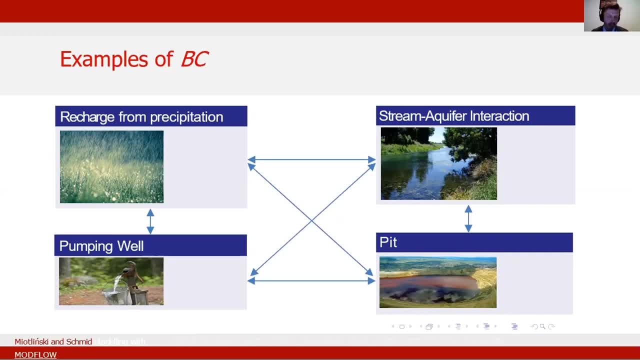 Because there is certain there is water there And obviously a pit is rarely it's well it's, it's normally very strongly connected with with the groundwater body, Particularly if there is discharge and the the the drainage of the pit happening. 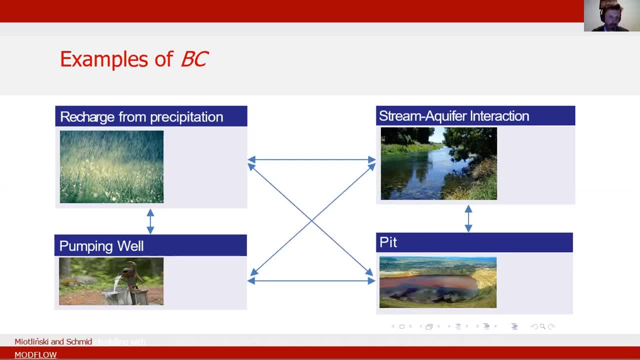 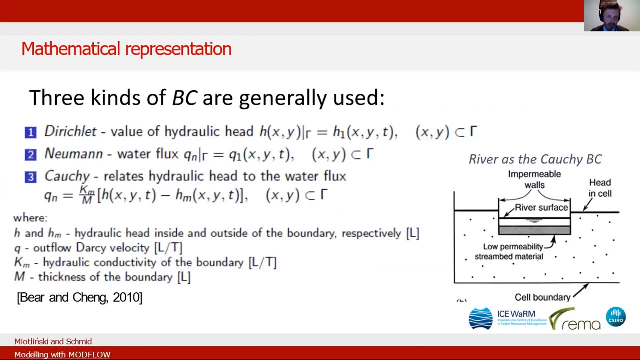 So there is, there is stronger inflow to the, to the pit And water and and groundwater system is getting depleted with water. So from a this, this, basically the there are the mathematical, the representation of the, of the boundary conditions. 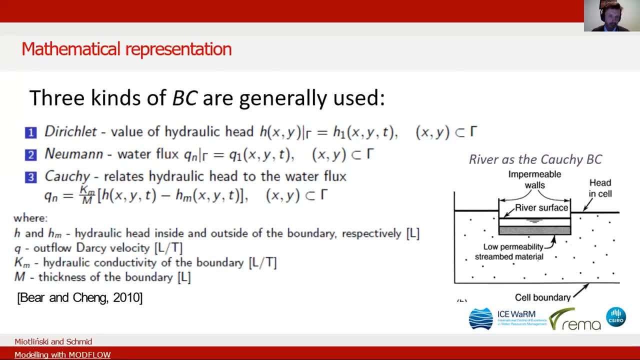 And there are three major kinds of boundary conditions. The first one, we call it first kind boundary condition. This is where there is this head specified And number of of or or the height of water. Then we may have a second kind of boundary condition where, where we specify flux of water, 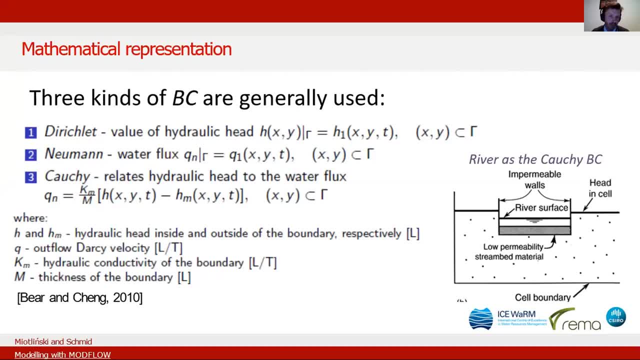 And thirdly, we have Cauchy boundary condition, which is combination of both And on the right hand side you may have, you may see, the example where there is a river, conceptual model of the river shown And a river is surrounded by the groundwater system and head in a cell next to the river is higher than inside the river. 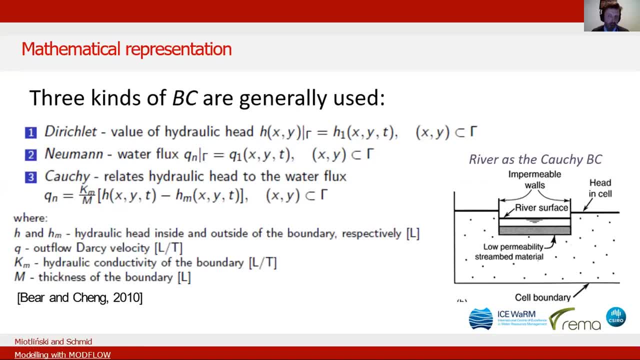 Which means that there will be flow, the river will be receiving water from the groundwater system, And and the flux or the amount of water that the river receives depends on the head difference, But also on the permeability of the streambed material. 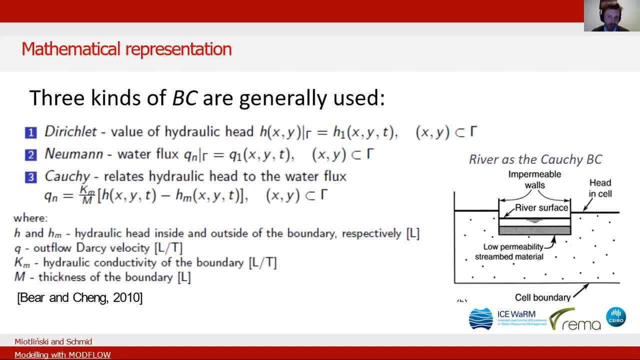 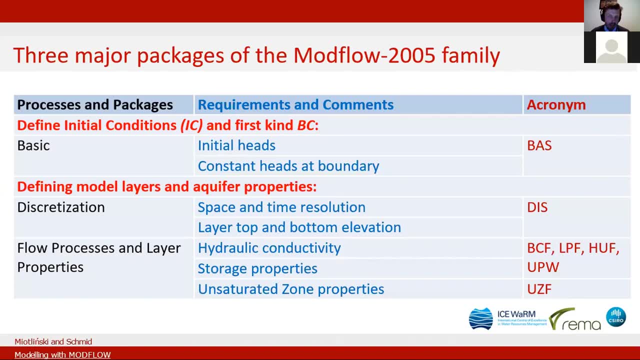 And and this equation basically on the left side, which shows this kind of situation. And so with with this classical modflow- we call it modflow 2005,- we basically have certain structure, that working structure. What we have is a number of packages, or this is basically a number of text files that are 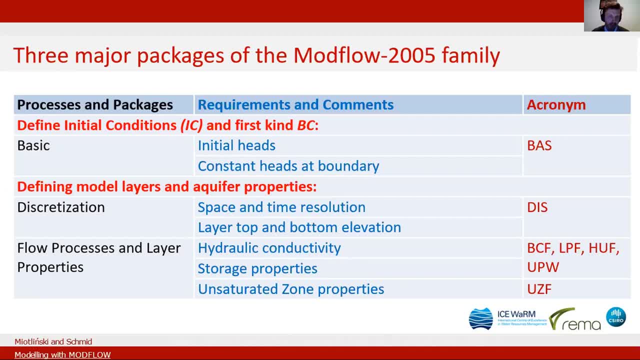 in certain in folder or in directory on your computer And each file contains certain information. So, for example, we have basic package, We may have discretization package that keeps information about spatial and temporal discretization, So the spacing between the cells. 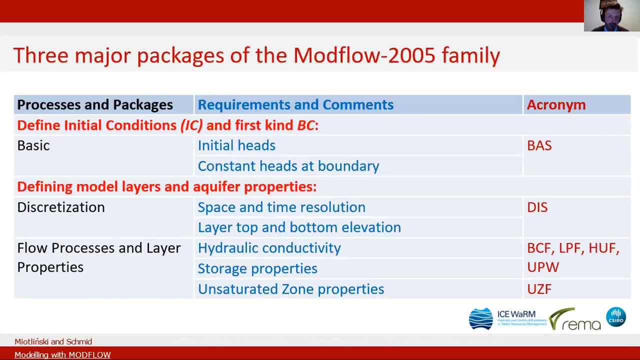 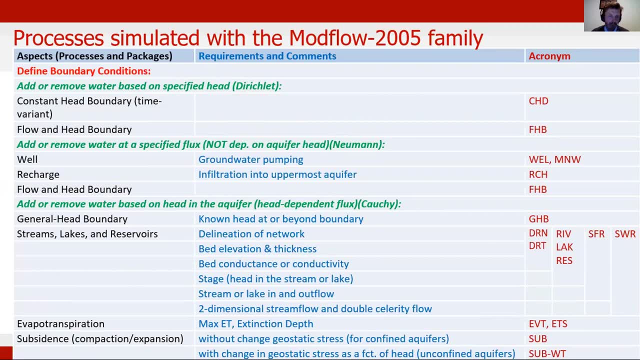 We may have information about the aquifer properties And there is number of other packages that are responsible for for this exchange of water with the surrounding, I imagine. So it's it's basically the boundary conditions We have first, first time boundary condition in the first group. 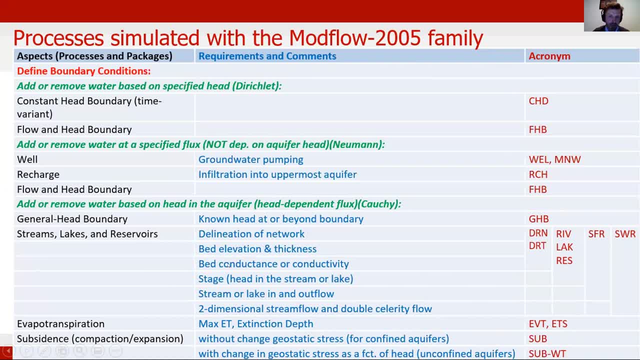 Then we have second kind of boundary condition and third kind, And you you may have. you have a list of them, Some of them quite specific: Extreme flow routing package Or evaporation packages, Subsidence, As you can see here, it basically shows you the what kind of processes can easily be modeled with with modflow. 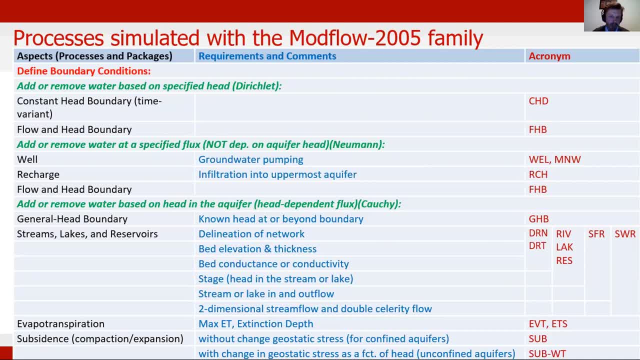 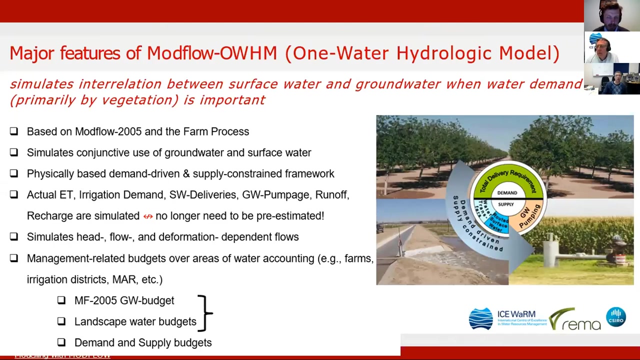 And, and, and, and, obviously in further reading, can tell you whether this would be appropriate in certain situations. You may be interested, And at this moment I would like to pass to Wolfgang, who will be talking about modflow home. So but I will. I will come back a bit later. 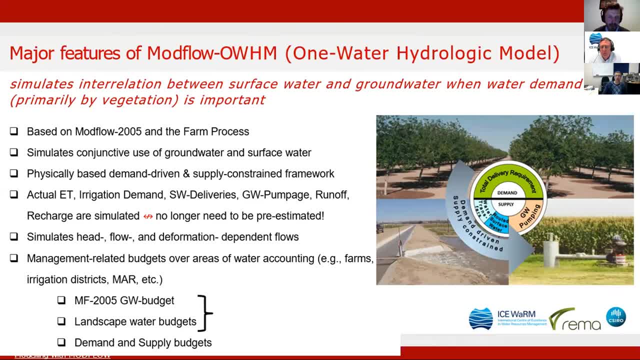 Would this be a good spot to just take a couple of these questions? They're coming in on the Q&A board. You might notice there. Wolfgang and Konrad, Are you okay if we just take a couple of these questions now? We won't take them all, but maybe just just a couple of them. 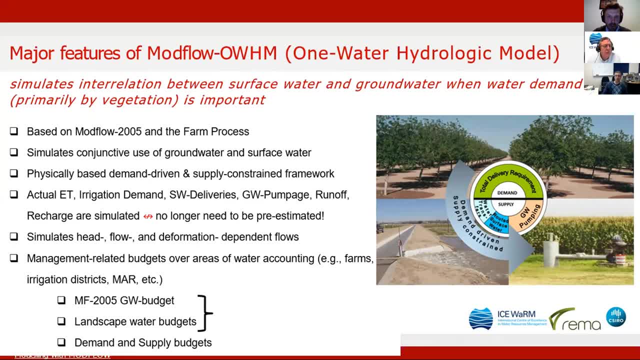 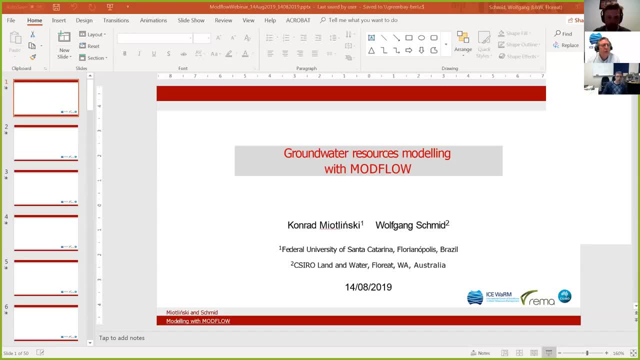 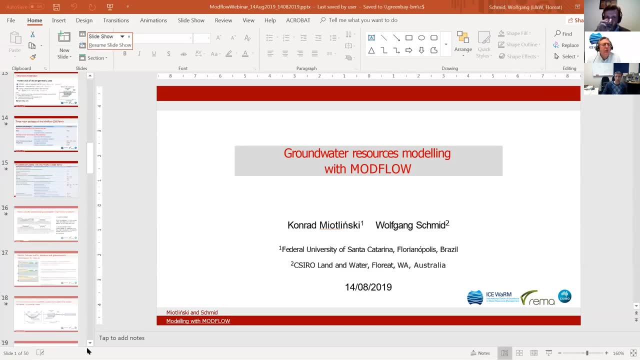 Just keep, keep the keep the discussion going. Well, look, Suzanne McDonald is a water treatment technologist in in GWM water in Australia, New to modeling. Her question was pretty broad and pretty, pretty open. Is modflow the best package? 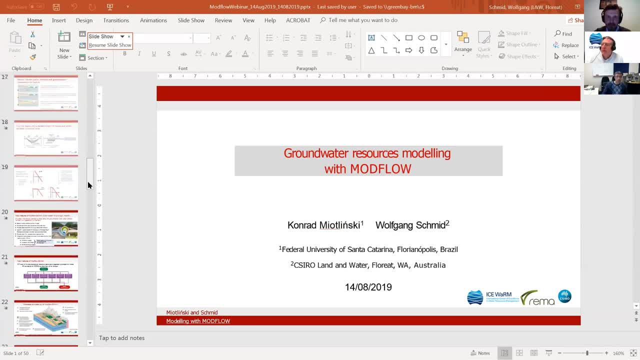 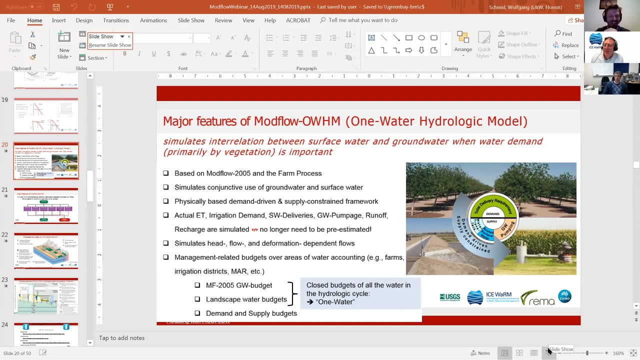 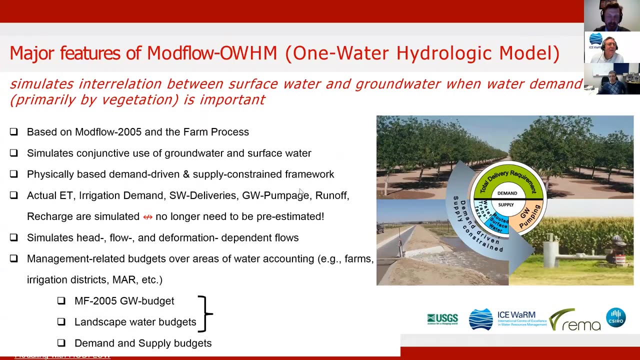 Is there a good course you could recommend? to get me started, We do have a good course. Very good question. Well, basically, Suzanne, It's, it's definitely very robust package, but everything depends on on the scenarios you may have, the objective of your modeling. 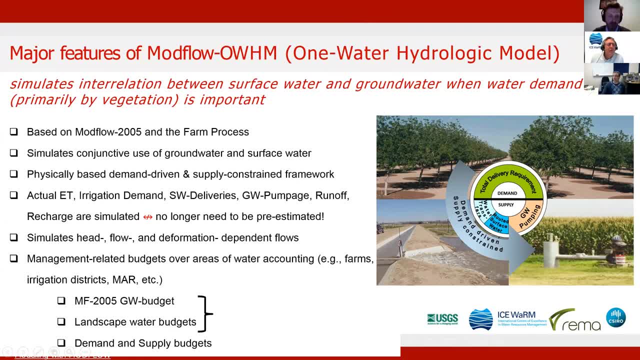 I believe there is no package or no software in groundwater market available that can. that can be called that. oh, this, this is the best. Everything depends what you are looking at. For example, if you are, if you are interested in hydraulic fracturing or multi-phase flow, probably modflow is not the best choice. 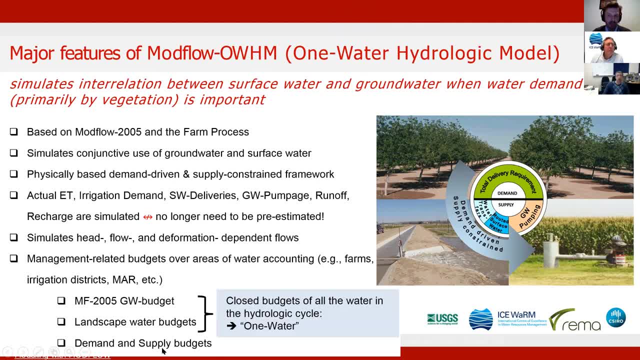 But if you, if you want to calculate groundwater or estimate groundwater resources in Great Artesian Basin, modflow would be definitely one of the of the softwares you should, you should consider And and is there a good course? 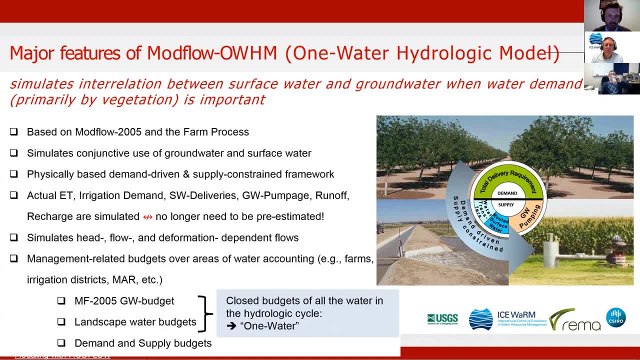 Well it's, we will be talking a little bit about this later. If- and we will show you something in a in a few minutes, maybe let's skip it for later, then, Sure, We do have three online courses coming up in October, December and February. 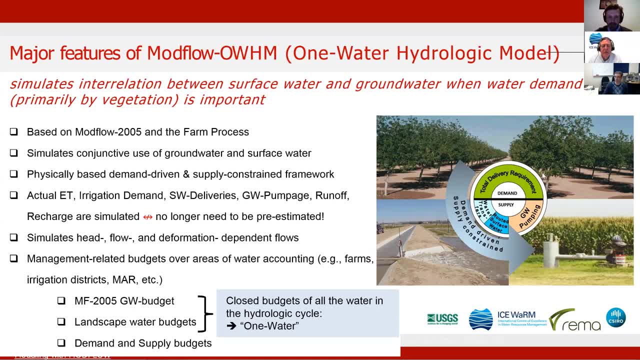 By Conrad and Wolfgang. we'll talk more about that later, as, as Conrad says, Any comments Wolfgang on that question? No, no, Okay, so we'll move on. Thanks for the ample question. One more question then from Tahira, a senior engineer in Canada. 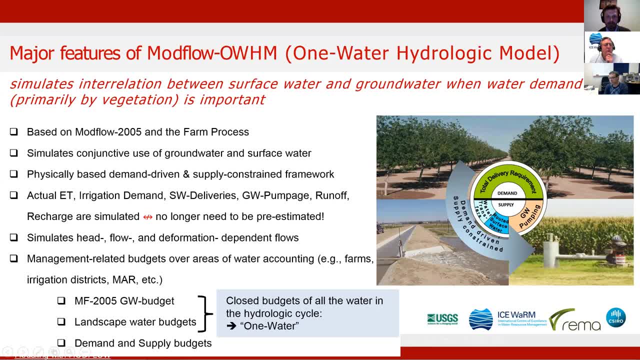 What type of input data is required to run the model in modflow? What's the basic data platform, common source of data? What's that second question? Oh well, it's the input data I I mentioned Just a few minutes ago. 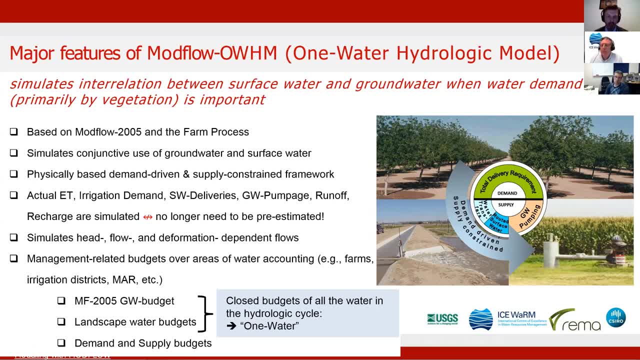 It's what, what we really need from from. from the mathematical point of view, We need hydraulic conductivity, specific storage and we need fluxes to the system. Is there any any platform that provides you this data? Probably there is no. 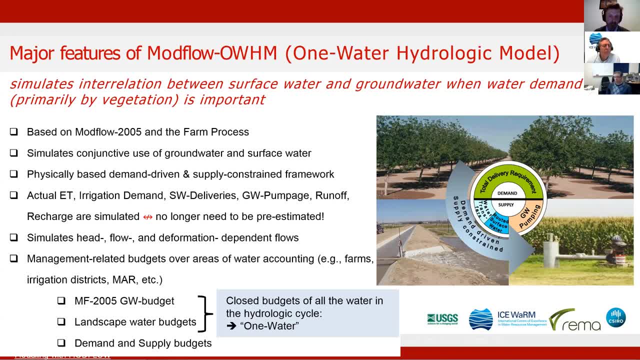 It also depends where you work And, well, from my perspective, I always, I, well, I, I work in different parts of the world And and I'm getting data, I'm getting. firstly, I'm asking person, who, who want me to develop, who wants me to develop a model? 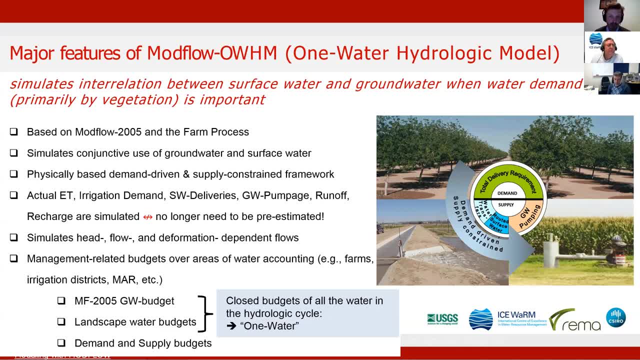 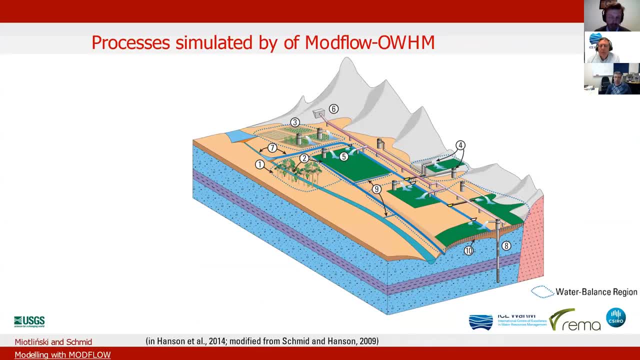 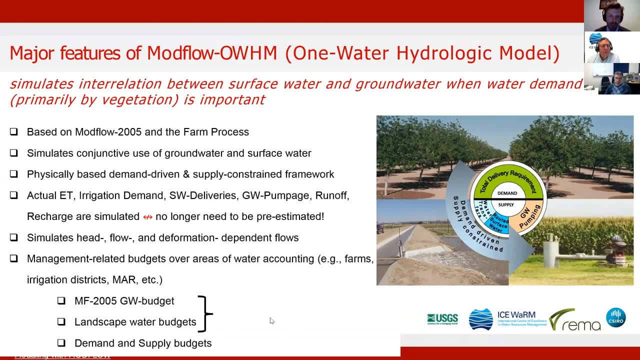 And I will ask him what kind of data is available and whether they can recommend any, any sources of data, And and, and. if they don't know, obviously I have to look by myself. But there is no, no one platform that may have everything, all data available that you, you can run a model. 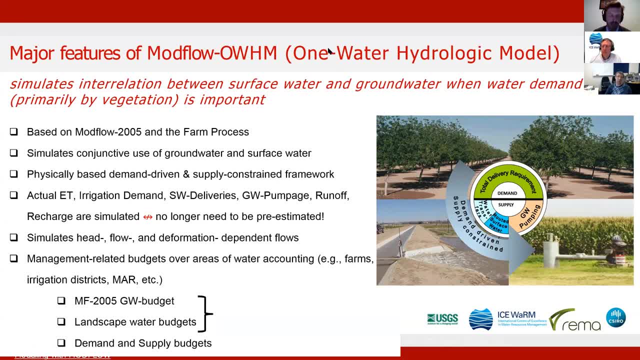 for again, it depends what kind of objective you may have, Because we we may also run a model without much data. Obviously this will be a model that is quite uncertain, Or the results may be not very certain, And sometimes we have to work in very in in areas with very little information. 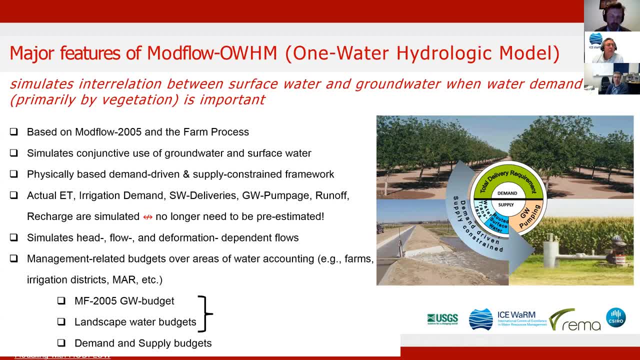 And we also have to do something. So, yeah, so this is basically it. what I would probably could say about this, And just one additional question from Tahira, Is: is a capable Modflow capable to calculate groundwater quantity and groundwater quality as well? 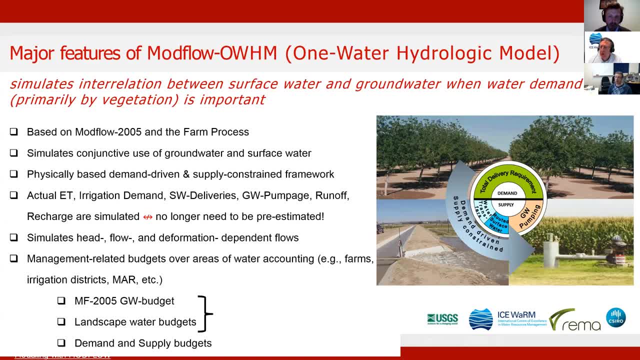 The answer is no. The answer is no Because you need. you need another code for that which is called MT3D, HT, MT3D, MT3D code. Yes, right, Yeah for for for quality, for quality. 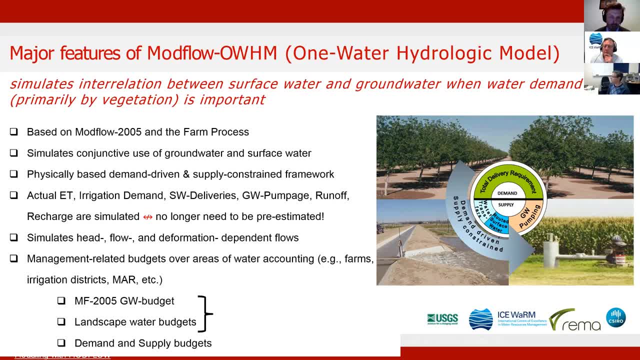 Or yes, so it's, they work together. So Modflow, what Modflow does? it calculates heads and basically velocities. And another software uses velocities calculated by Modflow And it does the calculation of, of solid transport, And that includes advection, dispersion, and well, basically advection and dispersion, but also diffusion. 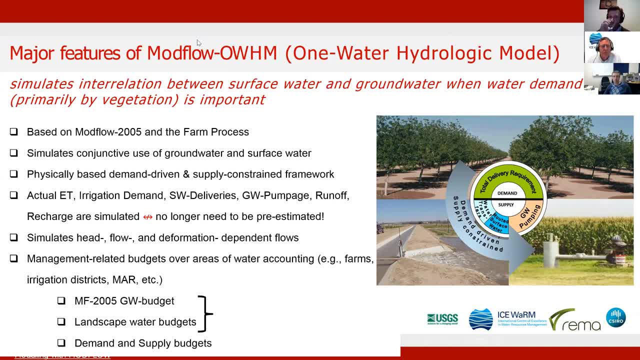 Yep, Okay, We might leave the questions there. Thanks so much. There's more questions coming. We'll come back to those questions again. Stay online there. Sunita Priscilla, Sid Nathan Adonis, I can see your questions coming in. 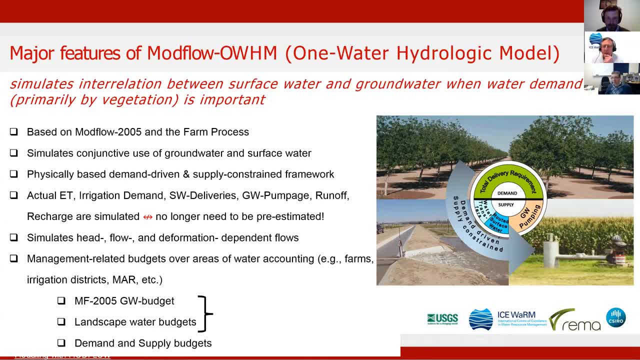 That's fantastic, But we'll move straight across to Wolfgang. now We're going to have to keep our questions, our answers- sorry, Wolfgang Conrad- keep them short, Because there's a lot more coming through as we go And there's a lot more material that we're going to be presenting. 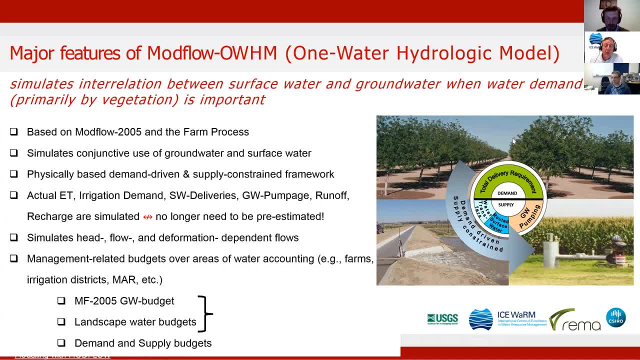 Thanks both of you so much. But I would say to everybody, go on the website, LinkedIn, Facebook, Twitter, And you'll see the online courses coming up for beginners in Modflow and groundwater modelling. There'll be three courses coming up in October, December and February. 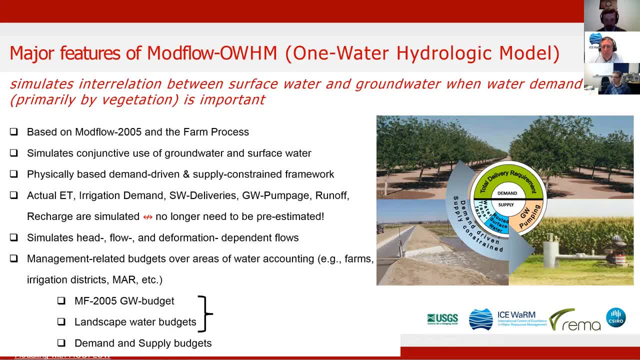 Across the next six months, we'll be presenting both Conrad and Wolfgang. presenting that, All right. Well, let's press right on Over to you. Wolfgang, Might have to come a little closer to the mic, We can hear you, okay. 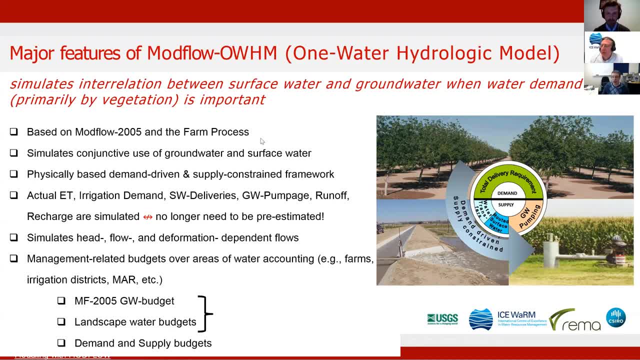 But just a bit clearer. Okay, Let me just ask you A little bit echoey, That's all. Are you seeing the presentation that I'm running off? We can Yep, Perfectly, Thank you, Yes, So are you going to see this? 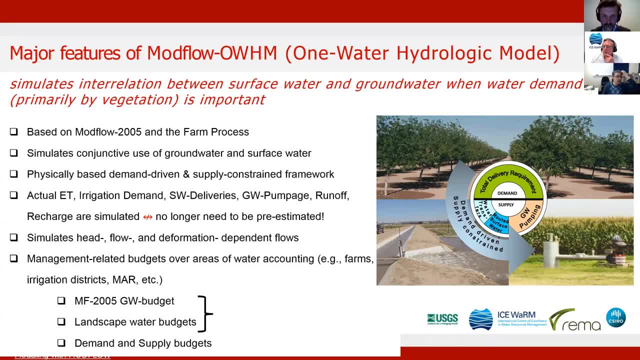 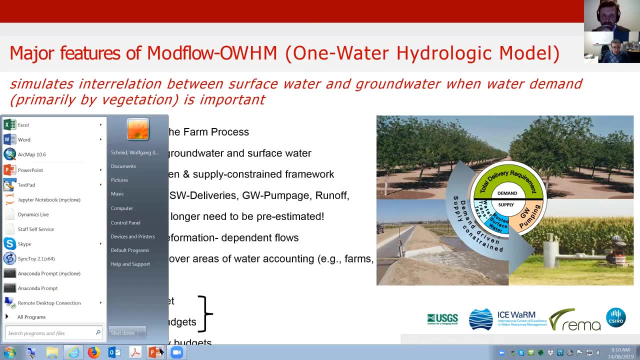 That I'm changing this slide. Is that the presentation All clear? Yep, Okay, So in addition to what Conrad was saying about Modflow 2005.. Obviously, There are different versions of Modflow out there now I just need to see you guys. 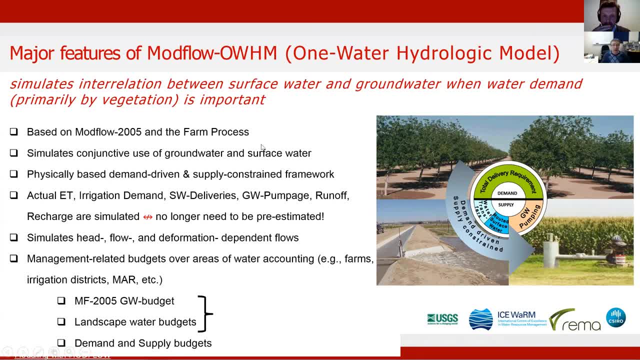 Move that over here. All right, Thanks. So the main difference between Modflow 2005 and Modflow One Water Hydrologic Model is that Modflow One Water Hydrologic Model is a more advanced version which you only want to use if you're really interested in management questions and water demand and supply questions. 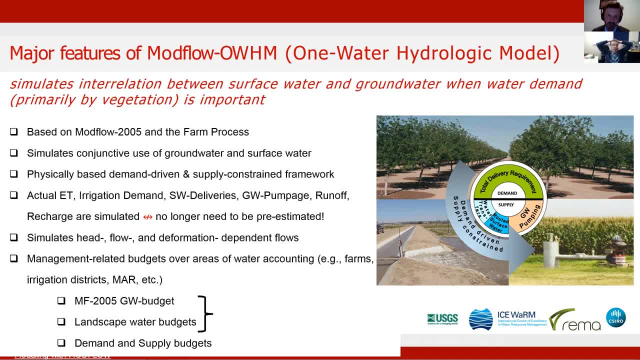 And it can do everything that Modflow 2005 can do as well, And it's based on the farm process. So what that means is the farm process actually drives the demand calculations and the supply constraint or the constraint supplies, And so basically these three, if you can see my mouse moving. 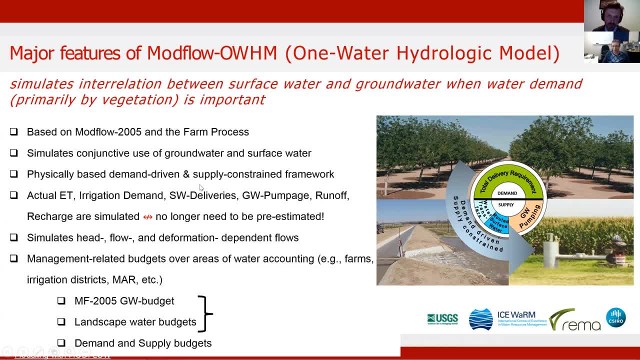 So these three points actually belong together. So, in other words, it calculates the actual ET, which is contrary to what Modflow normally does. All that Modflow normally does is ET from groundwater, So it simulates the entirety of ET and the resulting irrigation demand that you can. 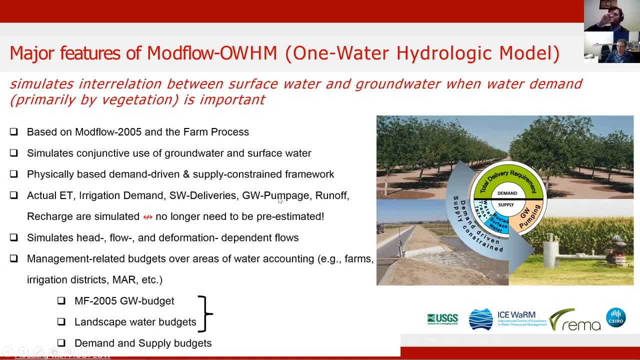 pick out from it And then subsequently surface water and groundwater deliveries And runoff and recharge are byproduct. Now you remember what Conrad said about, for example, recharge. That's a specified boundary condition normally, But in this case recharge becomes a simulated parameter. 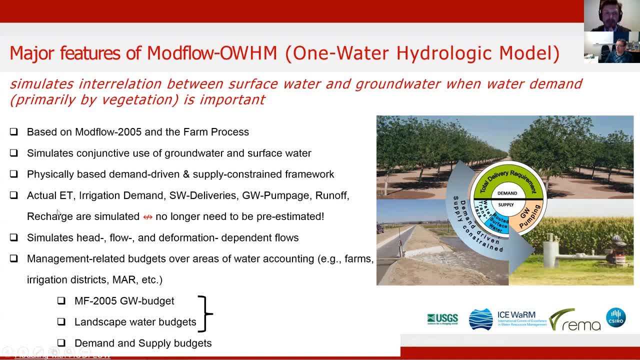 So in other words, this is a model output, just like hydraulic heads or velocities. So in other words, if you drive the system with demand and constraint supplies, you're going to have a lot more simulated parameters. that is pretty good to simulate those, because 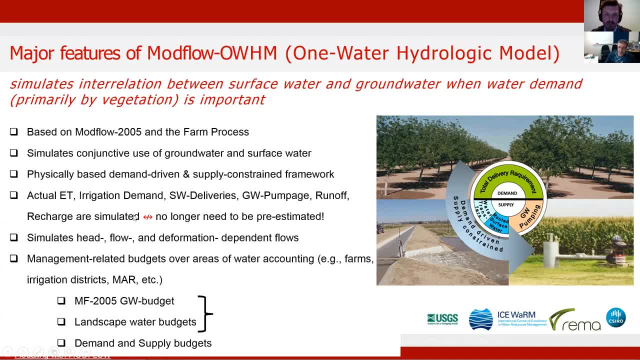 they are highly uncertain. So those are parameters that later on you would like to run uncertainty analysis on. The next difference is that normally you have, like Conrad said, you have non-head dependence and head dependent boundary conditions. In this case, a lot of the processes from one package depend on the other package's flow. 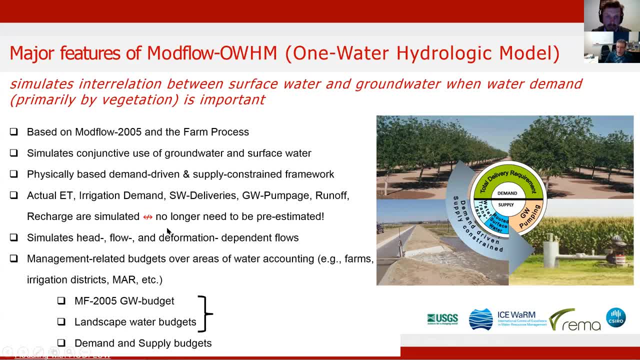 meaning it's flow dependent. And then we also feed back the land subsidence deformation on the land surface and the layer tops and bottoms into how that affects the flows of each package. So that's another difference. And lastly, the next difference is that Modflow Home can calculate the flow. 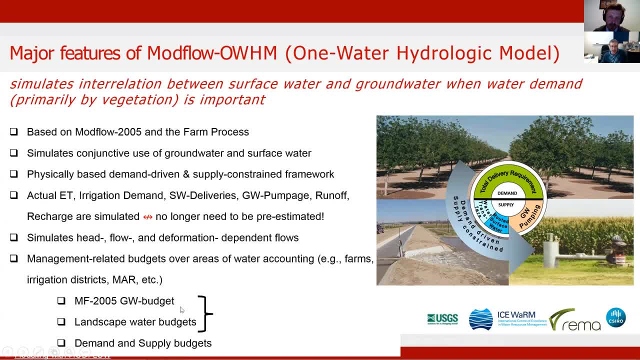 of the ground water patches, just like macro 2005 can, But in order to simulate all water in the hydrologic cycle. we also have landscape water patches. We used to call it just farm patches, but actually for larger entities like irrigation districts or water accounting areas, we like to call them now landscape water patches. 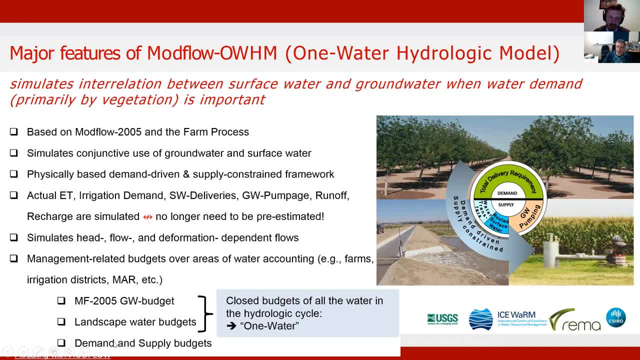 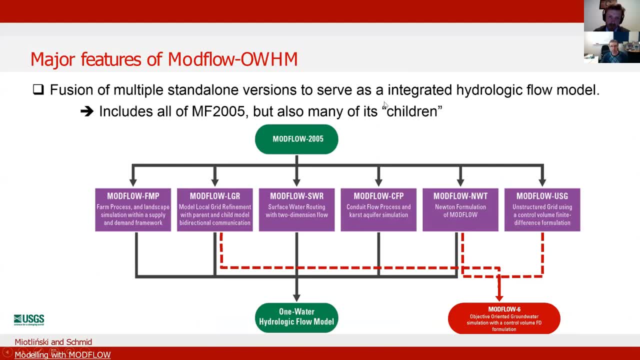 And lastly, as I said before, it can also be used to calculate the flow of the water and calculate economic batches. so demand and supply. Now Modflow Home basically also fuses a lot of standalone versions into one integrated hydrologic flow model. 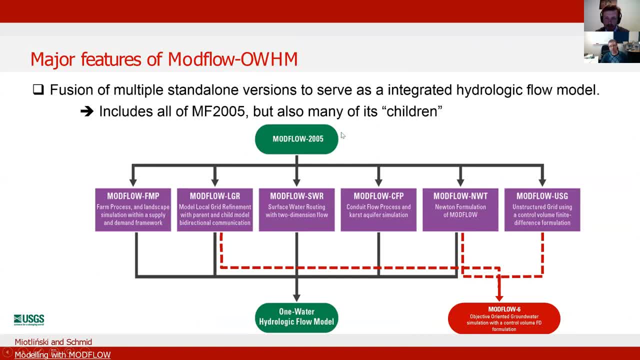 So it needs to be understood that there were a few years ago, just a few years ago still, a lot of successors of Modflow 2005 that had a specialty that stood alone, like local grid refinement, the surface water routing process, conduit flow process, the Newton-Raphson solver. 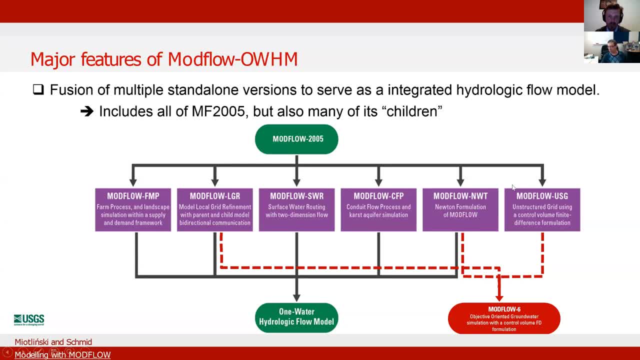 for mainly unconfined conditions, with a dry wetting problem and the unstructured grid and the farm process that I was involved in. Now Modflow Home fuses a lot of those together And later on we will talk about Modflow 6 that also fuses some capabilities of some. 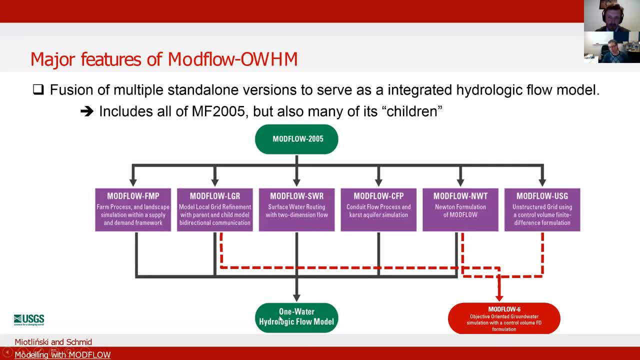 of those packages together. So this is why I said at the beginning: Modflow isn't Modflow anymore. People really need to know what they want. They can use each of those standalone versions as well, or they can use Modflow Home, if it. 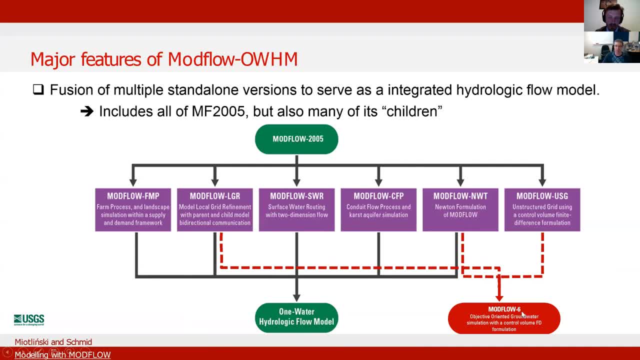 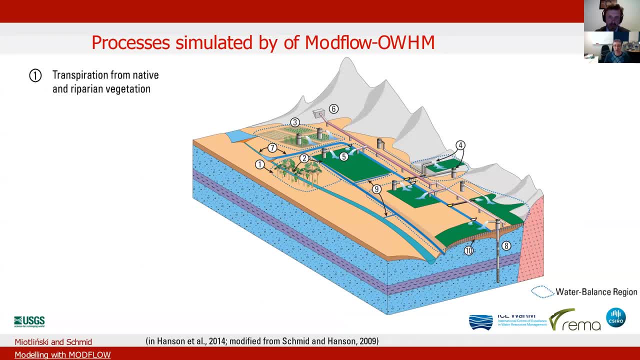 suits their application, or they can use Modflow 6.. So it really depends on what you want. Now in Modflow Home, based on the farm process, you can simulate all the transpiration and evaporation from native and riparian vegetation, a natural artificial recharge, and then you 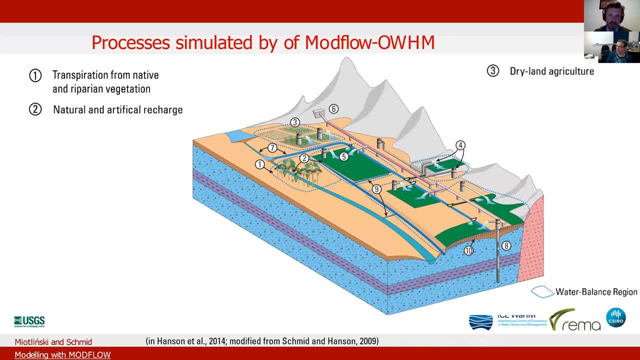 need to know which demand you would like to calculate. So either you have the demand of dry land agriculture, or of aquifer storage and recovery systems, or of irrigation systems. So these are all the main units, And then you basically supply them with known water quantities, say, for example, imported. 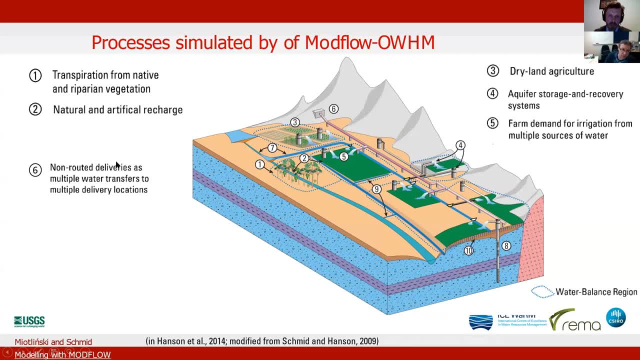 water pipelines that we call non-routed deliveries, or routed surface water deliveries, or groundwater pumpage. Now, the in excess of precipitation and irrigation, in excess of the crop water demand will then be runoff and delayed recharge, And if it's hooked up with unsaturated zone flow, then it may even be delayed. 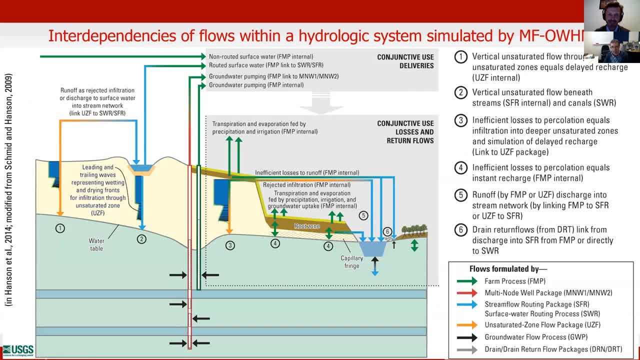 Now in this slide. I won't go through everything here. That way it will take much too long. But this is for people who are more interested in Modflow Home. But as an example, you can see here that the stream, The delivery from the streams, is hooked up with the conjunctive use of the farm process. 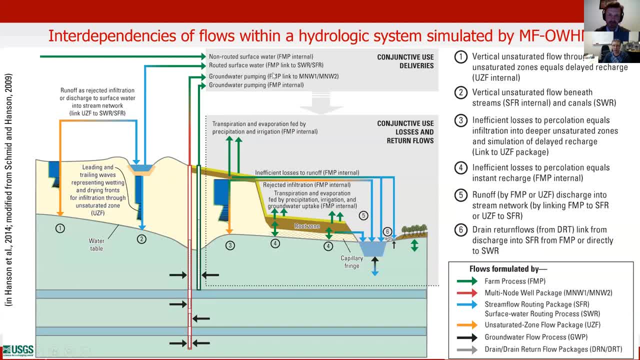 or pumping. The supplemental groundwater pumping is hooked up, for example, with the multi-node well package, So you basically pass on your demand onto the streams and divert automatically all the residual requirements onto the multi-node well package, where otherwise you would have to hardwire your desired package. 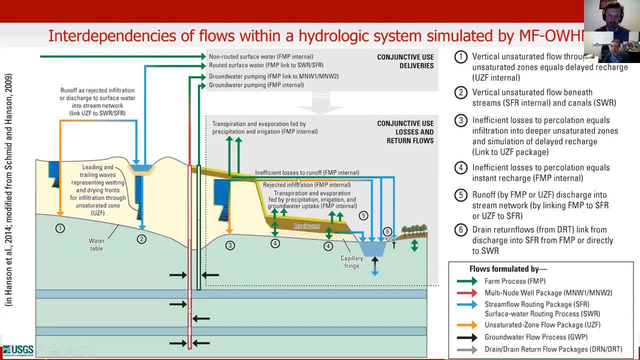 Likewise, the return flows are either inefficient or not, So you can see losses to runoff and back into the river, Or they are going into the unsaturated zone flow package in order to calculate delayed recharge. This is why we call it one water hydrologic model, because it simulates all the water. 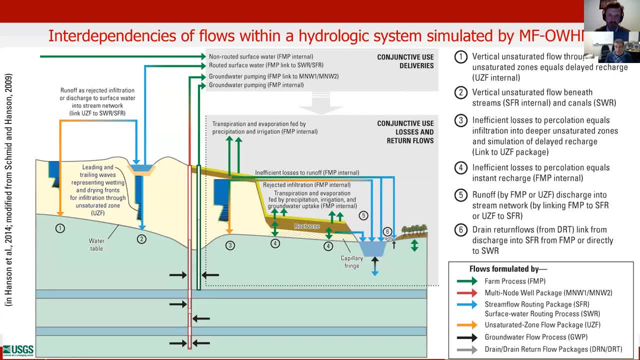 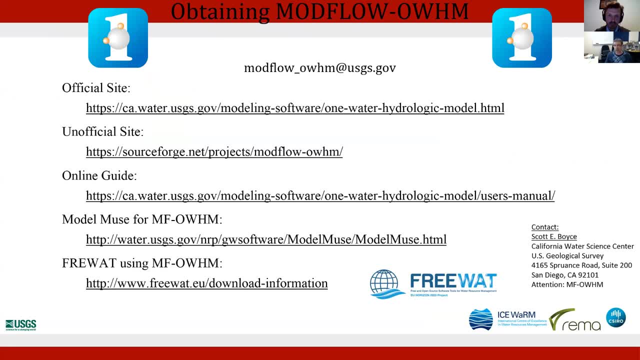 of the hydrologic cycle at all times. Now, this slide I just put in this morning, this I just want to have for the record. So if somebody is interested in obtaining Modflow Home, these are the internet links that you can get it from. 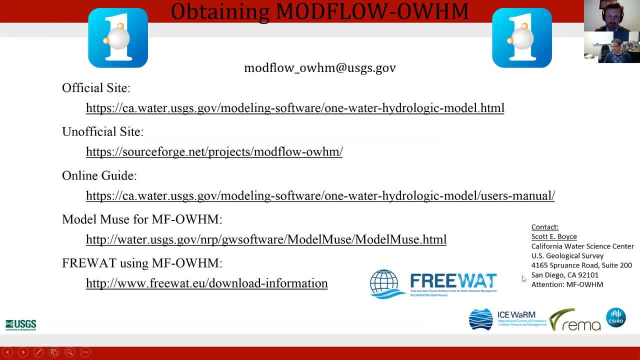 And just the last comment. So Scott Boyce right now is in the driving seat of developing old version 2. And that should come out within the next few weeks or months. And that is basically all from me for now. So back to you, Conrad. 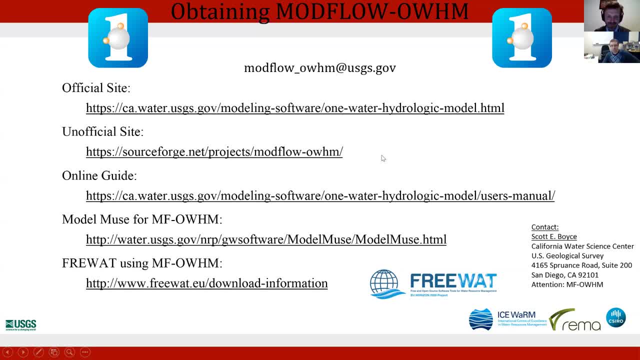 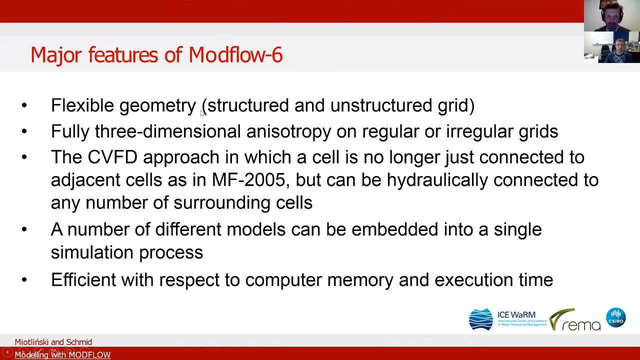 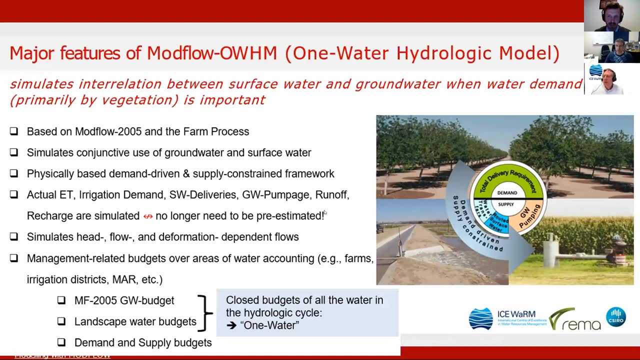 Now the next slides will be Modflow 6.. Yep, And then you can take my presentation away. Yeah, I've already done this, Conrad. would you mind if we took a couple more of these questions, just briefly? Yeah, sure. 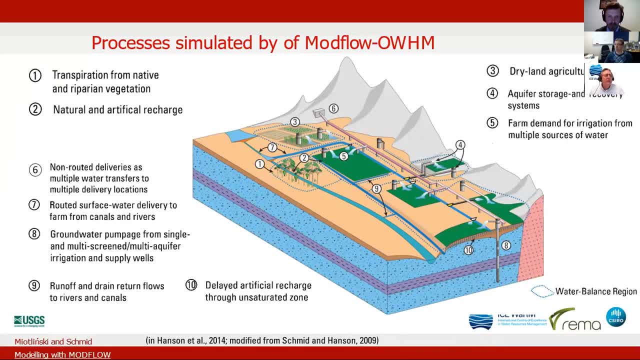 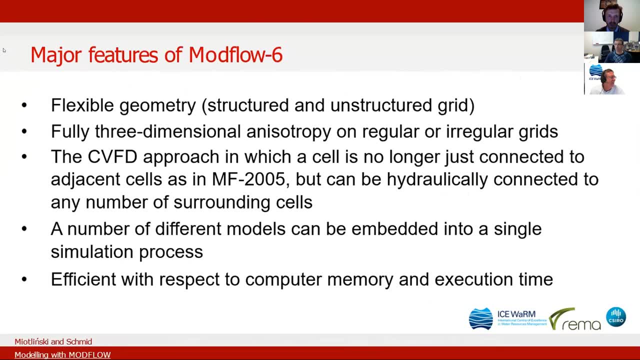 Sure, No, not a problem, All right, Nathan Young is a senior water- No, no, he's not, He's not, Not in here- A senior staff at Schnabel Engineering in the US And he said: is it typically recommended to calibrate a steady state bridge? 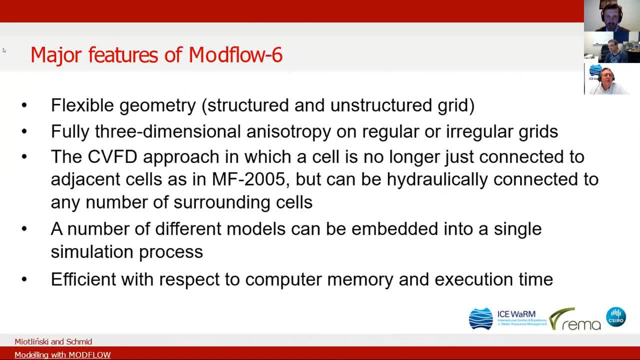 groundwater model before running and calibrating the transient scenario? That's the first question on your Q&A list at the bottom there: Yeah, short answer would be yes, Ah, that's one he wants to hear. That's good, Maybe we'll leave short answers for now. 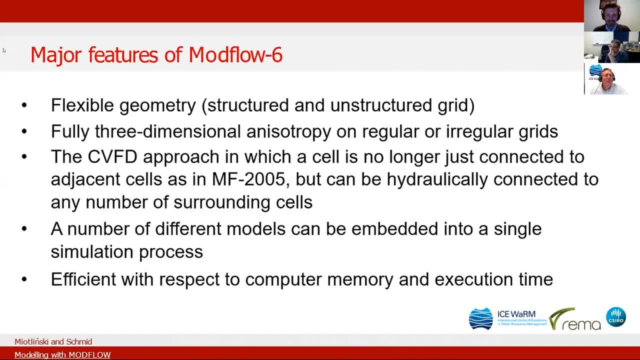 Is that okay, Or is there something you'd like to say extra? Yeah, I mean, the short answer is yes. A lot of times nowadays, when you deal with uncertainty analysis, you actually bypass the calibration path because you're dealing with the depth and breadth of the uncertainty. 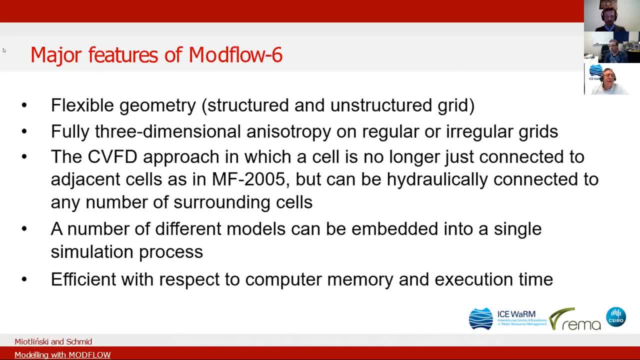 that can happen, But this is a very different topic. So in this class I don't think we go into. like Conrad said at the beginning, remember these three blue boxes. So the question of calibration and uncertainty is outside of the topic of this class. 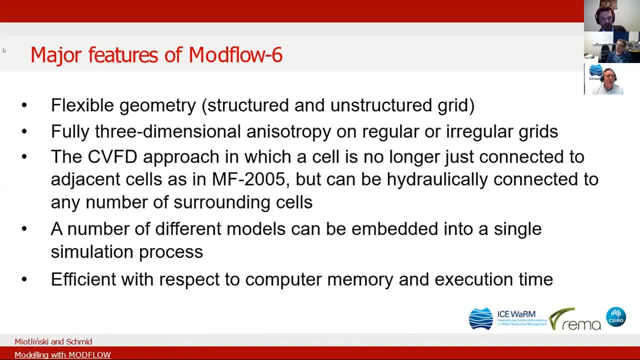 Yep, So this webinar is fairly brief, but do come to the short courses, Nathan. More detail will be provided there. for sure, Sunita is from Rockhampton, Australia. a senior environmental scientist with EcoSure in Australia has said: can mod flow be used to model groundwater surface water connectivity? 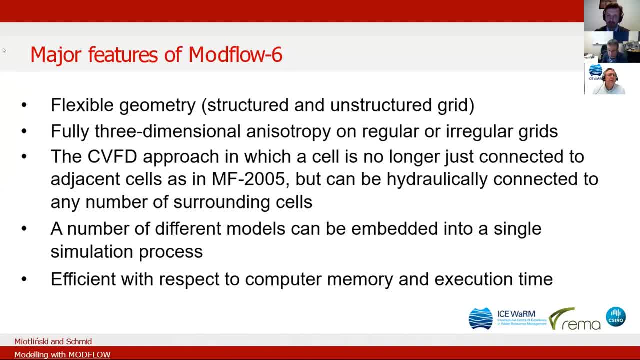 Yes, absolutely. As you can see, especially with MAFRO, one water hydrologic model, the interaction between surface water and groundwater is absolutely critical. This is absolutely a given now, And I'm talking both about the landscape groundwater interaction as well as the stream aquifer. 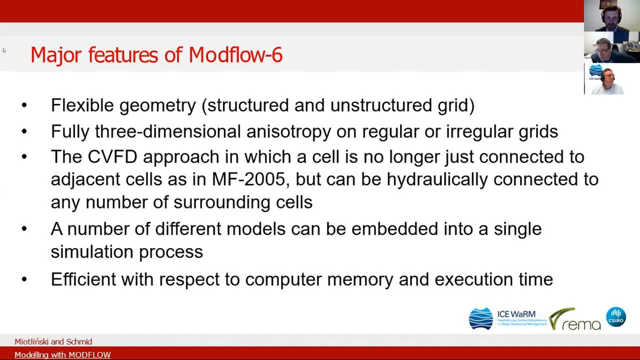 interaction. I would like to be quite specific about this because a lot of times people confuse the two. They talk about surface water groundwater interaction. In many cases they just mean stream aquifer interaction And there are different tools out there. So, as you can see, with MAFRO it's more about having surface water groundwater interaction. 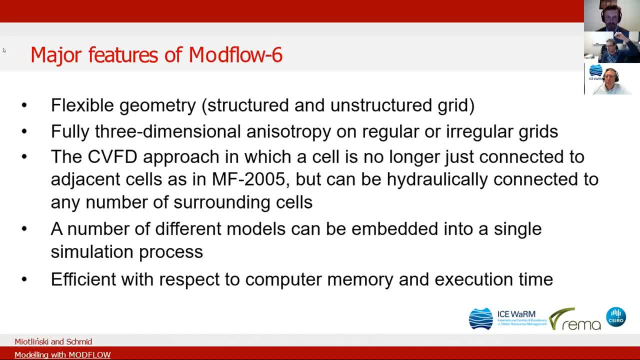 in the sense also that you have surface water and groundwater to satisfy your demand. But, for example, if you want riverbank infiltration and two-dimensional flooding, there are tools out there that go beyond what Konrad is talking about. In addition to the stream aquifer routing package, there is the surface water routing. 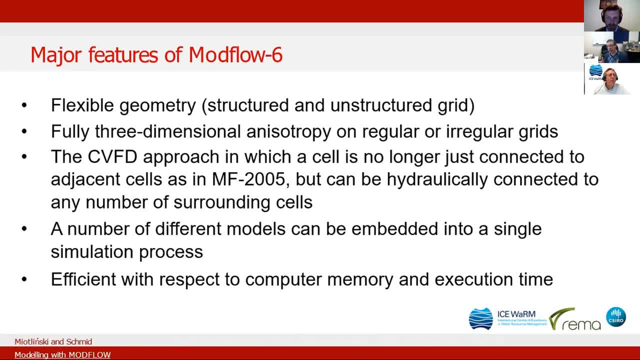 package out there which actually can simulate the St Benans equation. So it actually simulates really a wave of flow in two dimensions And that is all done in MAFRO. So that's why I said at the beginning, MAFRO isn't really MAFRO anymore. 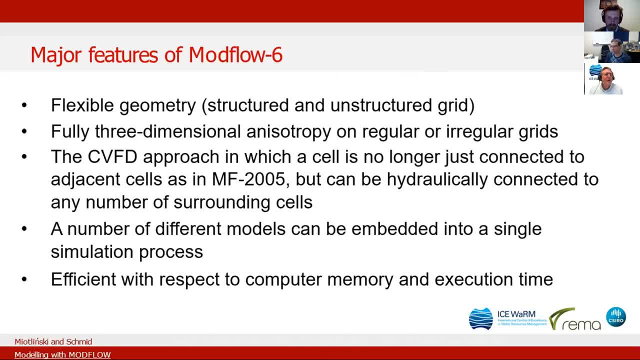 And it goes way beyond groundwater modeling. Yep Sid's a mining engineer with Energy Australia. How can we import 3D geological model layers in DXF and DWG format into MAFRO? Wow, Yeah, Wow, There are definitely. 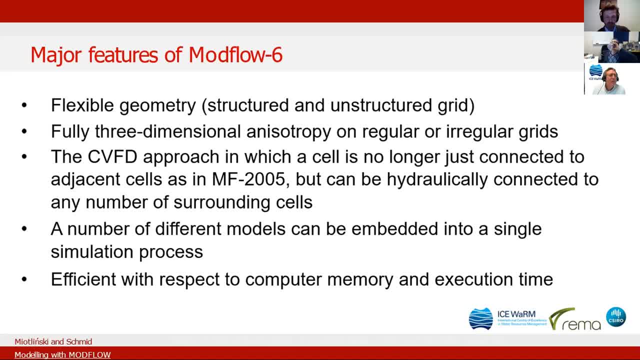 So to do this you need the graphical user interface, the way you import specific information into model. There is a number of commercial interfaces that can do this very easily. In open software you can also do this. You can do this particularly using some tools like FlowPy. 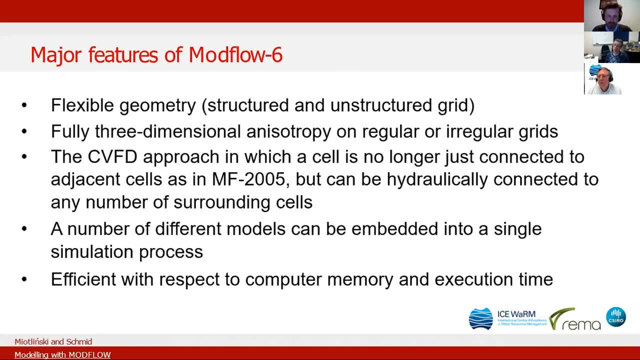 I'm actually not sure about these specific files, whether you can use Model Muse, But Model Muse has also some importing capacity capabilities, So we would have to check whether these particular files can be imported into Model Muse. Any comments? Wolfgang on that. 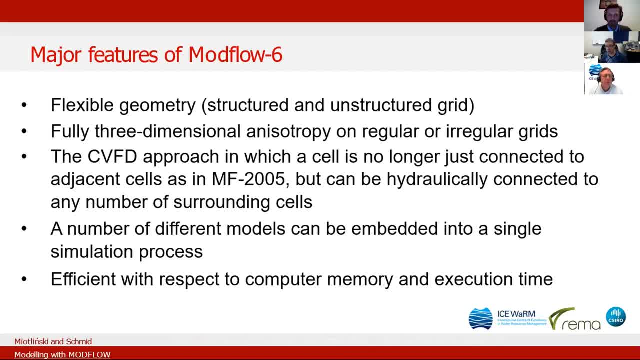 No, not at all, That's all right. Okay, All right. Thank you, Conrad. I'm keeping these responses short, sorry, gentlemen, because there's many, many more to come. Maybe we'll stop there for a minute. 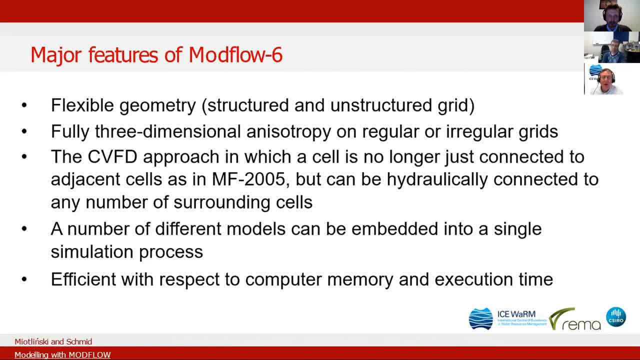 And we have 10 minutes toward the hour, the end of the hour for our webinar. We might be going a few minutes just beyond the hour, but let's keep it as brief as possible. But I would recommend to everybody that you sign up, register for these online courses. 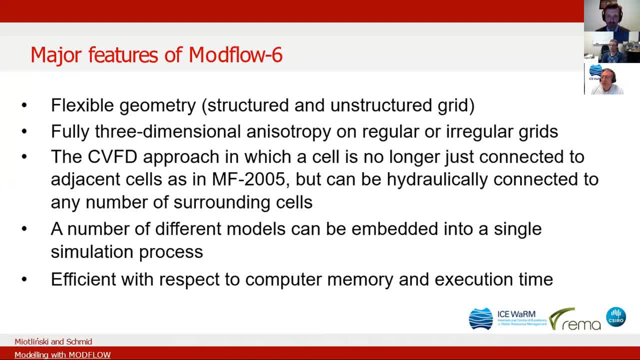 They will get to some of the issues here Over to you then, Conrad, Thanks. So now I would like to tell a few words about Modflow 6.. Modflow 6 offers you flexible geometry. So it's not Well, it's also. 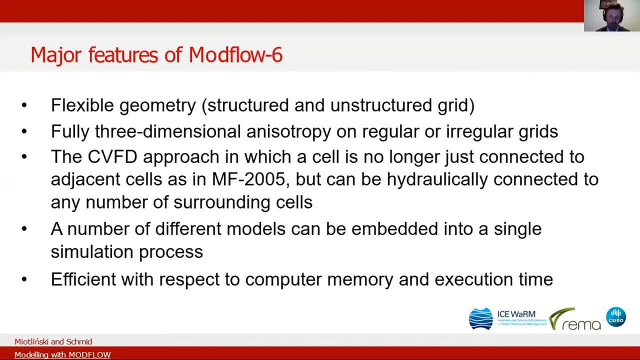 It can be used the regular grid, as we've shown before, but it can be. We can also use unstructured grids. It has some additional features and they include fully three-dimensional anisotropy on irregular grids. The computational approach used here can be. 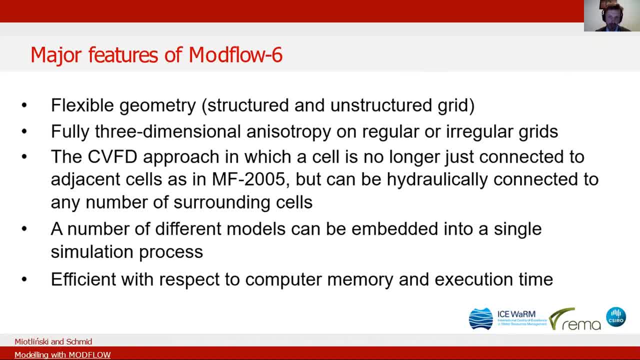 Allows us that, numerically, The cells don't have to be adjacent one to each other in order to simulate flow between them, So this is something very interesting and in certain circumstances, may be very useful. A number of different models can be embedded into a single simulation process. 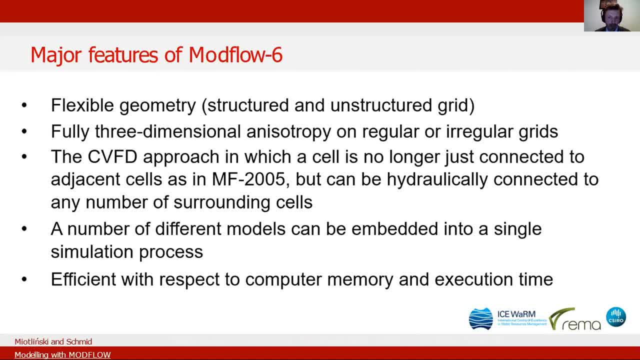 For example, you can model surface water independent of groundwater model, but they are still under the same umbrella. Then it's due to unstructured grid properties. it's quite efficient with respect to computer memory and execution time. There is probably. no, We don't have probably much time to talk. 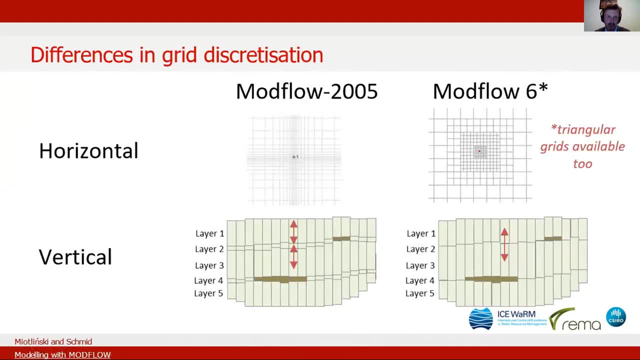 In very much detail about this, but I would like to show you a little bit more about the discretization. So in a horizontal, if you look at the plan view, we In a classical Modflow 2005,. you can see if you have your area of interest, what you normally needed to do in the past. you. 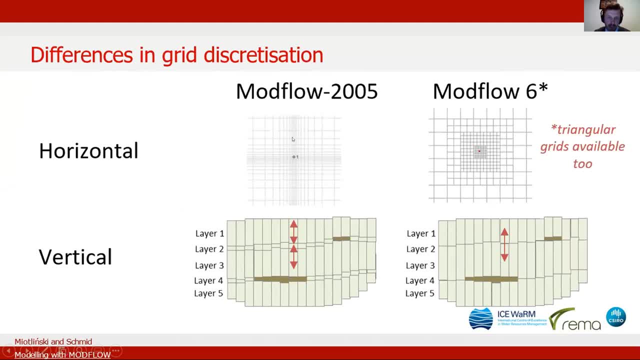 Well, still in the Modflow 2005.. You have to extend If you want to refine this area of interest. this refinement goes across the whole model domain And in Modflow 2006,. this is one of the ways to refine the area of interest. 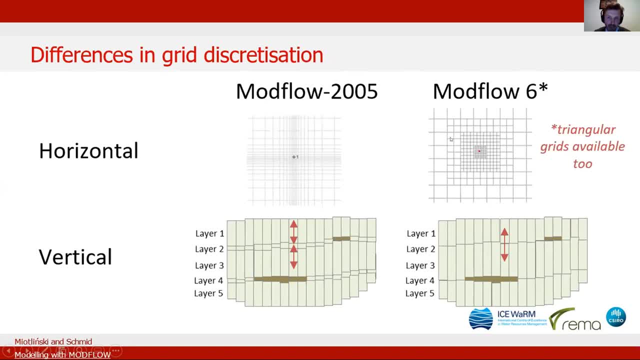 So by doing this you have much smaller number of computational cells And this saves you. There is some computational efficiency gain, And then in vertical direction we also gain a little bit more, because in classical Modflow 2005 or Modflow OM, 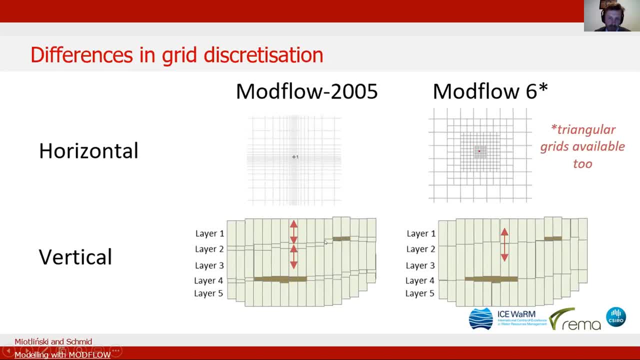 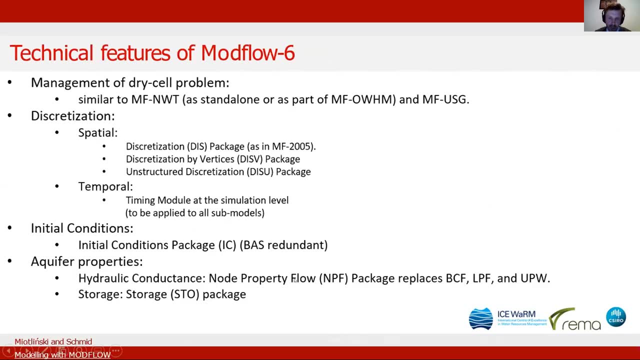 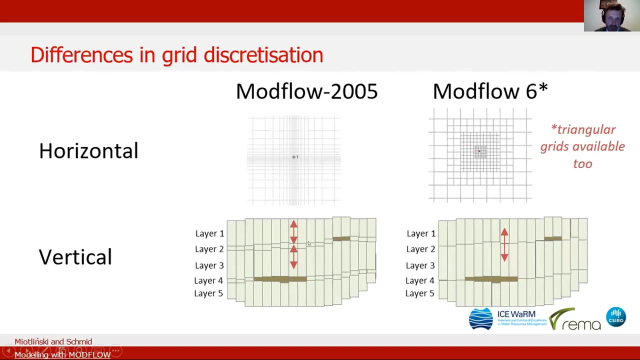 what you need to do. if you model, If you have layers that are discontinuous, geological layers that are discontinuous, you may still have, You still need to. In order to represent them, you need to put a layer inside And, obviously, 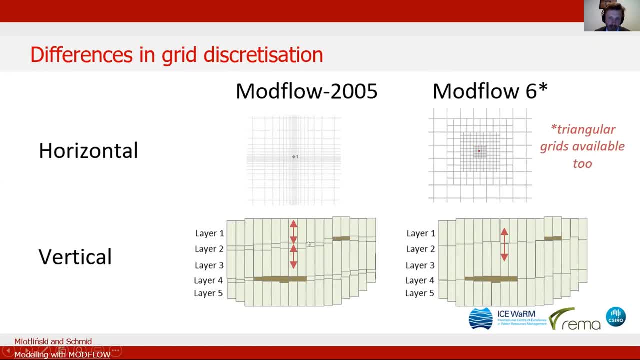 Well, this layer may have properties of the surrounding layers. So from a conceptual point of view, this is the same aquifer, but it generates a number of additional layers, And in Modflow 2006, this is basically excluded. This cell that is. 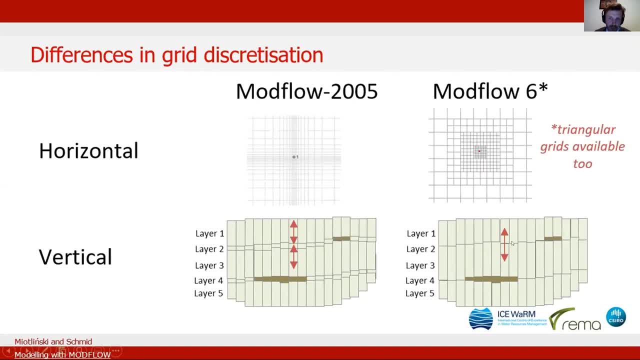 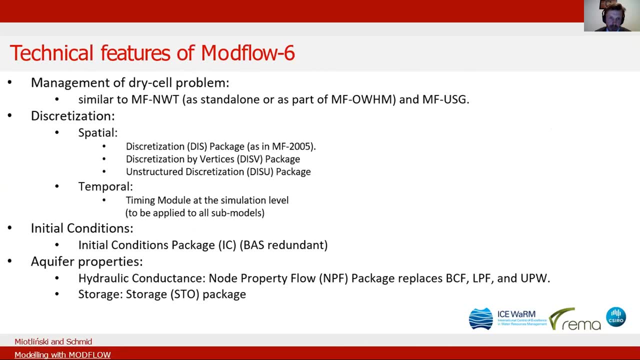 That pinch out is excluded from the computational process, So it saves basically time. There are There is a number of technical features related with Modflow 06, mostly management of dry cell problem, Or This is important, but it has been already implemented before in Modflow NWT. 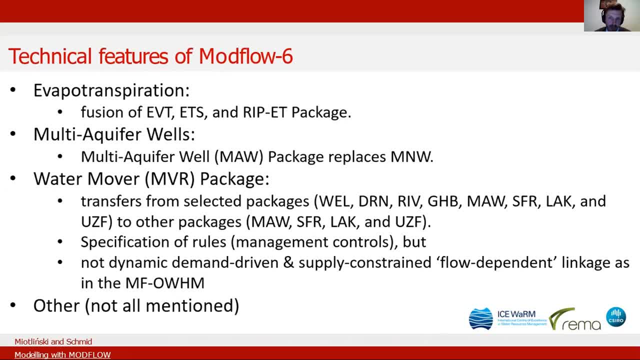 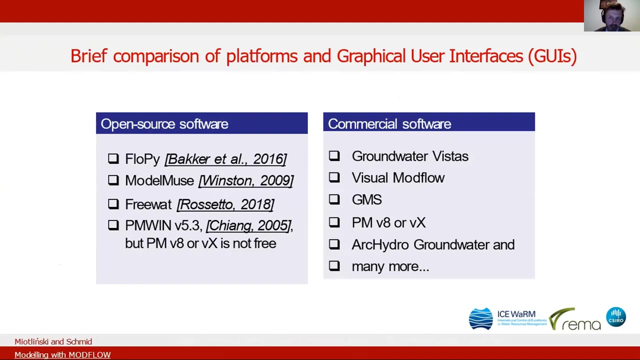 I forgot to mention. I will probably not be talking too much about the packages. They have been. They are different here. Some of them work in a similar way, but some of them are completely new. And now I would like to mention only about the graphical user interfaces. 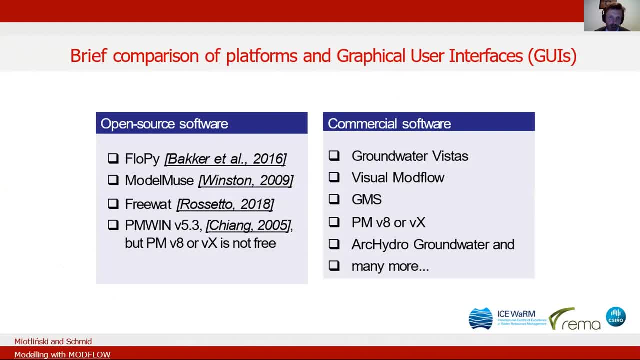 I mentioned before that there are There is open source software available, So this is free of charge. You can download this software anytime and use it. FlowPy is very popular at the moment. It's very powerful And And it basically 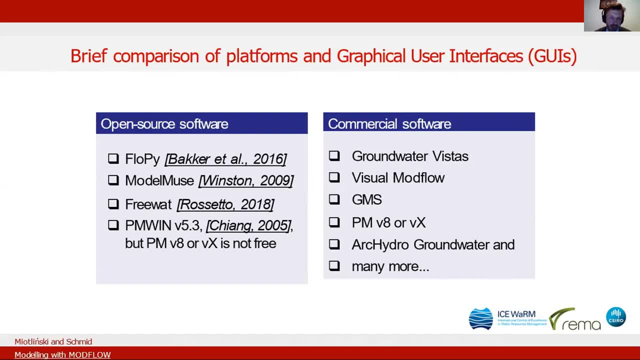 It's interfaced with Python, So if you have a little bit of programming experience, you would be definitely interested in FlowPy, And I would actually say that everyone who is planning to do modeling on a regular basis should definitely look at this, because it's a very powerful tool. 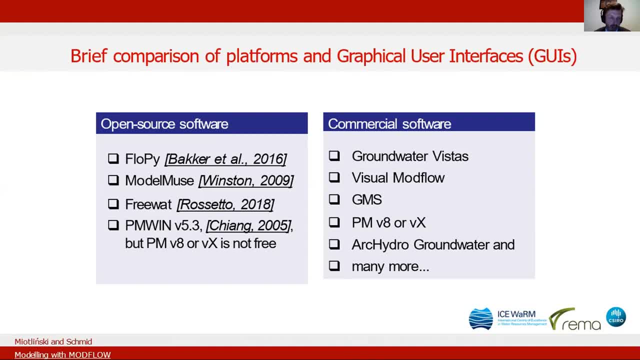 ModelMuse is another option that is available and can be downloaded from the USGS website. There is FreeWatt. that is actually a graphical user interface. It uses FlowPy too. And there is There is PMWin. Actually, I personally started. 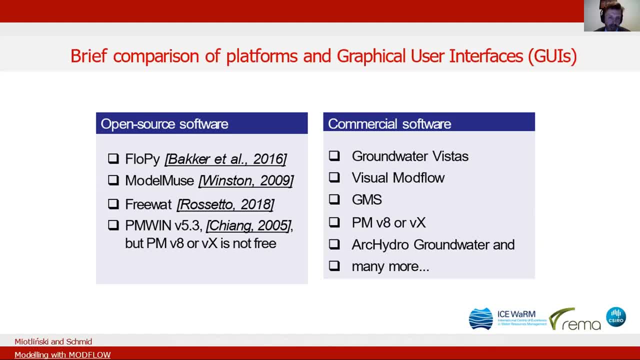 When I started modeling, I used PMWin. At this moment, I would probably not recommend this because there is a number of new versions of Modflow and packages and this will not be. The use of PMWin will not be very beneficial, And there is a number of commercial software, just to mention a few of them. 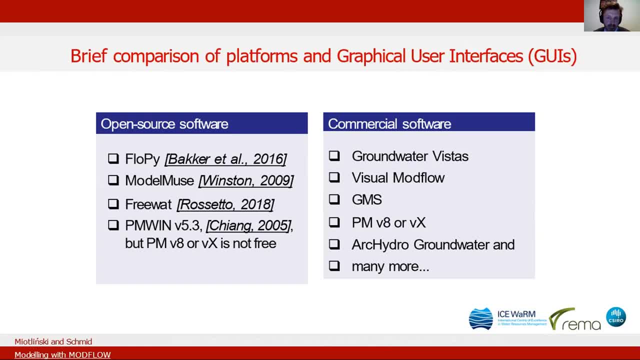 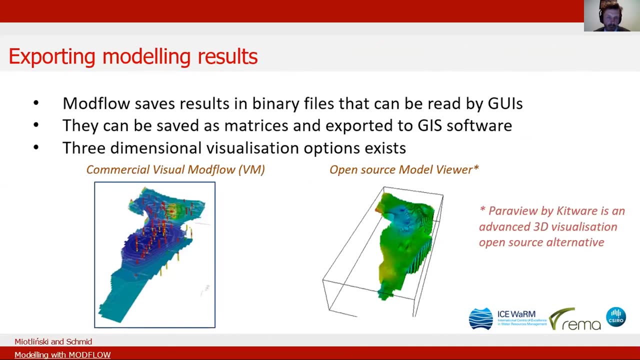 It's Ground to the Vistas, Ground to the Visual Modflow, GMS, No newer version of PMWin or Ike Hydro, And there is a number of more. And exporting. Well, we had a question about importing and exporting. It's another story, because once your model is done, 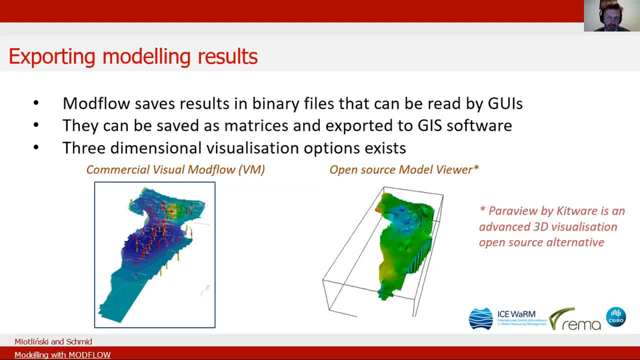 the files are normally binary. The output is in binary files and you need to read in some way. So people either use commercial software like Visual Modflow, and there is a software that USGS software that is used for input, and this is Model Viewer. 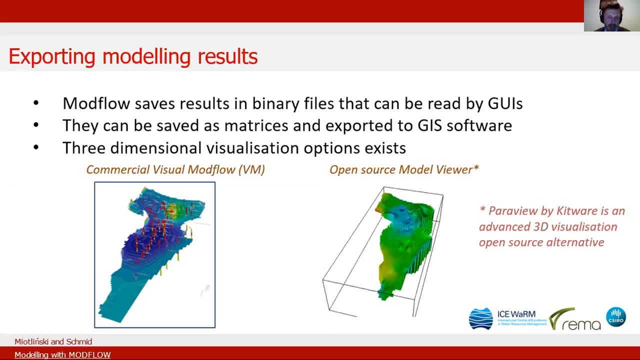 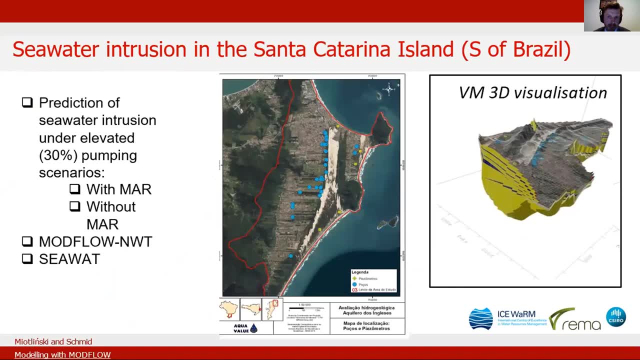 And it's actually, And this one is public domain software. And now I would like to give you very briefly talk about some. Well, one example, Give you one example from the Santa Catarina Island, where I live at the moment, where we use Modflow in order to study ground to the resources. 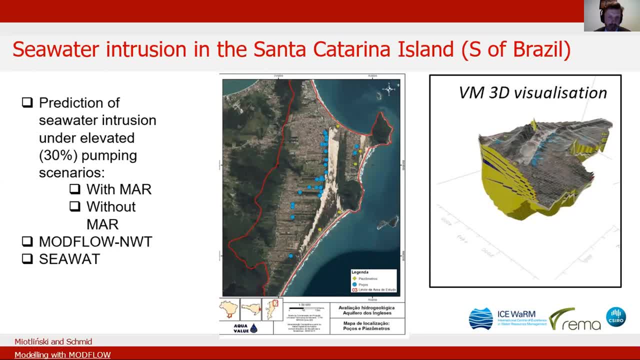 but basically the risk of seawater intrusion into the aquifer. The aquifer here. it's about 10 kilometers long and 3 kilometers wide. It's about 50 meters deep or thick And on the right-hand side you can see. 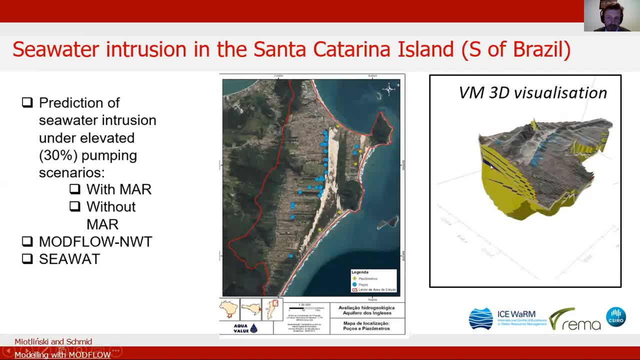 This is actually Visual Modflow visualization of this 3D visualization of this aquifer. There are some poorly permeable layers there And what we wanted to know is to see what happens if we pump 30% more than this pump nowadays. And then there was an option also to see whether some managed aquifer recharge scheme. 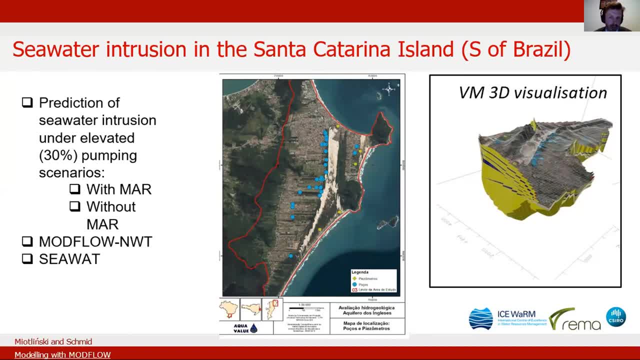 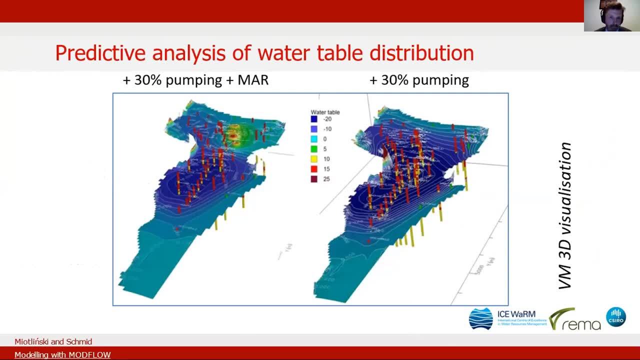 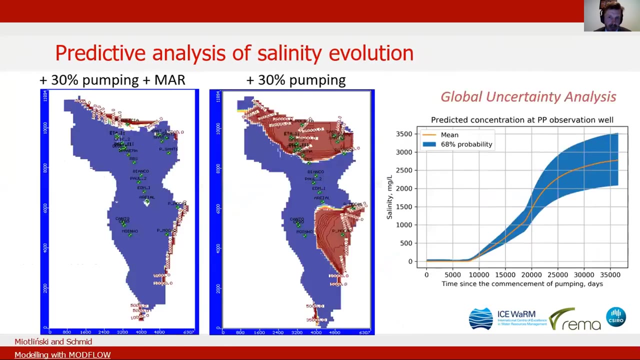 could be implemented in order to make sure that there is no seawater intrusion, And so we have done predictive modeling of the groundwater heads And you can see the water level maps also in 3D view of this under two different scenarios. And then we have done SEAWAT. 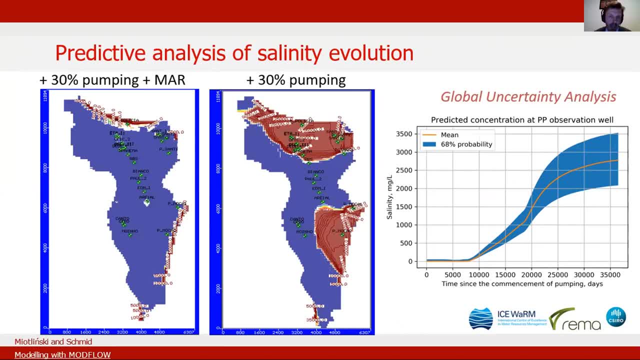 That's another software for water quality when we have density-dependent flow And we were interested how much. And we could see that if there is pumping without managed aquifer recharge, there is a very strong risk, a very big risk of saltwater intrusion. 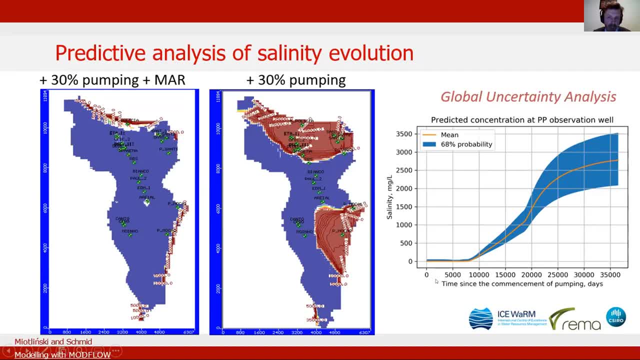 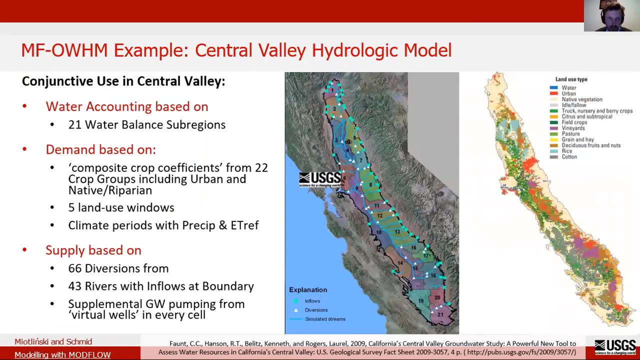 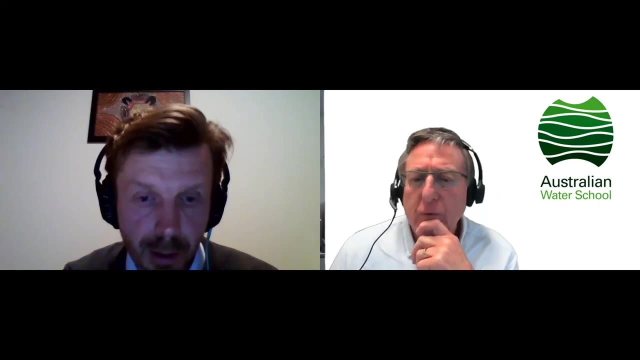 that from two sides may enter in the aquifer, And we did a little bit of sensitivity analysis here too. And now I pass again to Wolfgang to talk about his example. Thank you, Wolfgang. Are you there? Wolfgang? Yes, I am. I just need to get my presentation started again. 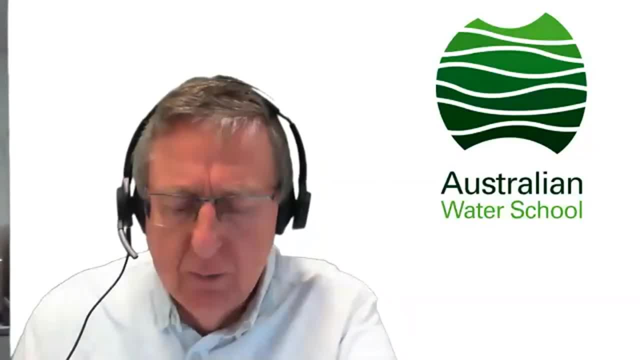 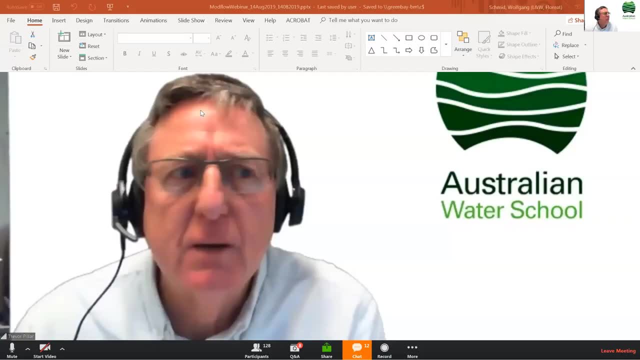 That's okay. So we are running at the one hour mark at the moment. I know we've got a little bit to go through, But if everybody's happy to hold on for a bit longer, we'll go for another 10, 15 minutes, I think. 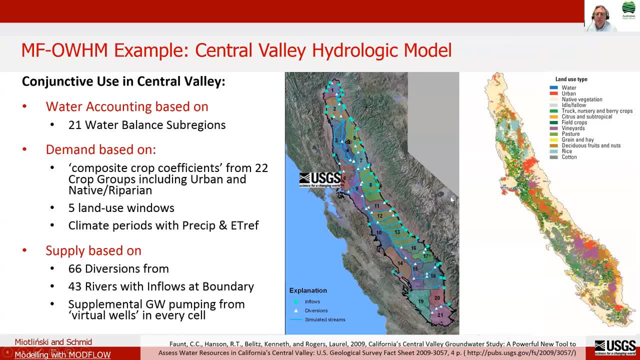 Can you see this? We've got that now. Yep, Thank you. Yep, Yeah, Okay, So how much more should we go over? I'm suggesting we do 15 minutes more. People are hanging on to the…. All right, I'll just breeze through all of this a bit quicker. 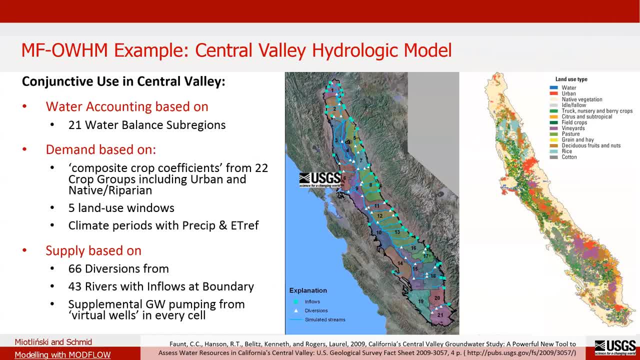 Thank you. So, in terms of macro home examples, most examples of macro home are located in the US Southwest and one recently in South Africa and another one in Mexico. So it is being used more and more. But I only can talk here about the poster boy of those mugs. 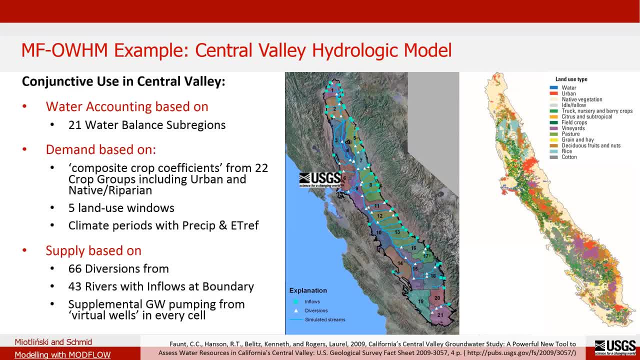 which is the first one that I was involved in, And that is in the Central Valley. So in the Central Valley, if you remember, what we wanted to do is to… Hang on, I can't see you guys. Just a minute. 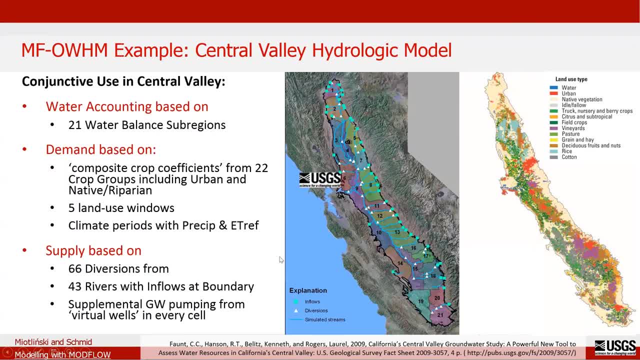 How do I do this? Just… Anyway, So in the Central Valley we do these demand-based calculations, like in a bank account for different water accounting units. So not only do we calculate demand for climate and crop coefficients that are basically obviously land use dependent. 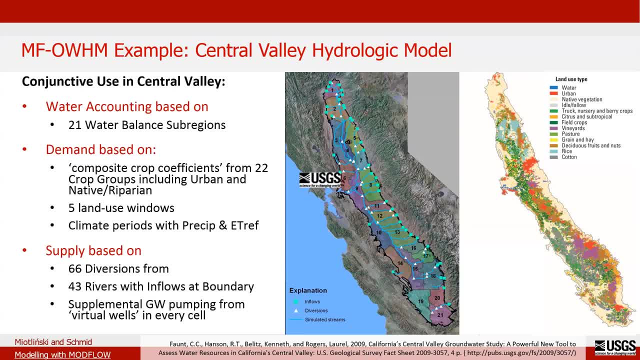 but we are doing this for a particular area. That's why it used to be called farm process, because it is for a family farm or for a farm. But a water accounting unit in this case can be anything. It can be a political entity or it can be an irrigation district. 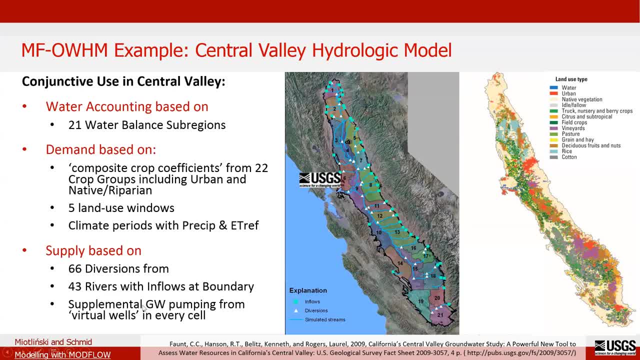 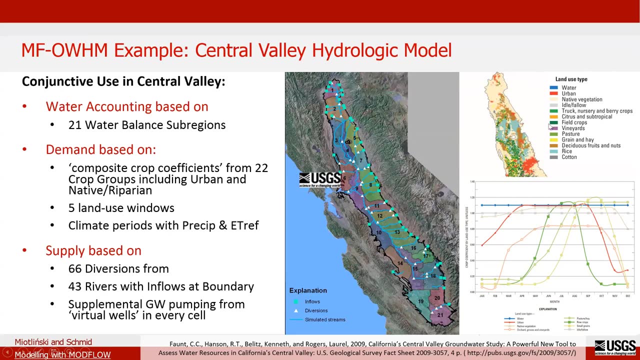 And then you've got supplies from rivers and from groundwater pumping, And what we do in this case, because the land use is so diverse, is that you are lumping certain crops together into, say, for example, field crops. So what you do is you're driving the demand. 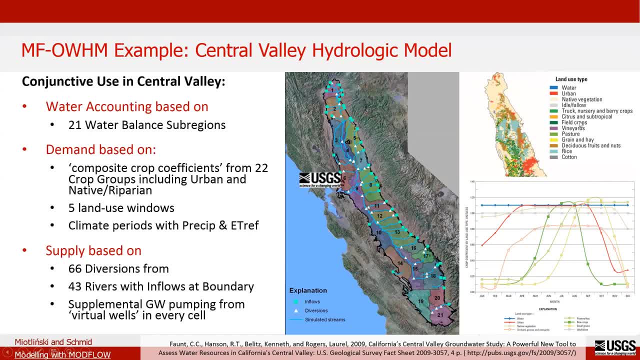 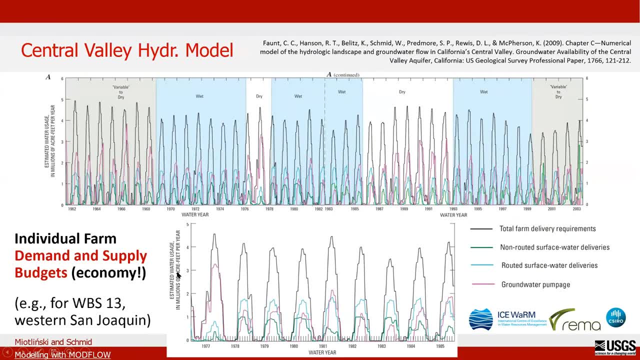 of this particular crop, not with a crop coefficient, but with a composite crop coefficient, And then the outcome is obviously this demand and supply budgets that I mentioned before. So these are time series of demand and supply across the whole historic period of this model. 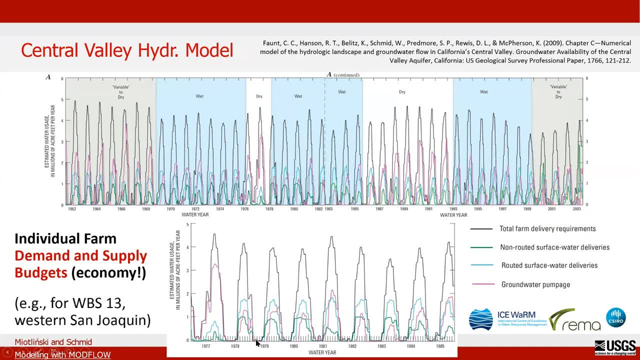 And a zoom up here for a particular time period shows you that you have in black the demands, the total delivery requirement, And then in blue you have crowded deliveries And with some time lag then you have the groundwater pumping kicking in. So this is done here for an individual farm. 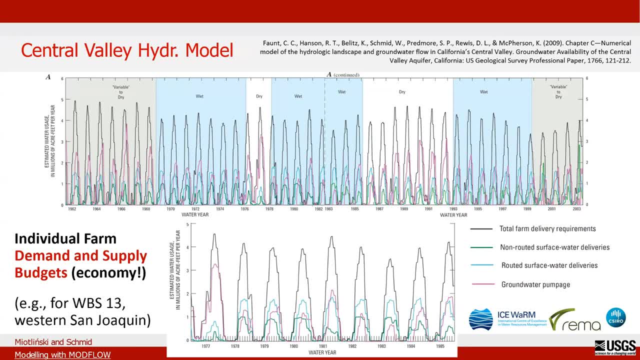 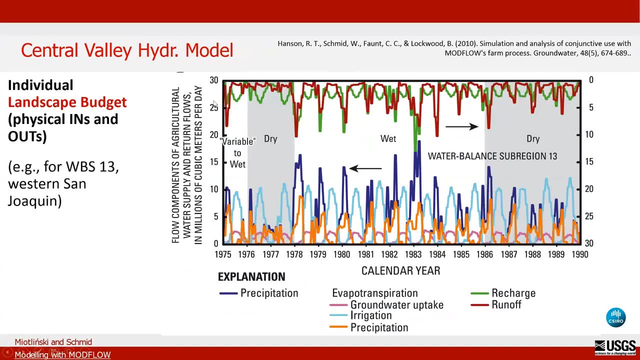 or water accounting unit or water balance upgrade. So you can see that this is the same water balance operation as it's called in the Central Valley. But then you also have physical inflows and outflows, So this is the same water balance operation. 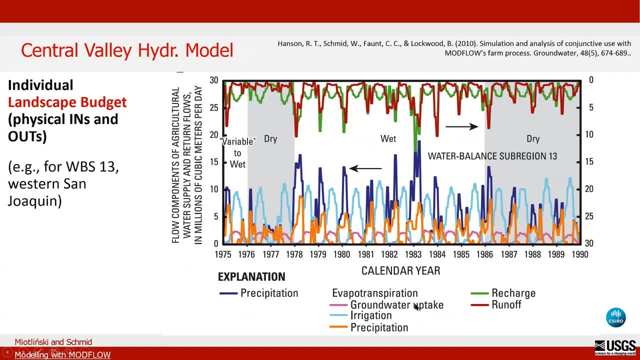 So you can see, you have components, physical inflows into the landscape, such as evapotranspiration, groundwater uptake or portions of evapotranspiration that are satisfied by irrigation and precipitation, But then you have outflows such as recharge and runoff. 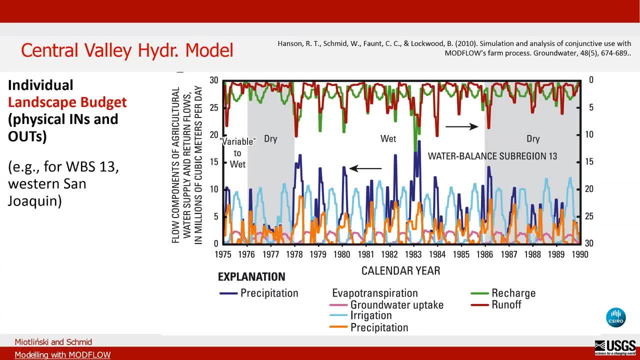 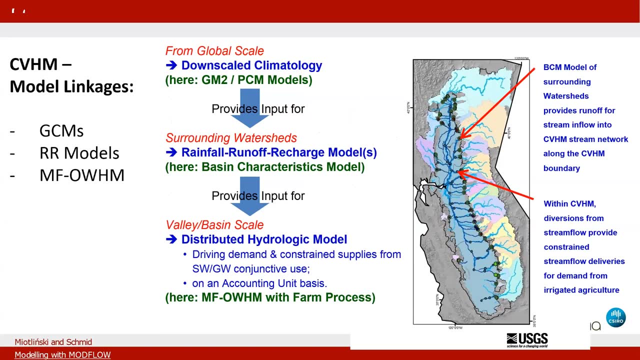 So this is just the details, but just the point that you have individual demand and supply budgets for water accounting units and you also have individual landscape budgets. Now, what we do with the entire model, once it's calibrated, is we're driving it into the future. 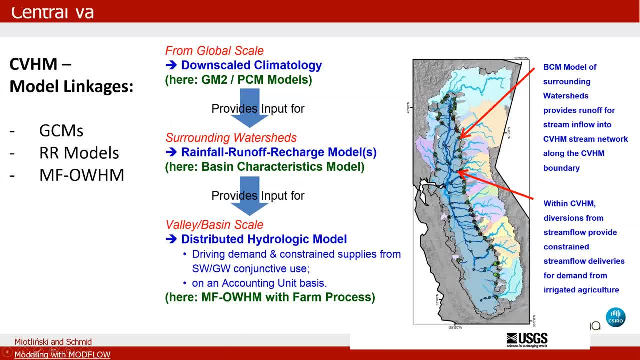 So the beauty of this is that, because it is demand-based and the demand is based on climate and crop parameters, the inflows at the streams, at the boundary, and the climate can be pre-processed by downscaled global climate change models. So the way that works is: you've got a GCM. 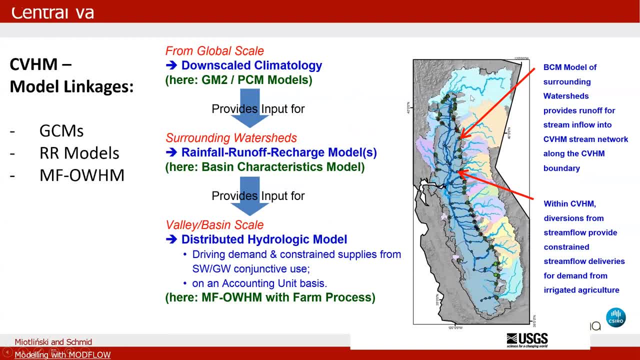 you downscale it, you populate rainfall, runoff models that are surrounding the MADFLOW model and then you basically drive the inflows into the rivers and the climate from the downscaled climate models with reference ET and then you basically can run your MADFLOW-owned model. 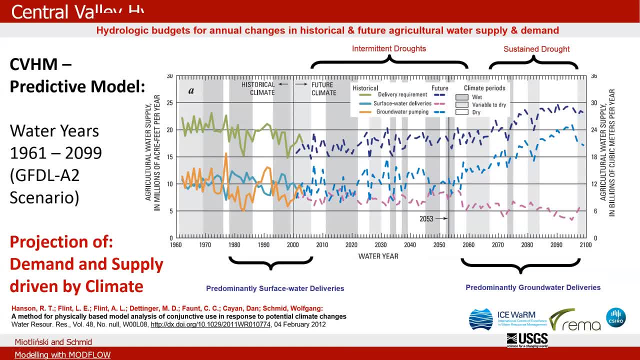 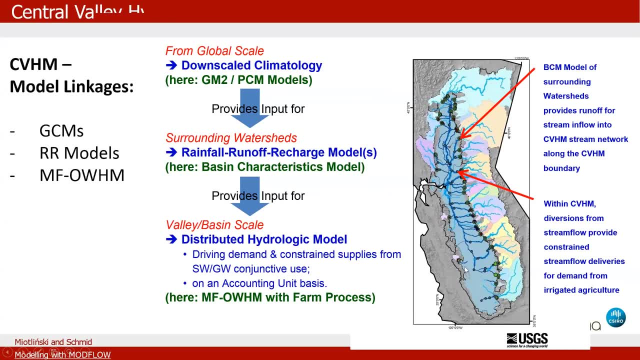 into the future. And remember that this kind of coupling is only possible if you have an automatic link between demand and supply and the demand is basically driven by climate. Otherwise, in standard MADFLOW this kind of coupling wouldn't be possible. So now here is you, remember? 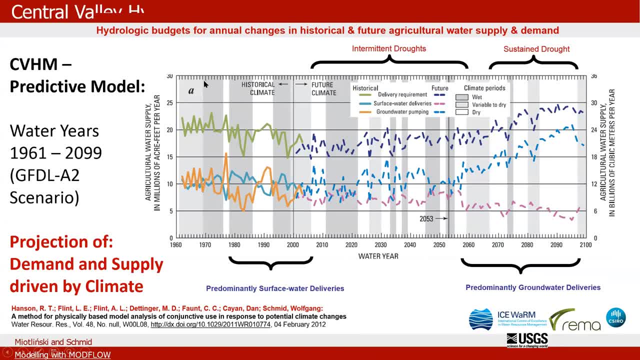 I told you about these individual budgets, economic budgets and physical budgets. This is now tallied up for the entire Central Valley, So this is the demand and supply for the whole model. That's historic. So in blue you have surface water deliveries. 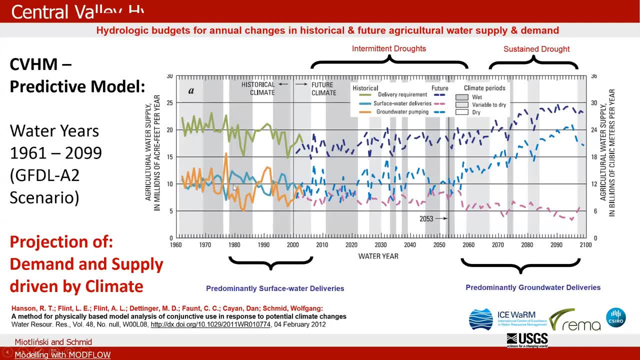 that are basically satisfying the demand. and then you have groundwater deliveries. So you see, in the 80s there was a bit of a relief and the surface water deliveries- here they made up for a lot of the demand. so actually the rock rivers were able to recover. 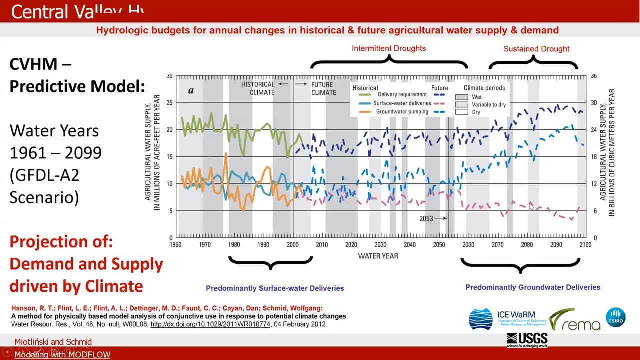 and groundwater pumpage was down. But with the GCM, the predictions, with wet and dry periods and obviously the dry periods getting longer and longer, the future looks pretty dire, judging from this model. So you get an extensive increase in demand and following that obviously 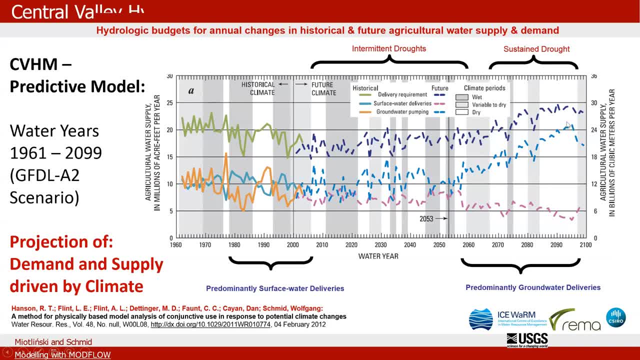 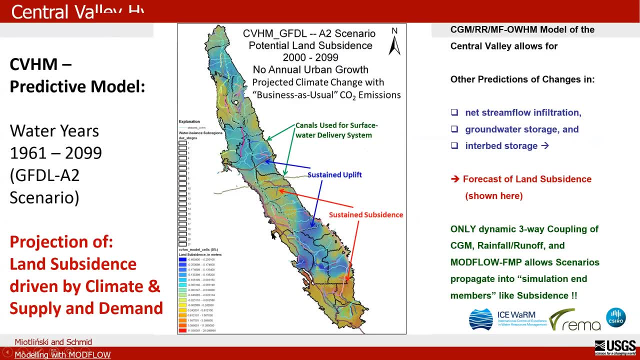 a quite increasing increase in surface water deliveries and also groundwater pumping. So now the last slide I want to show for this example is that once you have this dynamic linkage between climate demand and supply in MAFLO, you can also drive with those parameters. 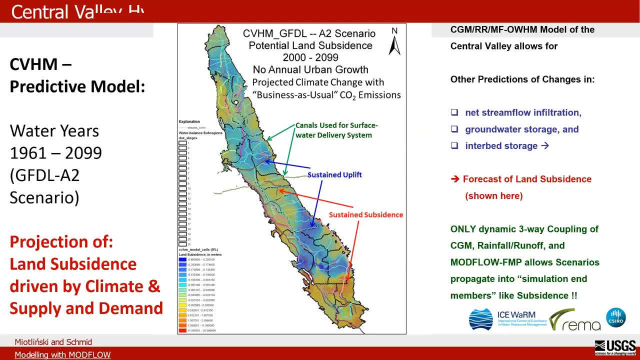 other simulation parameters, such as land subsidence. So, in other words, land subsidence in this case is also calculated into the future, driven by climate and supply and demand. And this is just what you can see with a normal business as usual scenario. 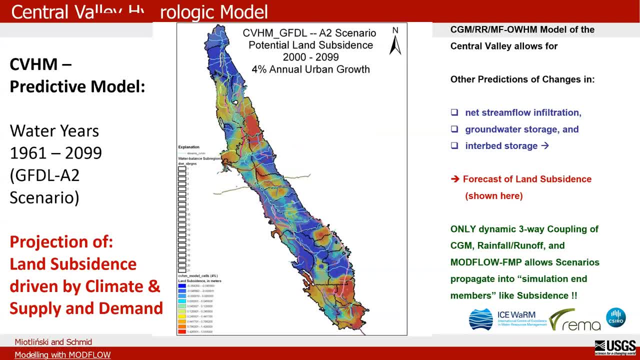 and this is basically with a 4% annual growth. So this is the Central Valley model and if you're interested in that, you can just Google for it and download it, And the lead author of this is Claudia Horn, so please contact her if you have any questions. 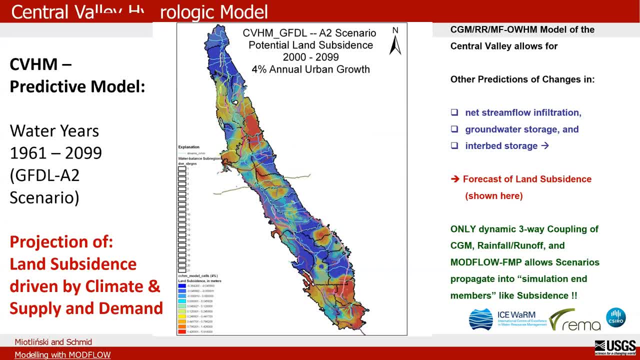 And also, of course, this model that I'm showing you. I think the historic period ended in 2006, and the application date was 2009,. so there are newer versions that are in process at the moment, which should be published shortly. 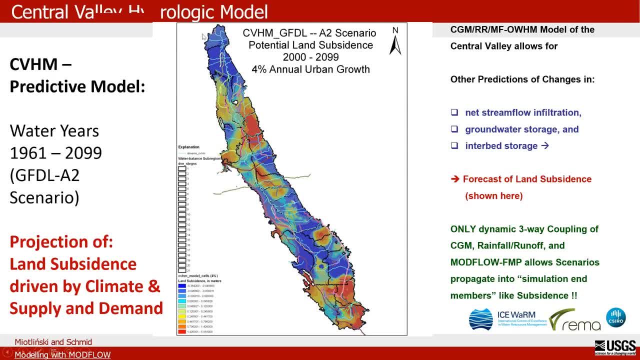 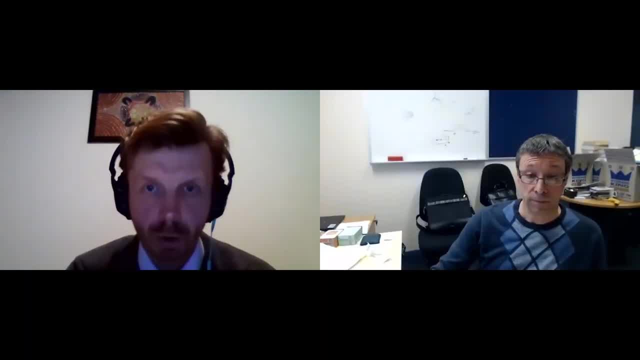 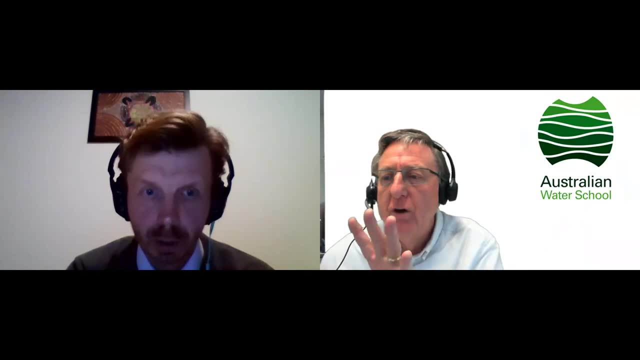 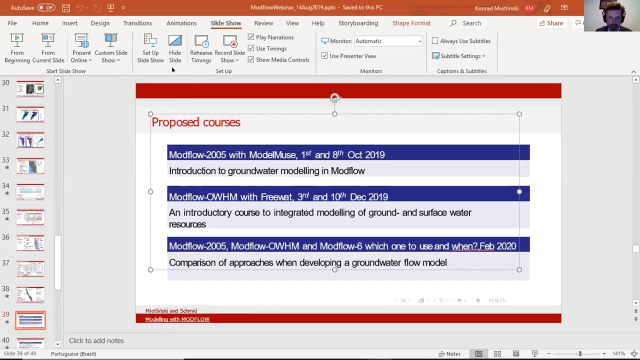 So back over to you, Conrad now. Yes, thank you, We've got about six minutes. we kind of read that five minutes ago, Yep, yep. So basically, now we would like to suggest some courses. This is something that we still have to. 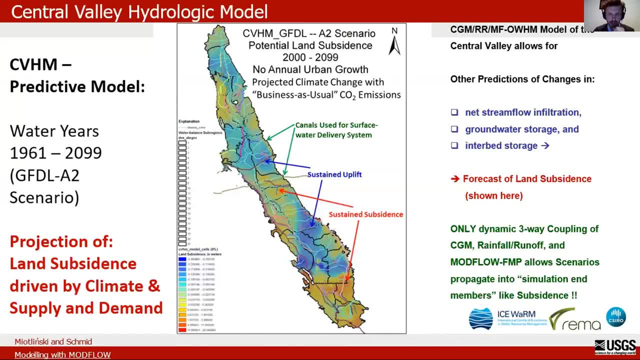 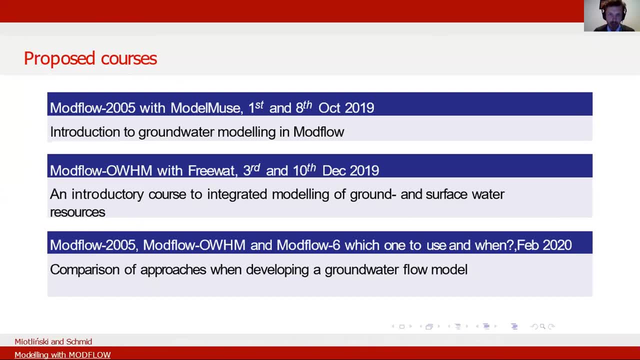 well, the first course is will be in October 2019, in the beginning of October, and this would be introduction to groundwater modeling with Modflow, And at this point we suggest to use Modflow 2005 together with Model Muse. 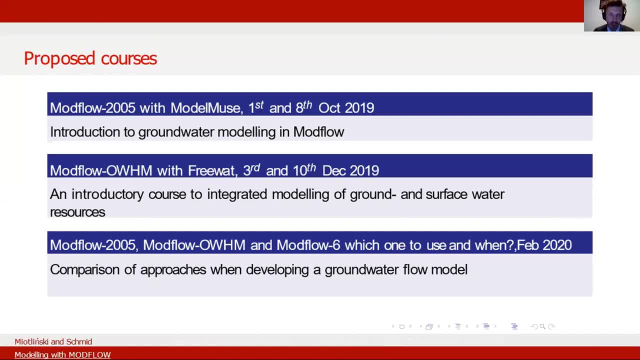 which is open source software. so if you want to, you basically don't. if you want to continue and develop some models with it, you don't need to invest any money into the software. everything is publicly available. Second will be Modflow OM with FreeWatt. 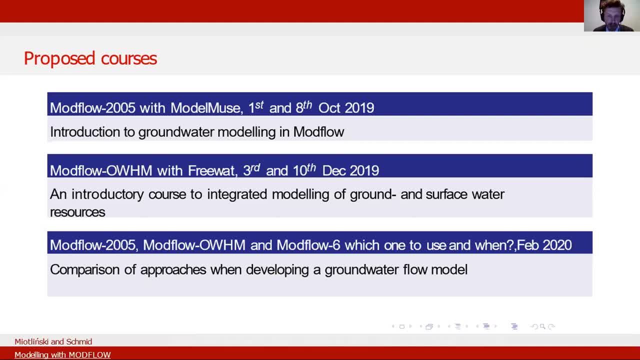 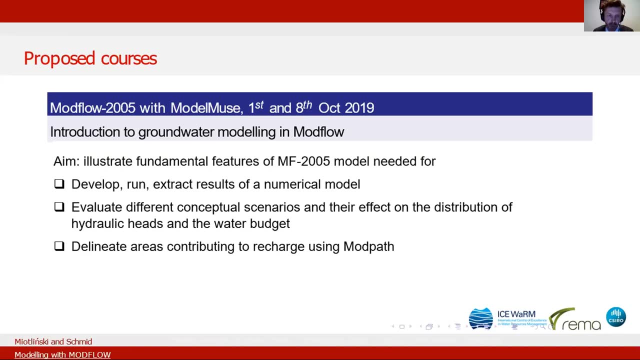 and third will be some kind of comparison of approaches when developing a groundwater model. So we'll be talking about Modflow 2005,, Modflow OM and Modflow 6.. So the first course will be very basic, as I mentioned, basically how to import data. 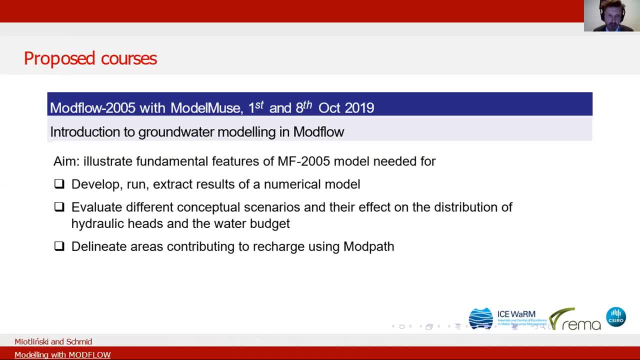 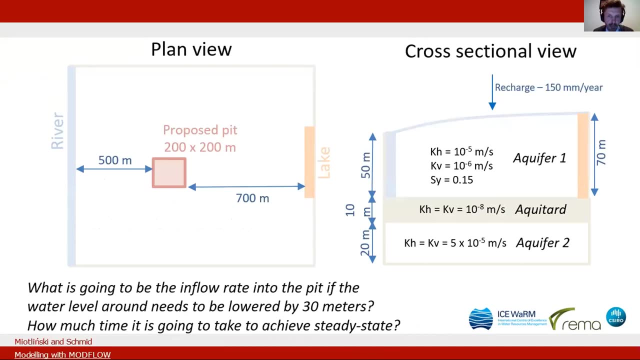 develop model, run and extract results and evaluate some different conceptual scenarios and maybe delineate areas contributing to recharge. This is some kind of conceptual model and some kind of actual problem we may be working on, and this will be very basic level If you are starting modeling. 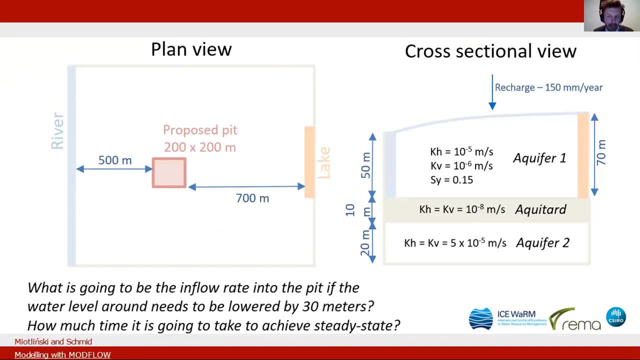 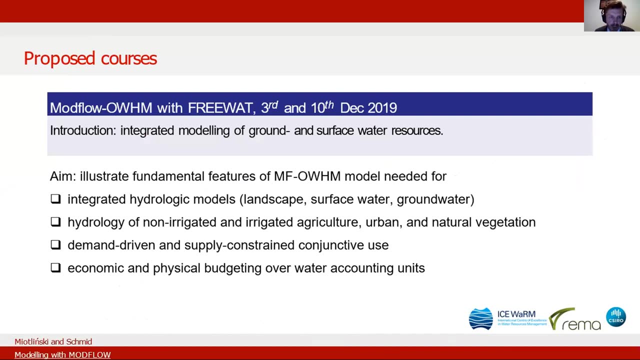 if you are, or you had a break and you want to refresh your knowledge about Modflow 2005,, this will be a good course for you. Then we have Wolfgang's course. Wolfgang, would you like to say something and probably go to the end with this. 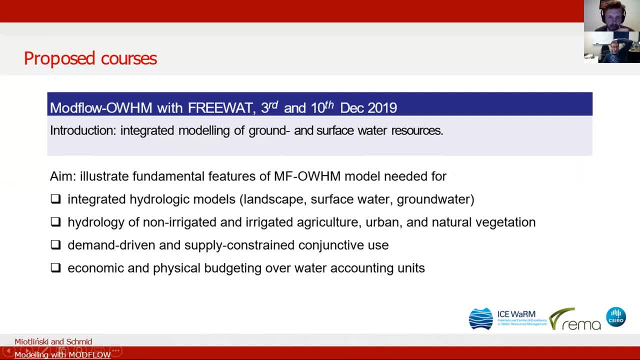 Yes, yes, but we'll use your presentation. so if you just Yeah, yeah, yeah, sure. So this class, basically, will just show you the few highlights of Modflow OM embedded in QGIS, which is the freeware GIS platform in FreeWatt. 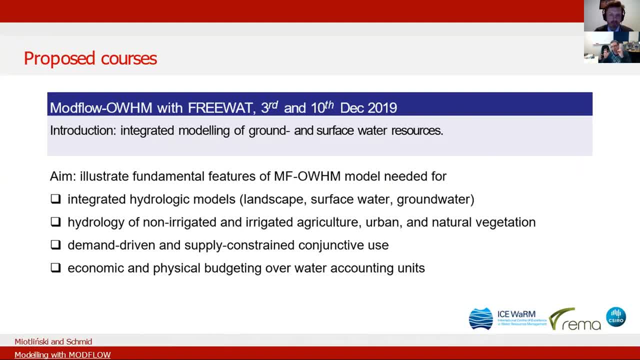 So it's all free, it's Modflow, OM and it's FreeWatt and it's QGIS, and we'll show you how to develop a very, very simple model, integrated hydrologic model, where we calculate precisely the budgets that you also saw on a larger scale for the Central Valley. 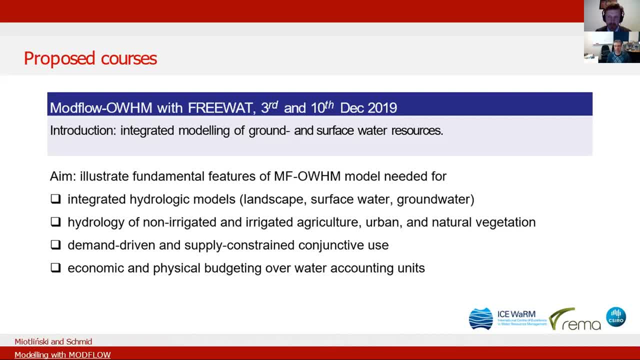 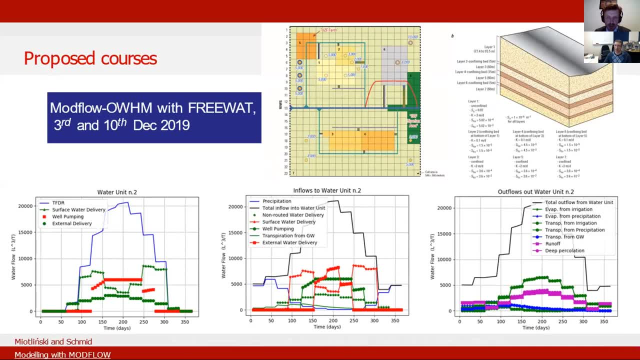 If you can go to the next slide, Conrad, Yep. So this is basically where you can see the layout. This is the standard time process example that we have had since probably almost now 15 years. One of the things to mention is: it would be really good. 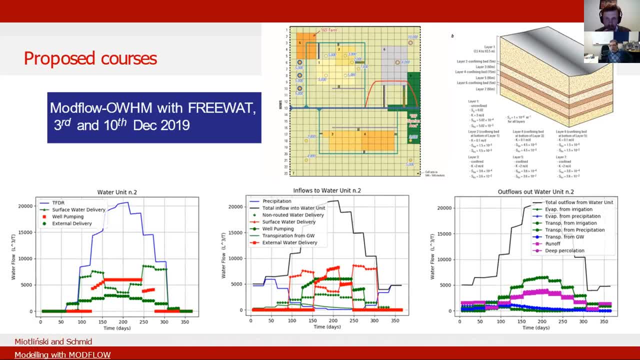 if participants for this class took Conrad's class first, because you have to have a basic understanding of how to do a general Modflow 2005 model In the interest of time, because we got two different sessions, two by two hours, we may actually I don't know really. 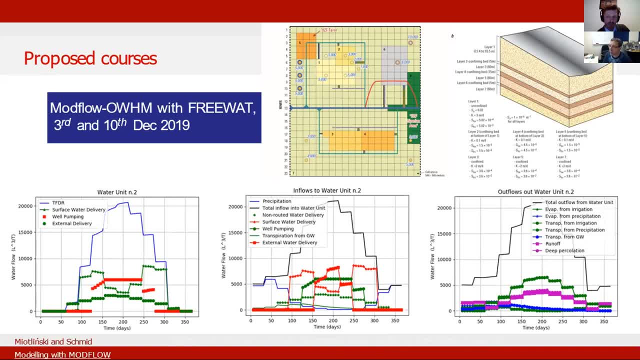 I haven't decided on this, but we may import the entire Modflow 2005 model first and then superimpose the farm process in the second session. So I have to experiment how that works. But what I will do for this class is: 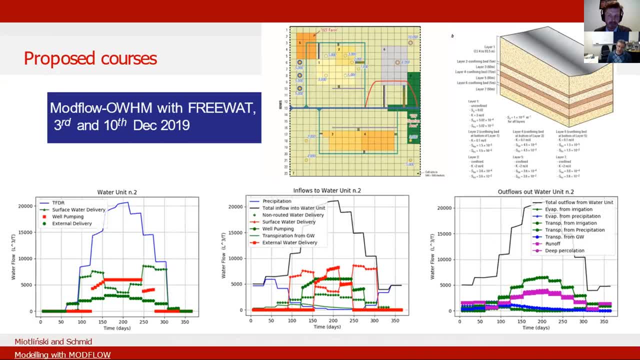 I will send you all the download instructions and make sure that you have FreeWatt properly installed, which can be quite tricky, but this needs to happen, obviously, at least a week or two before we start this class. So if you want to sign up, 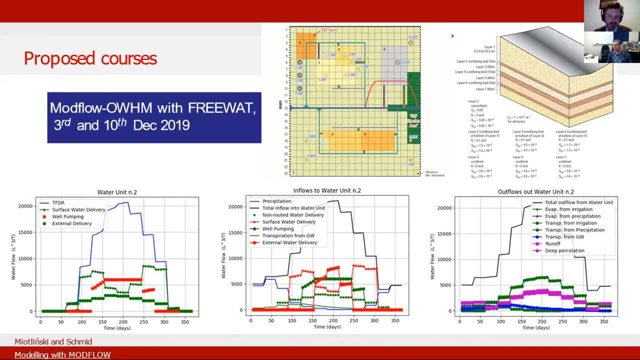 before this class: make sure you sign up early, not in the last minute, because you won't be able to install the stuff anymore, And below you see exactly what we want to do with this. So the outcome is demand and supply and inflows and outflows. 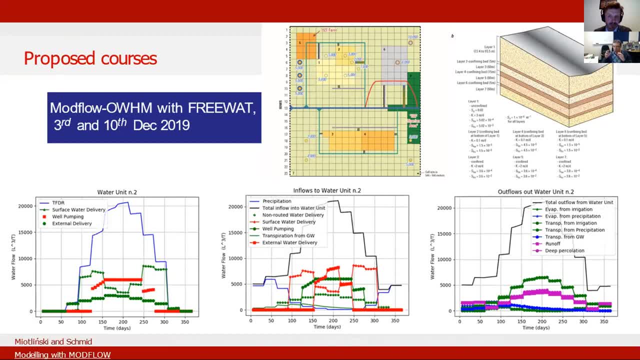 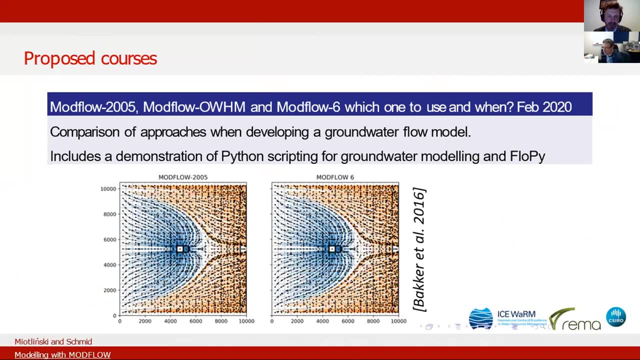 That is not a lot compared to what all the stuff that Modflow OM can do. but that's all we can do, probably in two by two hours: Conrad, Yep and the final, well, February. we would like to integrate in some way the approaches. 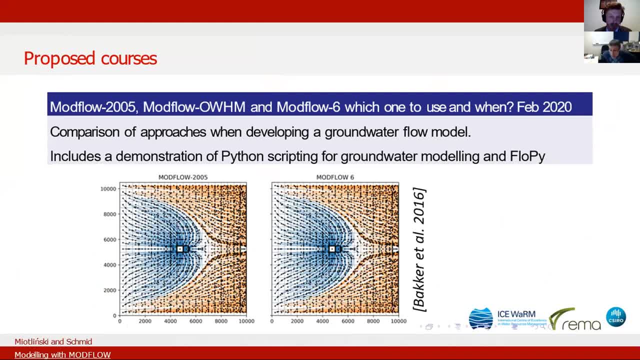 and to talk about possibly develop a model, a single model, using different kinds of tools, And we may include the demonstration also how to use FlowPy. Obviously, this is quite a complex thing, so we will not be a developing model using FlowPy probably. 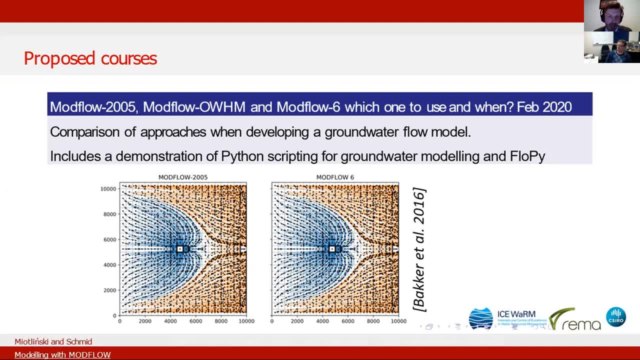 because at this stage it may be too much, But at least the demonstration and you can- later you can also play around by yourself and see what the capabilities are of FlowPy. But at this stage I can tell you that the capabilities are huge. 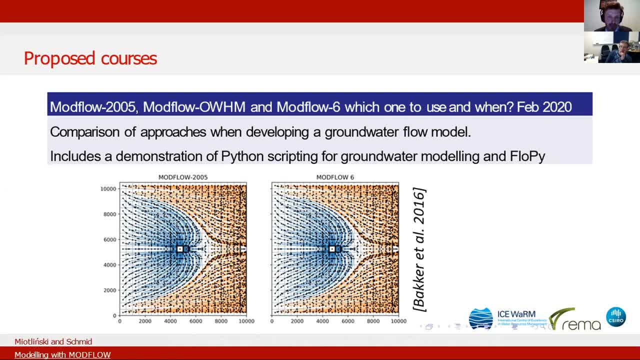 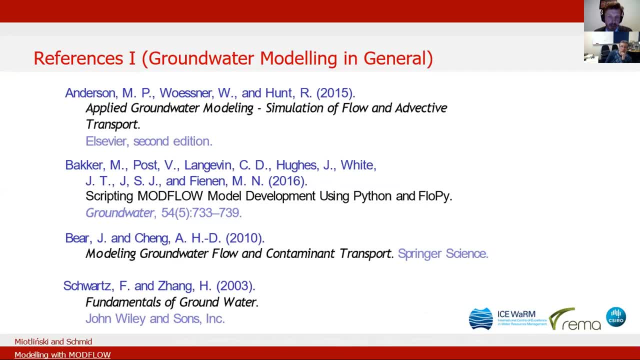 So it's definitely something that we at some stage would like to share with you guys. And then what we prepared are some references, everything what we have, well, the figures we showed and some concepts we used. Very important book is the Anderson 2015.. 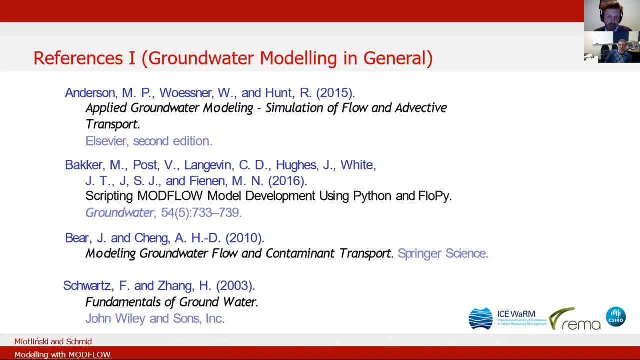 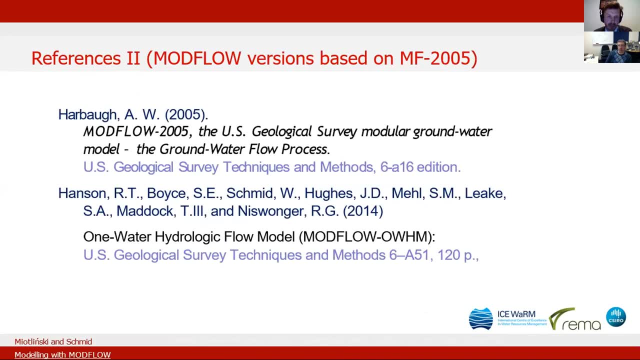 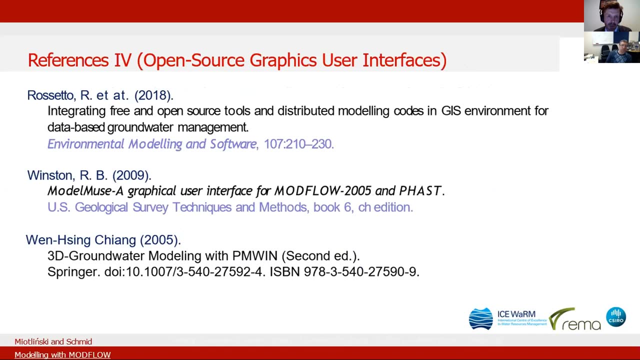 There are a few others too: Bear, obviously, 2010.. There are references for Modflow, Harbo, 2005.. And a couple of other things And open source graphic user interfaces too. Thank you very much for your attention. 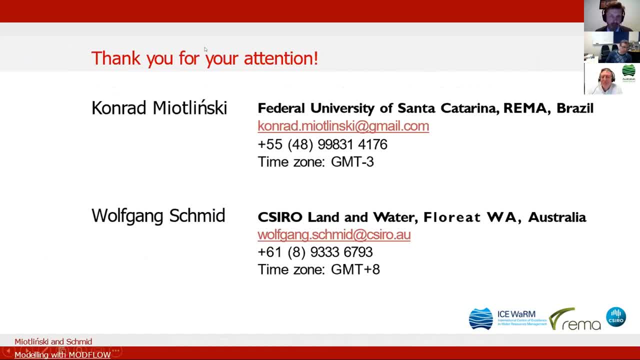 That has been a very good time. I'm still replying some of the software, some of these questions here. Trevor, Thank you. I'm replying some on the fly. I see that, But I haven't replied everything yet. No, that's been fantastic. 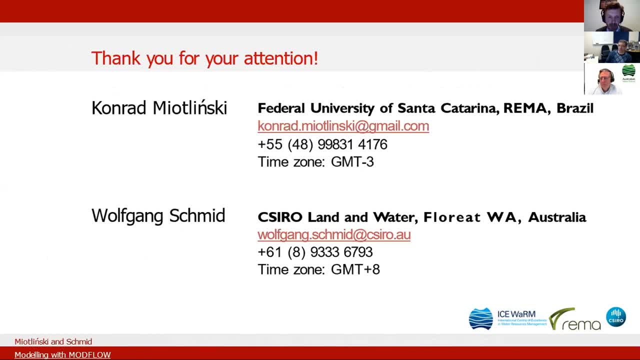 So if what will be, so shall I continue like this. Certainly We'll have a minute or two to keep going, But, Wolfgang Conrad, it's been absolutely fantastic, Your carefully step-by-step precept-on-precept approach. 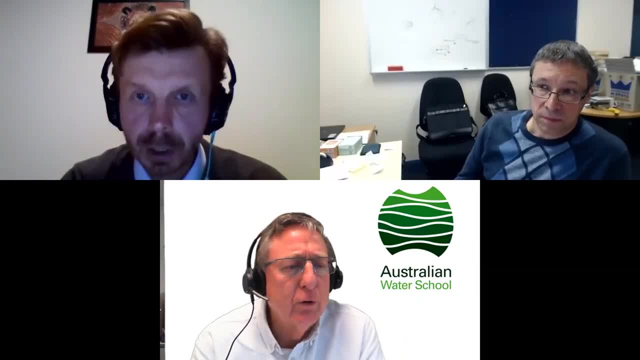 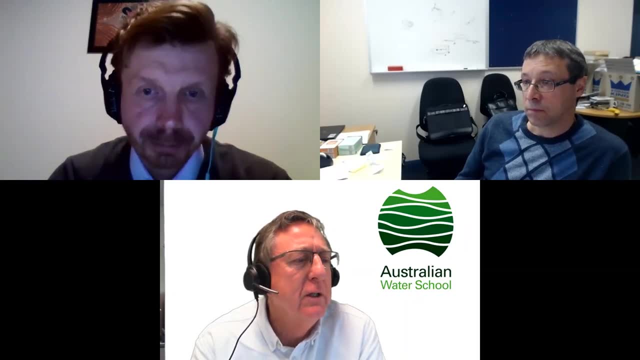 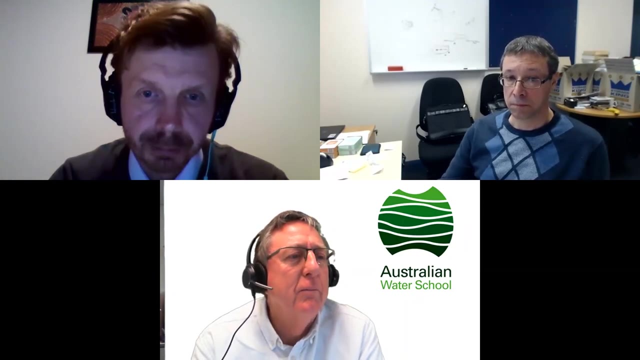 everybody really appreciates. It's been a wonderful hour and a quarter and much more to come. My colleague Christy has just put up on the chat line. you'll see the registration link. Do go to that And we'll have a fantastic time in October. 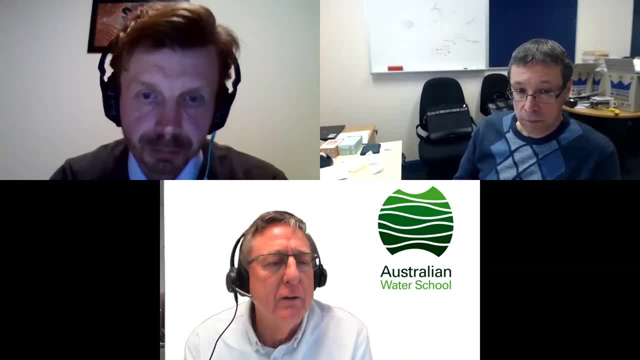 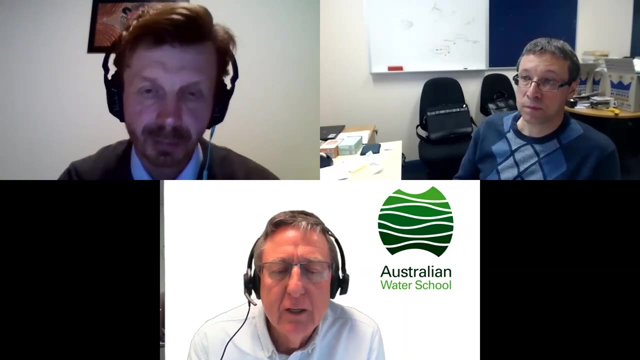 December and February to tease this all out in much more detail, But for now I just want to say how much we appreciated your attendance and, for Conrad and Wolfgang, your huge amount of effort and preparation that goes into these things. We greatly appreciate it. 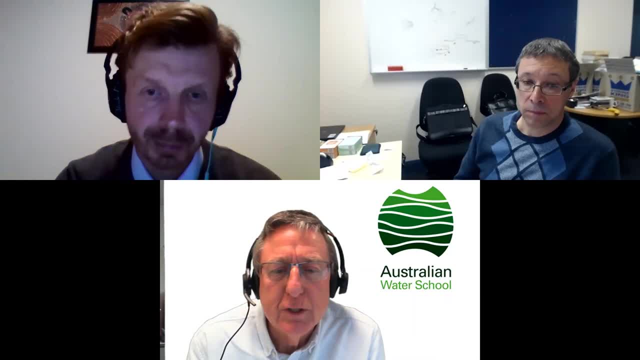 And we look forward to the three courses coming up. Each course is two sessions of two hours, So you'll be getting a full four hours from these very experienced gentlemen. All right? Well, I think we'll wrap it up there and move straight on. 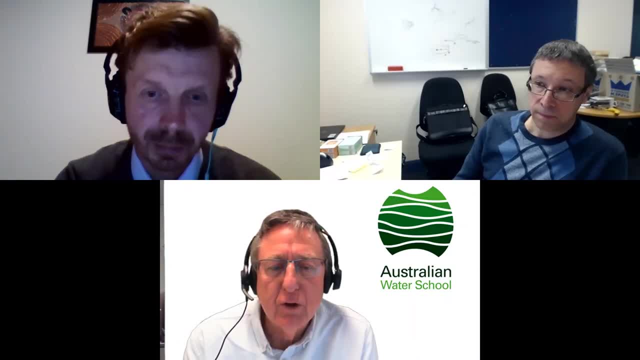 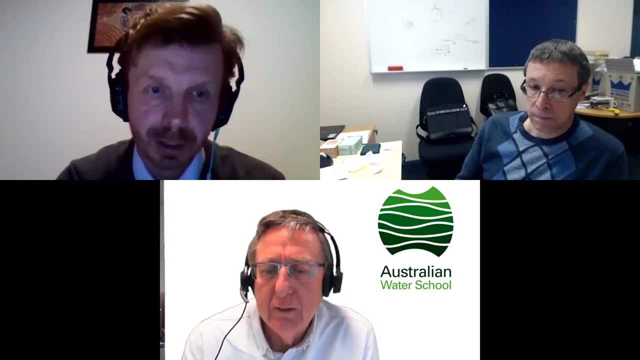 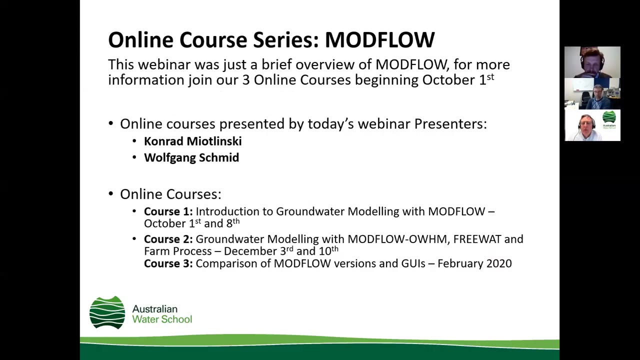 Unless there's any final comments from yourself, Conrad Wolfgang, around this whole thing, we'll go to our last slide and end the webinar here. I reckon Yep, So well, there it is. There's the dates at the bottom there. 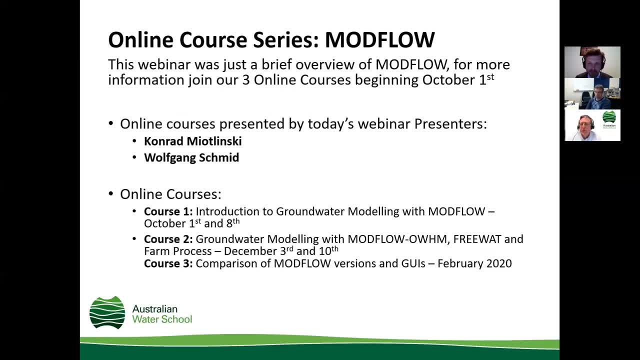 Course one, October 1st and the 8th, That's the intro. Course two with Modflow OM FreeWatt Farm Process, December 3 and 10 with Wolfgang. And the last one with both Wolfgang and Conrad. 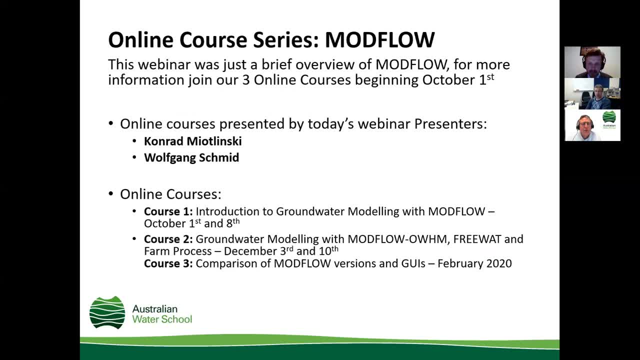 Comparison Modflow, versions and GUIs- Some of the questions. we're touching on all those three areas. So terrific, We'll wrap it up there. I have a couple of questions. Nothing more to say. Conrad, your last comment. Wolfgang, last comment. 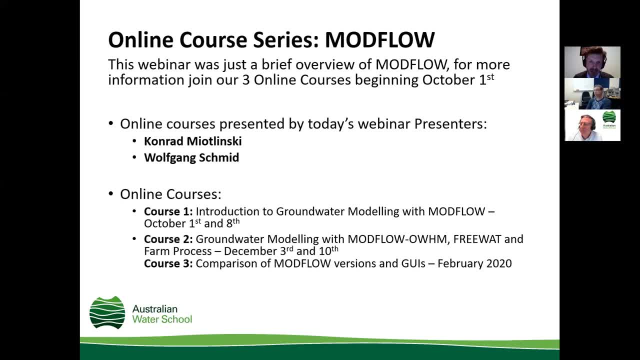 Well, thanks very much. I appreciate all participants who attended. Hopefully you'll get something useful for you. Thanks very much, Trevor for organizing this, and Wolfgang, of course, It has been great. Yeah, Thanks everybody, It's been terrific. 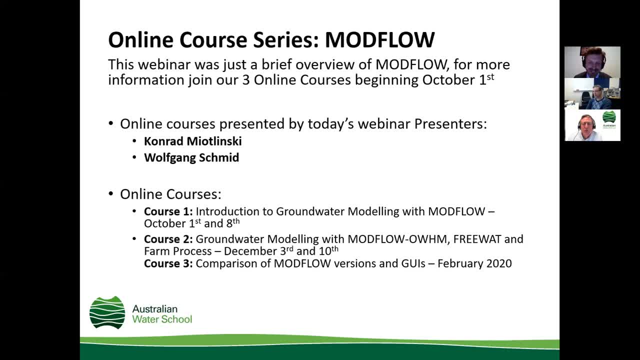 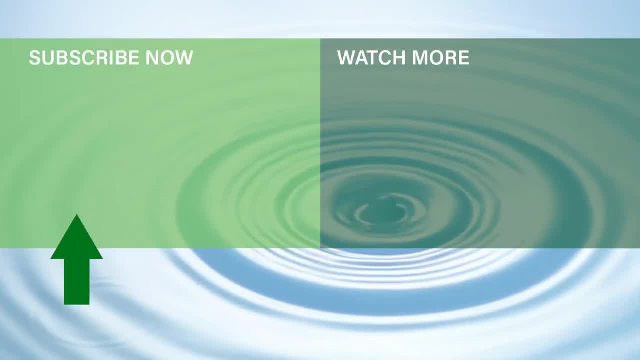 I appreciated your questions, everyone, So I look forward to seeing you at the courses, hopefully. Bye for now, Okay, Bye-bye, Bye-bye, Bye-bye, Bye-bye. Subscribe to this YouTube channel by clicking the subscription button.